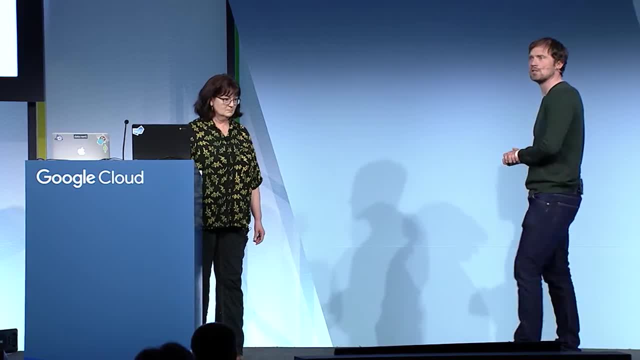 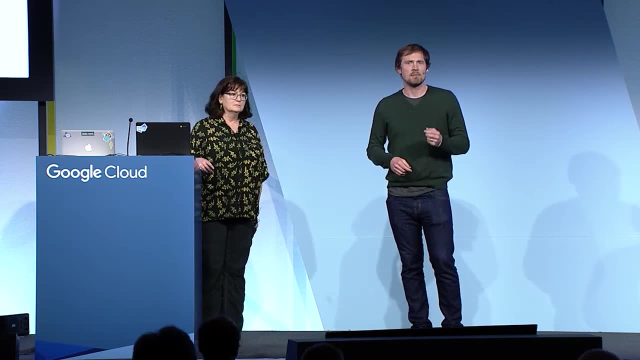 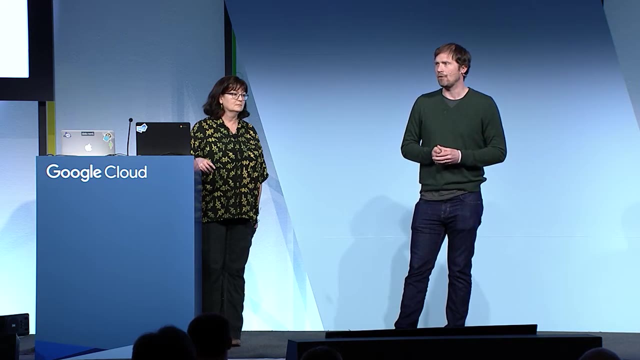 The main project I work on is Global Fishing Watch, which is the main thing we'll be talking about today. My background is in physics and earth system science and I am both fascinated by, and deeply concerned by, the human impact on the globe and very excited about the role of data in better understanding and addressing those challenges. 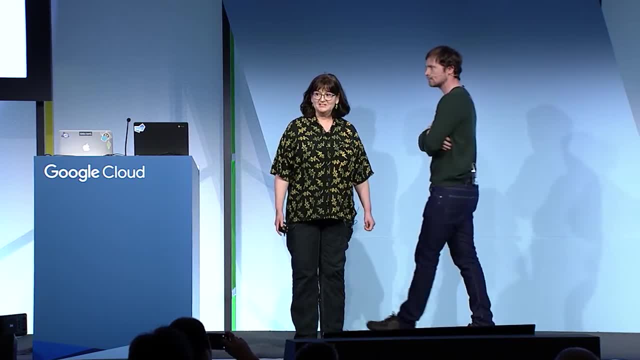 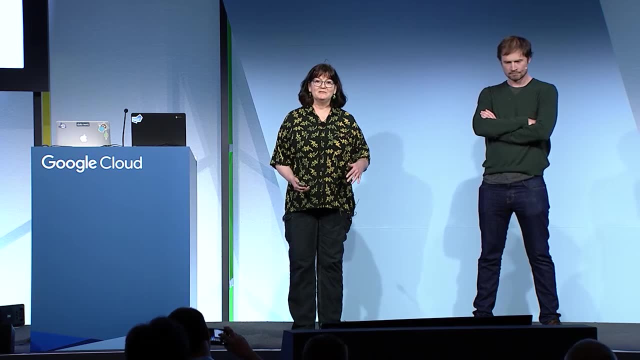 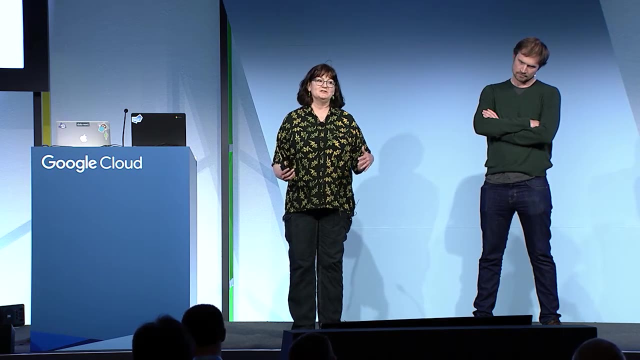 And I'm Amy Unruh. I am in developer relations on the cloud platform at Google, And so how this came about is: I originally proposed a Google Next talk that was essentially on the same topic in terms of the underlying infrastructure that Global Fishing Watch is using. 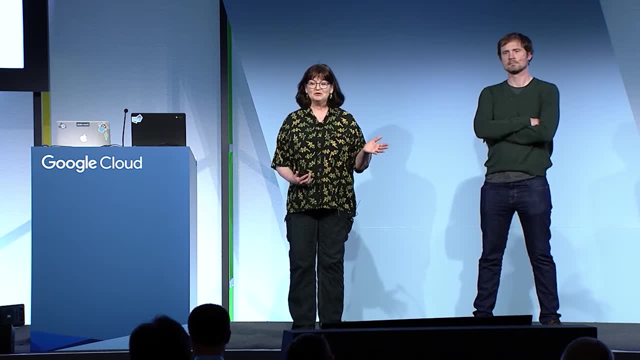 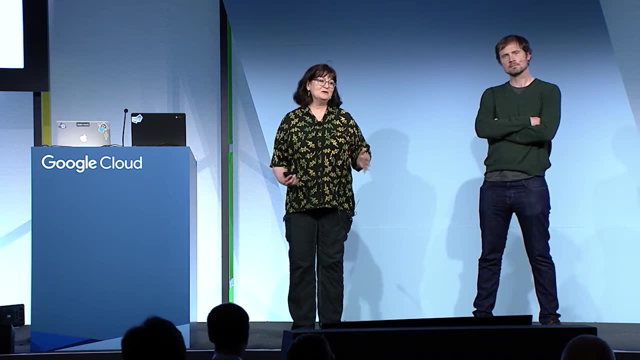 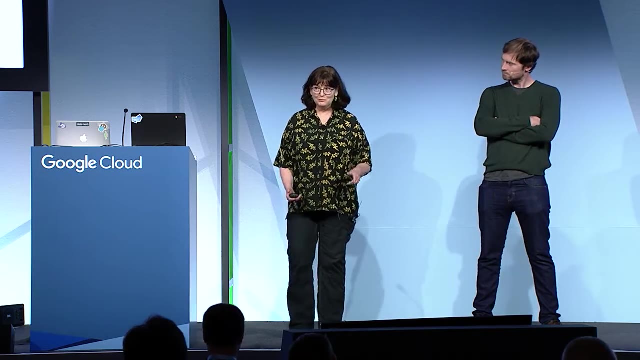 And so then I, After I proposed that I attended an internal talk where I learned about Global Fishing Watch and I was extremely enthused, And so we joined forces, and so you're going to hear about a lot of interesting- really interesting- tech solving real-world problems. 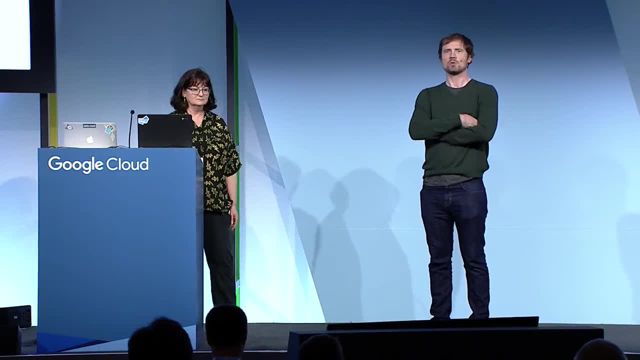 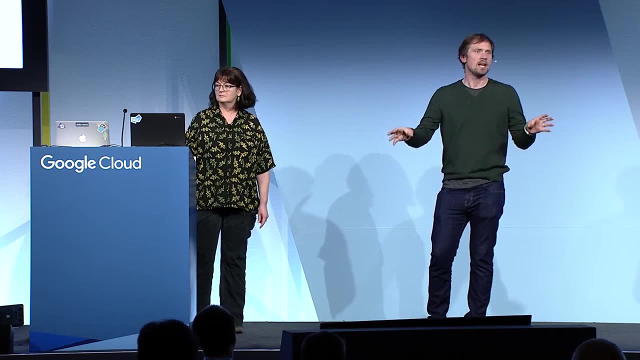 And so the first thing we're going to talk today about is Global Fishing Watch, which is this project, And we should say right away that Global Fishing Watch is a partnership between SkyTruth, where I work, Oceana a, a oceans conservation nonprofit, and Google. 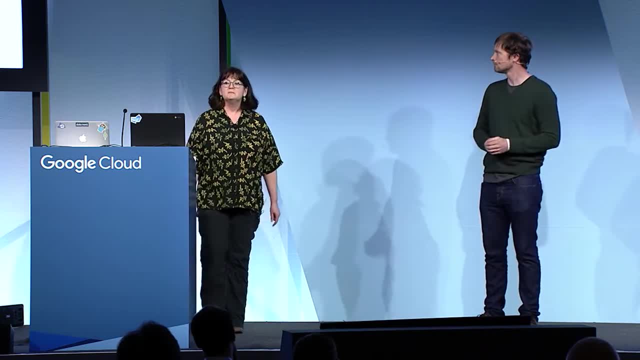 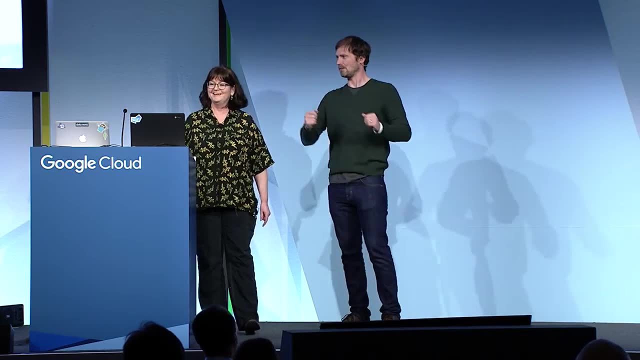 which is one reason that I'm working with Amy, But the slides don't seem to be advancing properly. by the way, We see it right here though. Yeah, we see it on our. Let me just turn the laptop around. There we go. 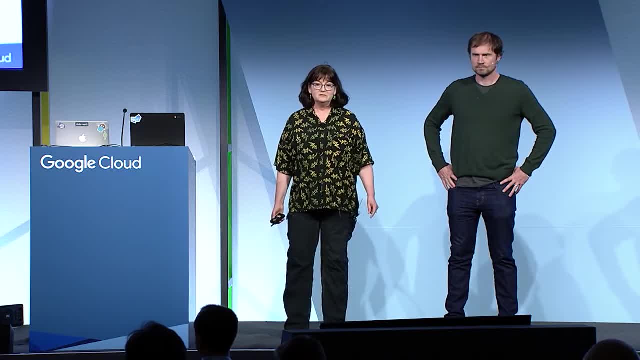 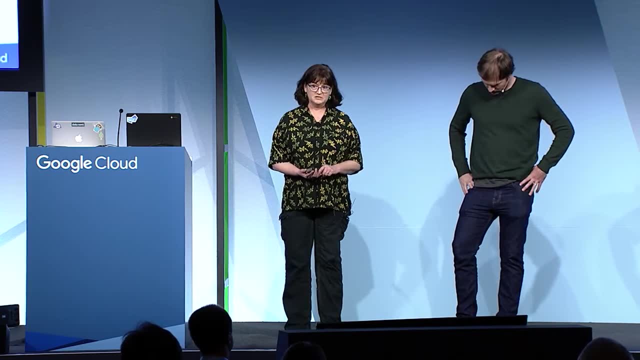 So we're going to talk about how Global Fishing Watch uses Google Cloud Platform products And, in particular for this talk, we're going to focus on Cloud Dataflow, TensorFlow, Cloud ML Engine. They also use BigQuery and GCS a lot. 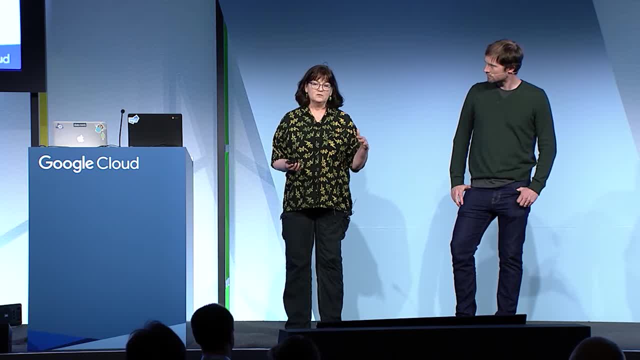 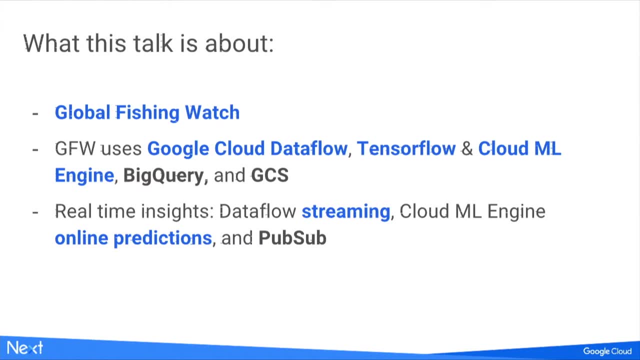 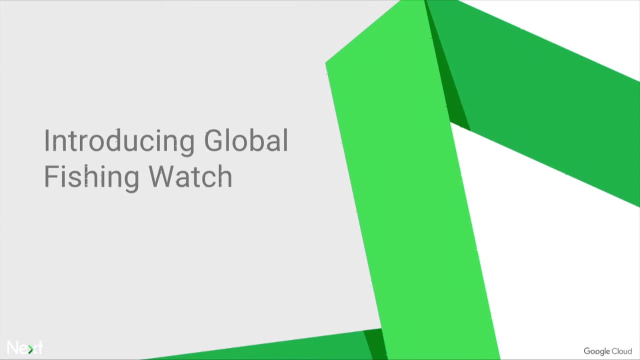 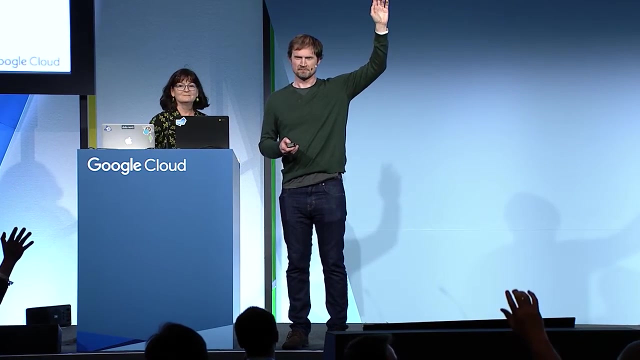 And we'll also talk about how we can take what Global Fishing Watch is using sort of as a basis for doing something new to generate close to real time insights about the things that they're tracking. OK, so Global Fishing Watch. So who here has gone fishing, as most of you. 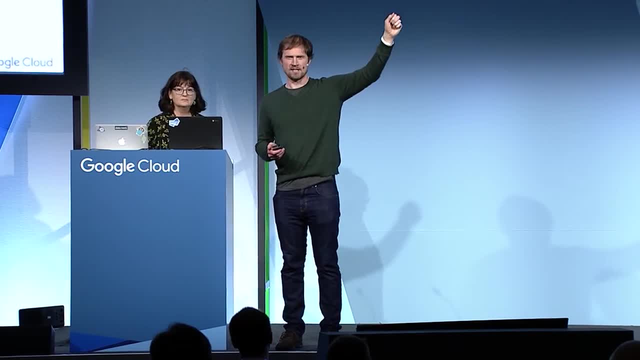 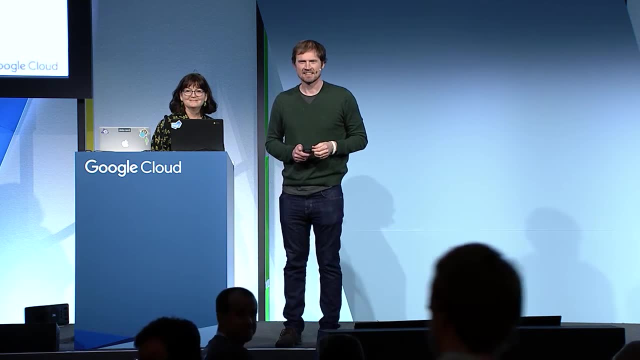 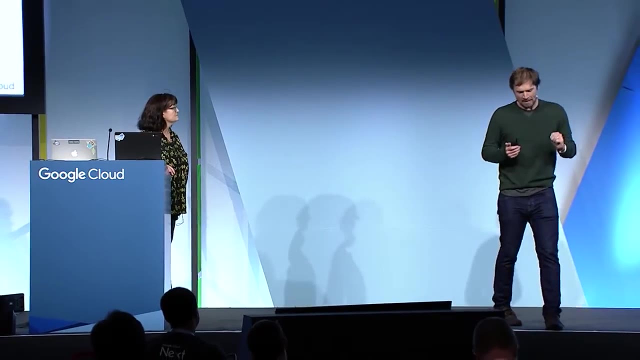 Who here has been on an industrial fishing boat at some point in their life? Where was it and what was it? OK, So I probably won't be able to find that boat, But most of us, when we think of fishing, think of this. 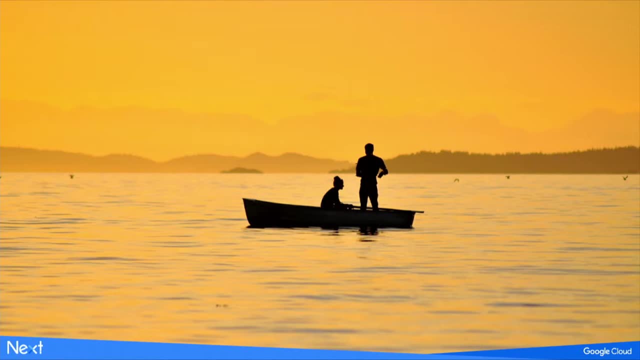 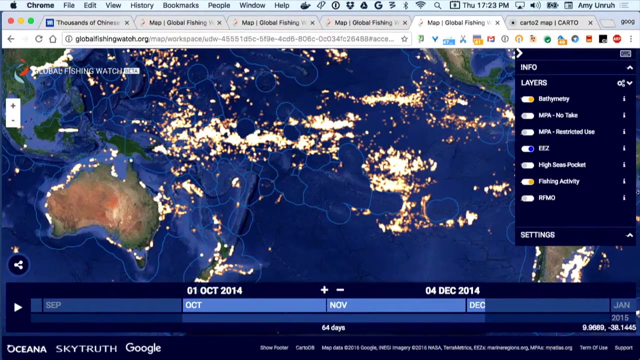 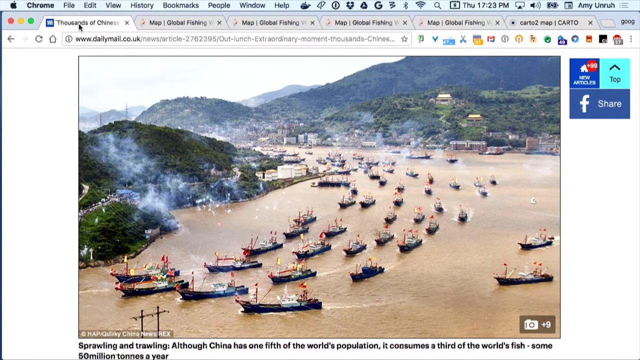 And this is what I do as fishing, and this is what most people do. But most of the world's fish are actually caught by boats, And they're caught by boats like this. This is a picture of China. Each of these boats is about 100 feet long. 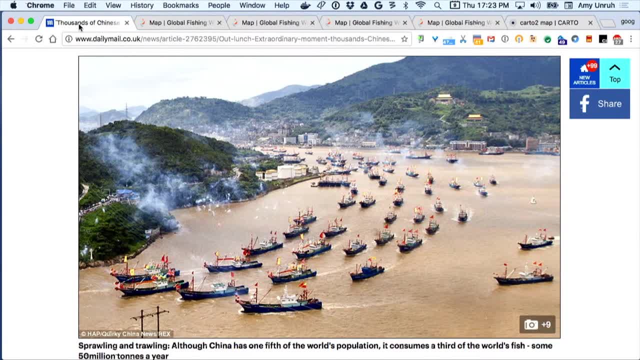 And the way that China manages its fishery in order to prevent overfishing is they have a three month moratorium on fishing, at the end of which everyone's allowed to go out, And this is at the end of the moratorium, when all the fishing vessels are about to go out to the ocean. 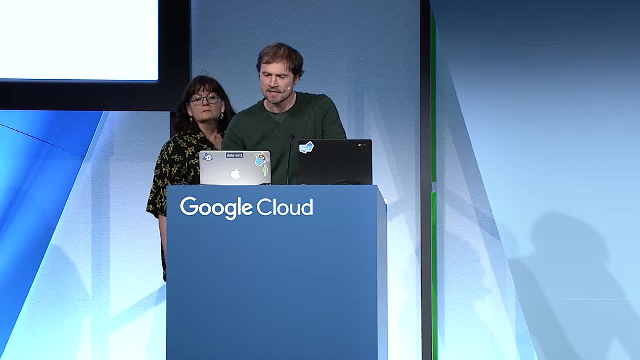 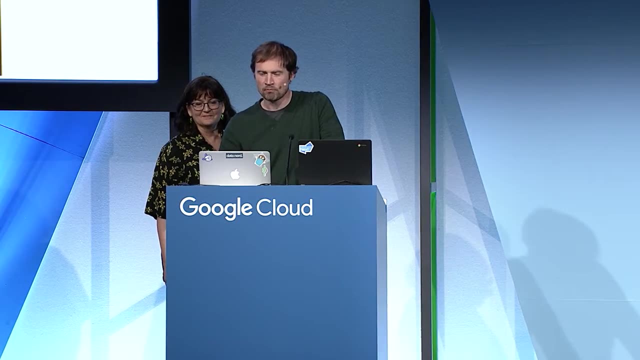 And so it gives you a sense, when you can see all the boats at once, what is heading out for you if you're a fish, And this is really remarkable. But this is not to pick on China. This is happening all over the world. 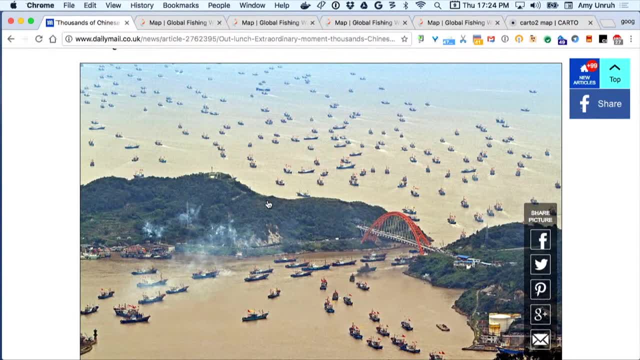 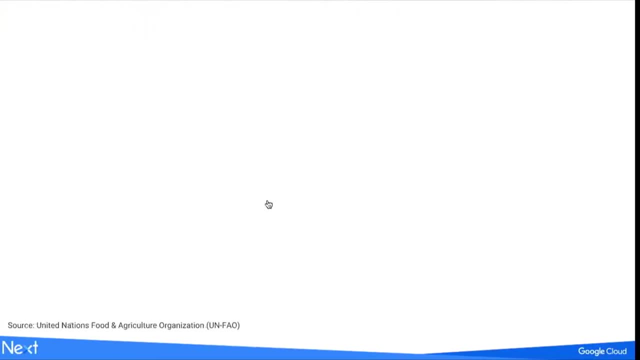 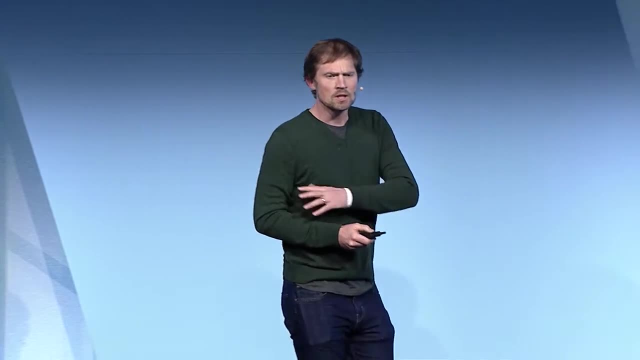 And it goes over out into the ocean and extracts fish from this shared global resource And it's kind of an ultimate tragedy of the commons. And the reason we care about this is because fishing is such a huge problem. So about 1 billion people in the world rely on fish. 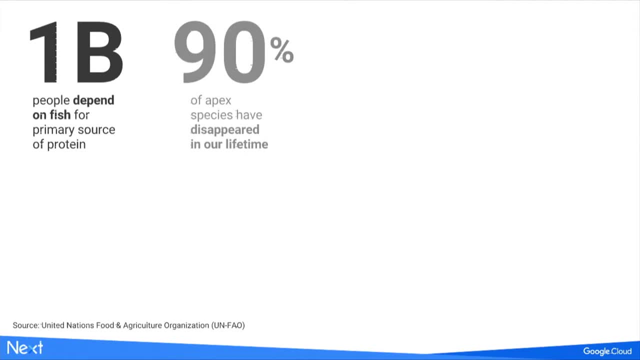 as the primary source of protein. But the oceans are very overfished. 90% of apex species have disappeared in our lifetime, So that's big things like shark and tuna. About 85% of the world's fisheries are either overfished at capacity or recovering. 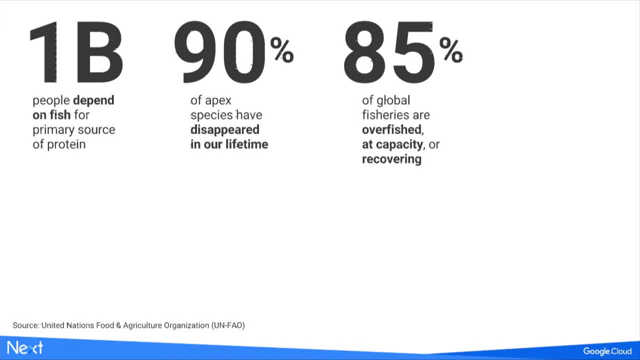 from having already been overfished. And perhaps the most important number here is this one, one in five, which is the amount of fish which is we call overfishing. It's called IUU or illegal, unregulated or undocumented. 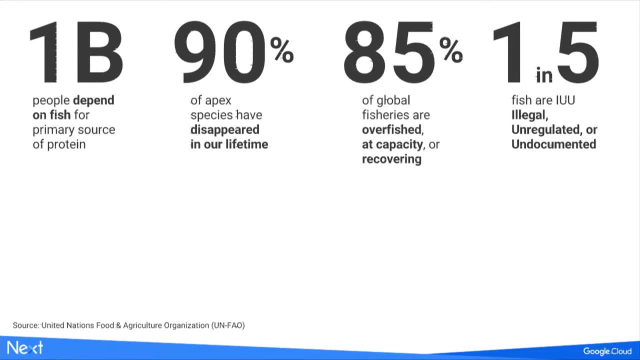 Essentially it's fish where we don't know where it came from. And if you imagine, you have a huge shared resource and you're not even able to measure where 20% of it comes from. that's one of the reasons you're going. 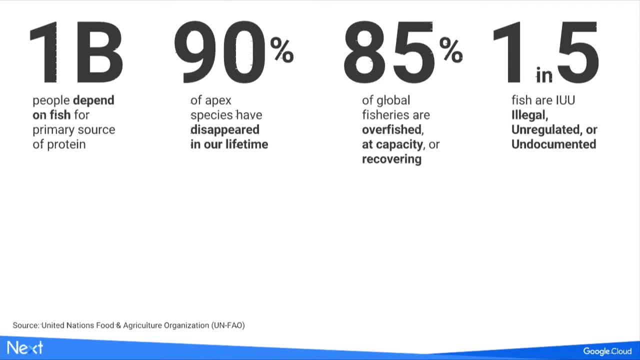 to have an overfishing problem. At the same time, this is a problem which really requires a global approach. 38% of fish is traded internationally, 55% comes from developing countries, with an export value of $60 billion. So, in summary, overfishing is a huge problem. 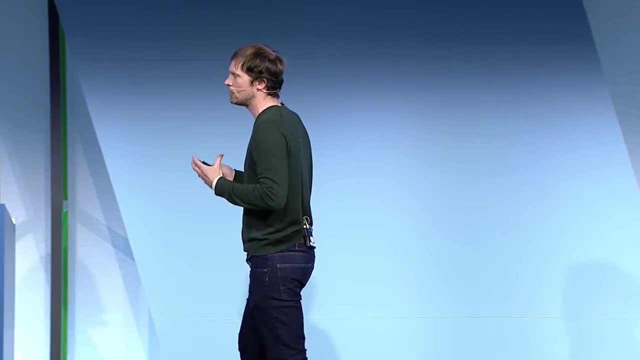 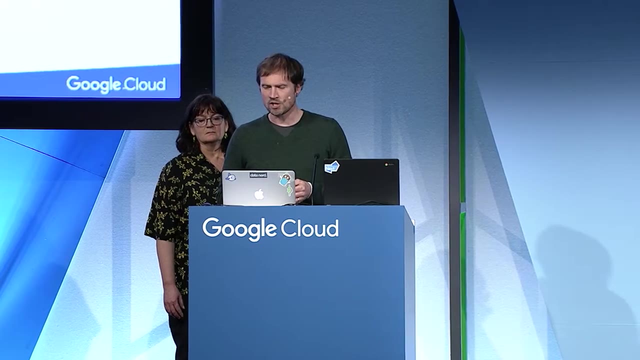 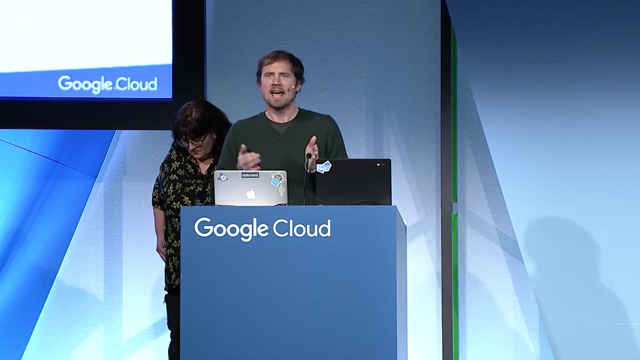 It desperately needs transparency and requires a global approach to address, which is why we developed Global Fishing Watch. So Global Fishing Watch takes data from transceivers on boats which broadcasts their locations, And these are big industrial boats, not the small ones. 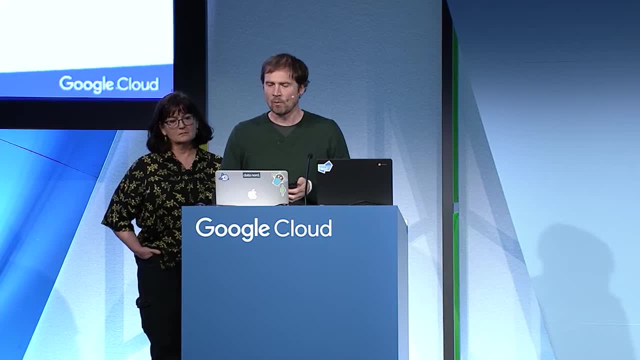 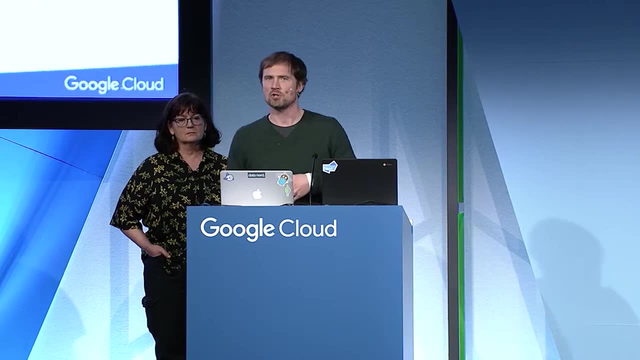 and maps out how they're moving and then identifies where and when fishing is talking. If you go to globalfishingwatchorg, you can look at our map. It's almost near real time, so it shows fishing from three days ago to five years ago. 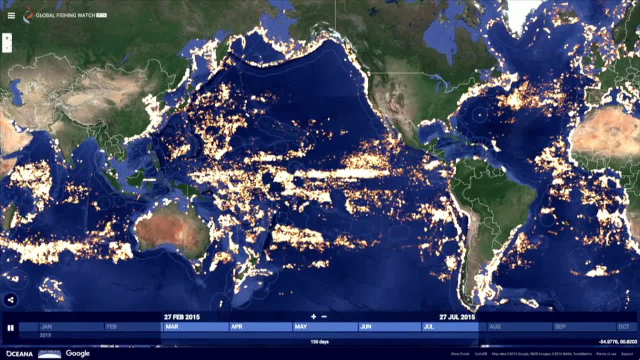 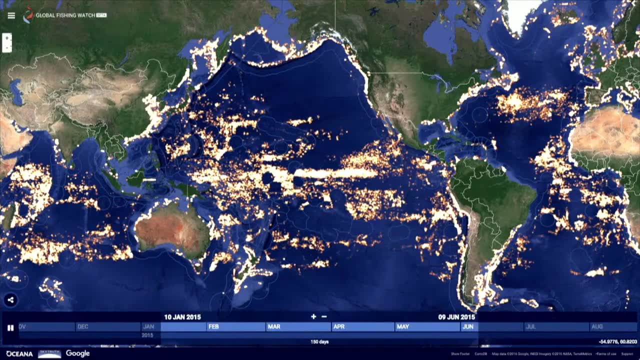 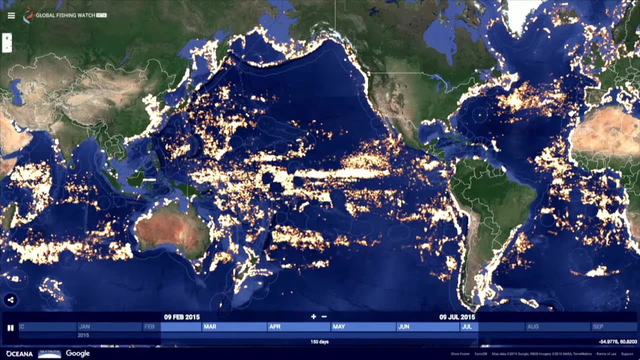 And it looks like this And it animates and shows you where fishing is happening. And I love looking at this because every time you look at it I see something new. You can see patterns of fishing along the equator where there's upwelling bringing nutrients. 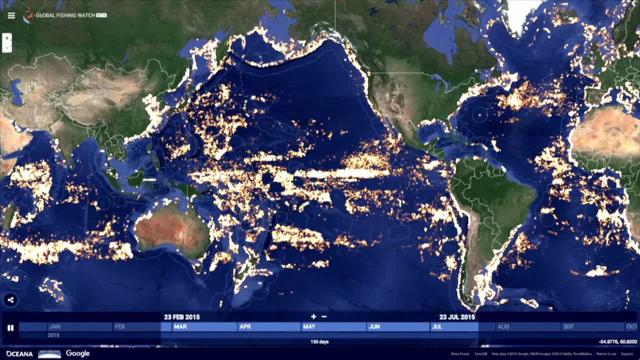 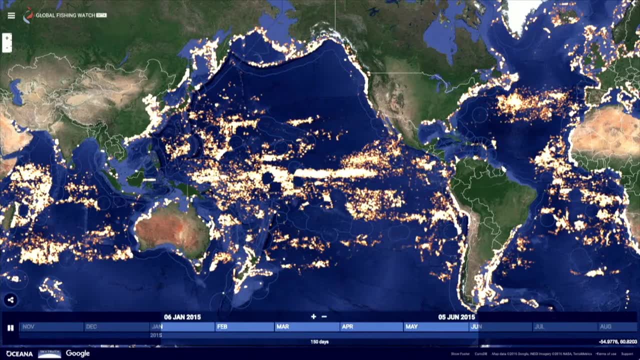 A lot of tuna fishing happens there. You can see fishing all along the continental shelves, because that's where a lot of nutrients are, a lot of fishing is. You can see political boundaries where a lot of some type of fishing vessels aren't allowed to fish within certain country waters. 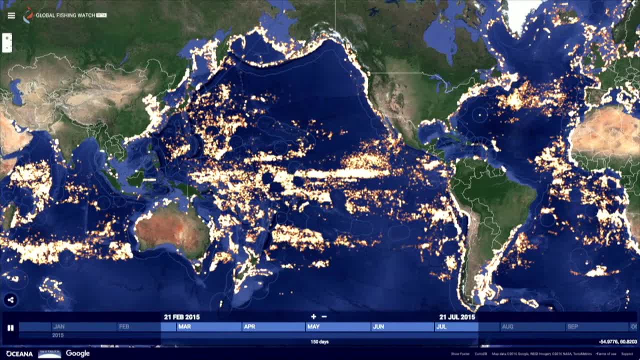 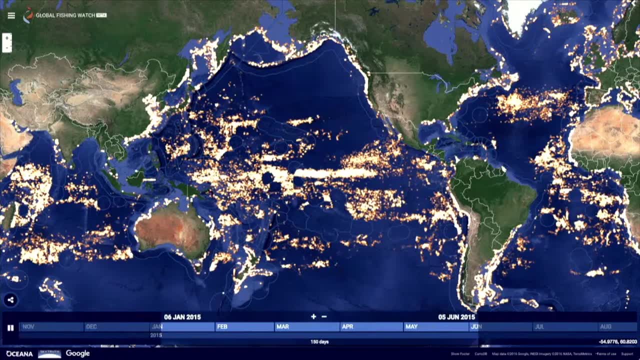 so they fish right along the edge of it. And you can also see where people don't respect the boundaries of different countries. You can see Australia, right there. You can see fishing happening right along the edge of it. You can see in Africa, people ignoring some of those lines. 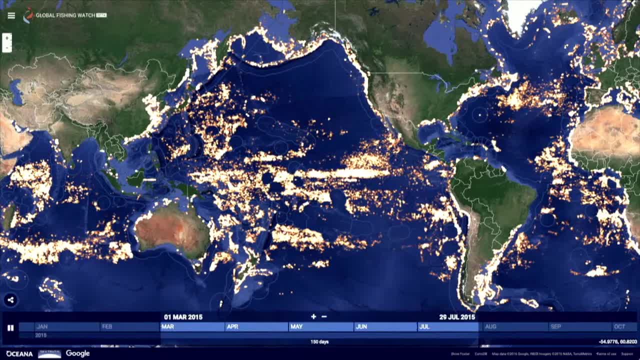 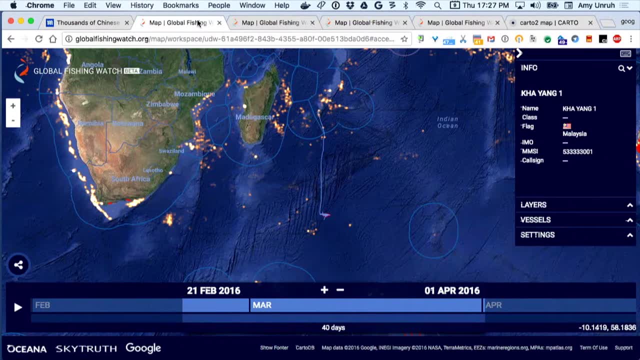 So I'm going to now switch to our website so you can see what it actually is, So you can click on individual vessels. So this is actually our live website And you can watch them move. So here I clicked on this one, which is the Kai Yang 1.. 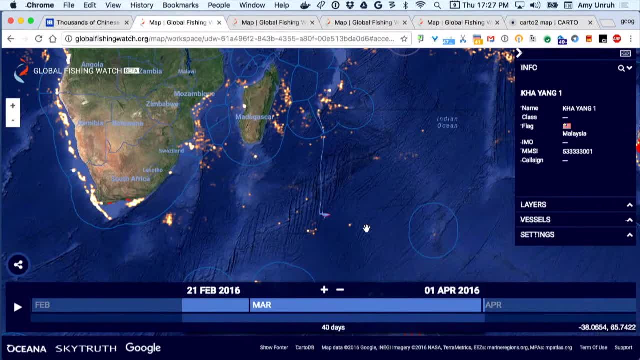 So each of these- and I should explain each of these little yellow dots is where we think a fishing activity happened, And so if you hit play, you can now watch where this boat is moving, And this is a Malaysian boat, the Kai Yang 1.. 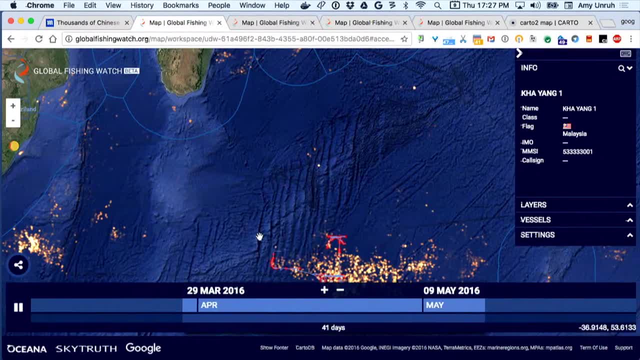 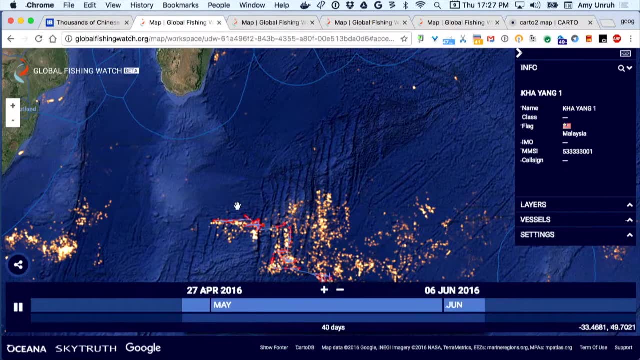 It's a long liner, which means it sets long lines of hooks, Sometimes as long as 100 kilometers, and then retrieves them, And so here you can see it moving back and forth across the ocean. All the other dots are where there's other boats fishing. 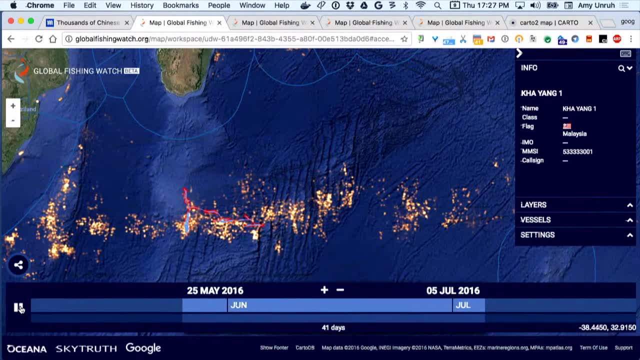 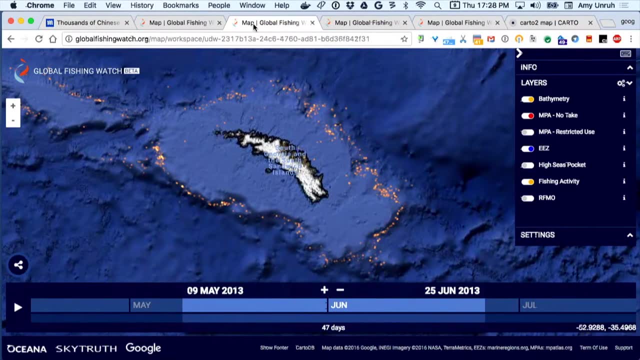 here as well, You can see interesting patterns, such as here: Here's an island in the southern Atlantic. You can see fishing happening right along the edge where the continental shelf ends And that's, and you can see that the, the, the, the, the, the. 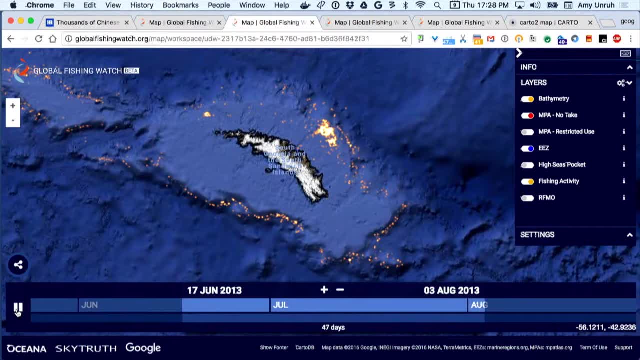 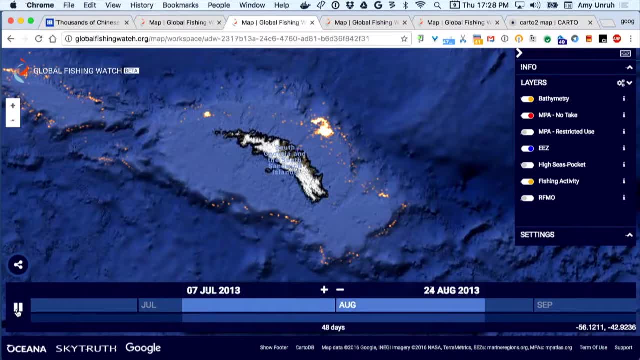 of the ocean where upwelling happens right along the edge, and that's where fishermen are are are directing their boats, And so there's all types of interesting patterns we can use to gain insight in how to better manage our oceans. So that's, that's the tool, that's the exciting thing we've. 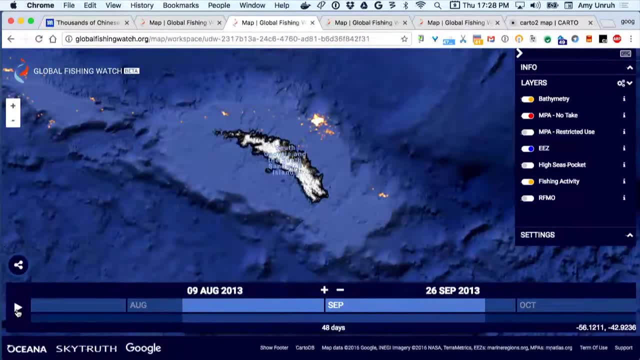 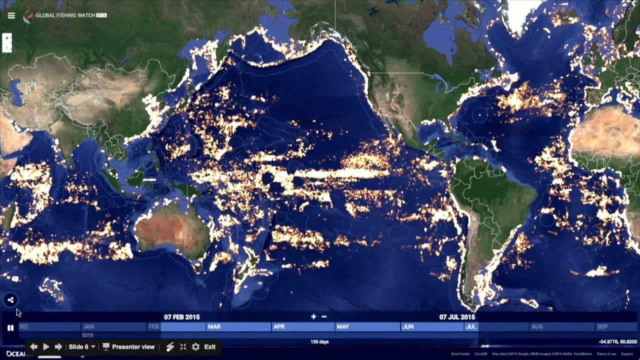 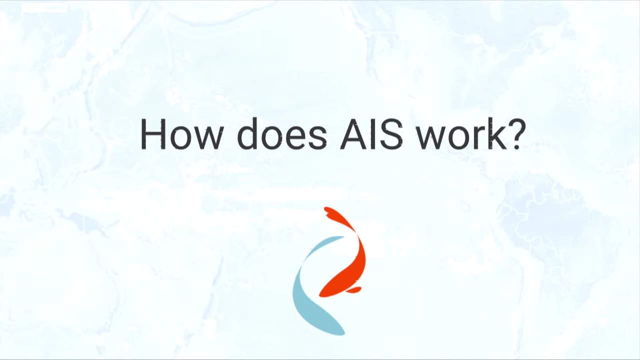 built And we're going to spend the rest of the time here talking about how we built it And hopefully that empower you to be able to do some of the same types of machine learning- machine learning techniques. So the core technology to this is called AIS, which stands for the Creatively Named Automatic. 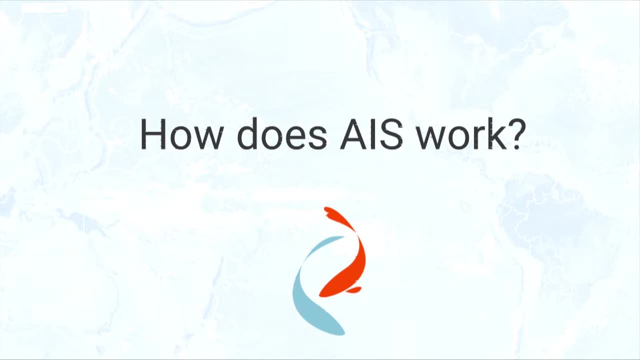 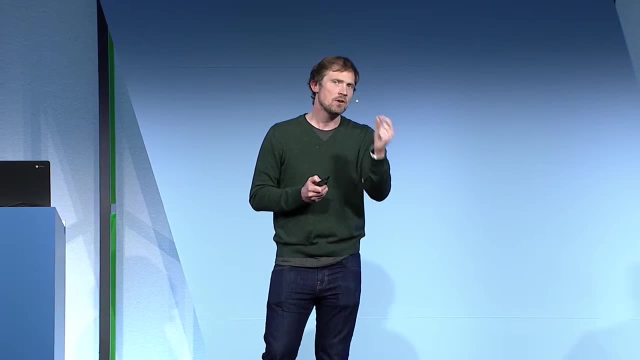 Identification System, which is something that all large fishing vessels are required to carry, And it's a safety mechanism. The idea is you broadcast your location so that other boats nearby can see where you are. This is very important in some parts of the ocean. 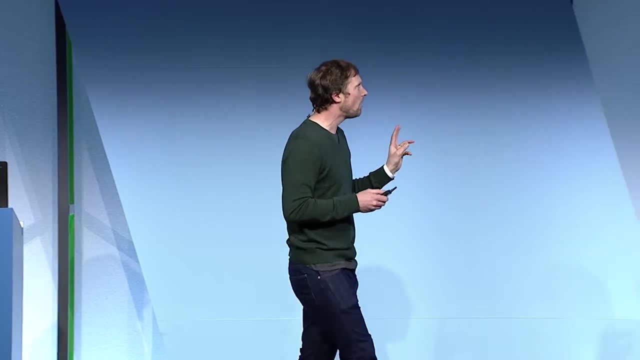 Here's a chart of boats in the English Channel, and all of these boats want to make sure they see where the other ones are so they don't collide with them. If you're in a boat with an AIS device, it looks like this: 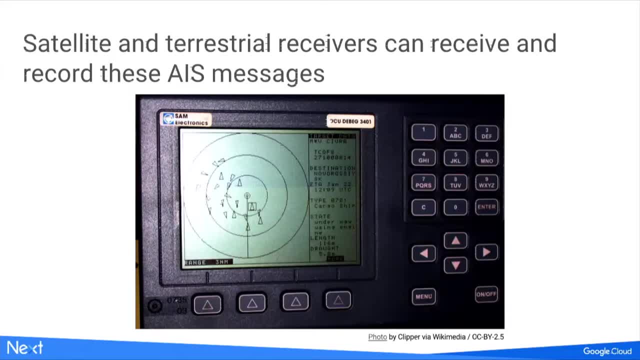 And you can see. you know it just brought. you can see where all the other boats are nearby you. It tells you the name of that boat, which direction it's headed, its speed, all types of useful information to help you not collide with it. 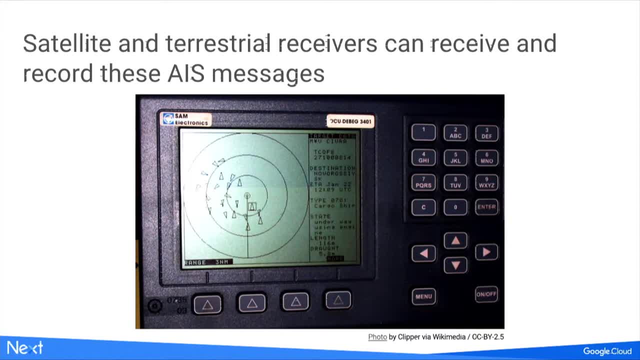 These signals, though they can be picked up by satellite and also by receivers along the land, terrestrial antennas. In the last few years, a few companies have launched satellites which collect this data, and we have finally been able to do that. We've been able to build a global database of AIS signals. 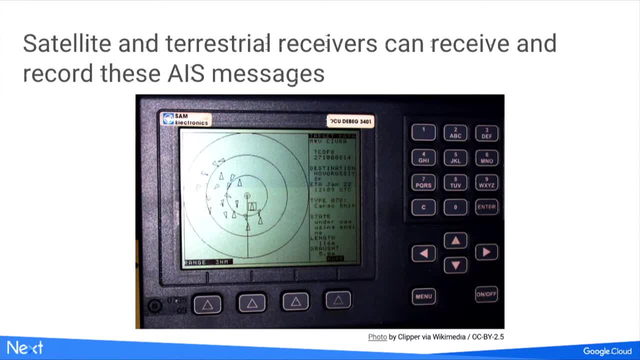 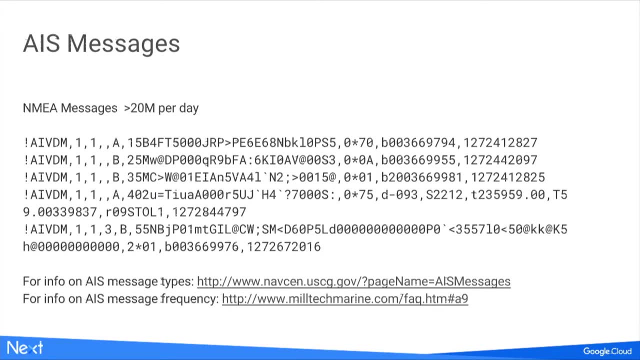 And that is what we have been collecting at Global Fishing Watch and working with Oops. I was back. The AIS message looks like this: It's an NMEA message. is the type: There's a Googler who wrote a library that we used to parse it into a readable JSON file. 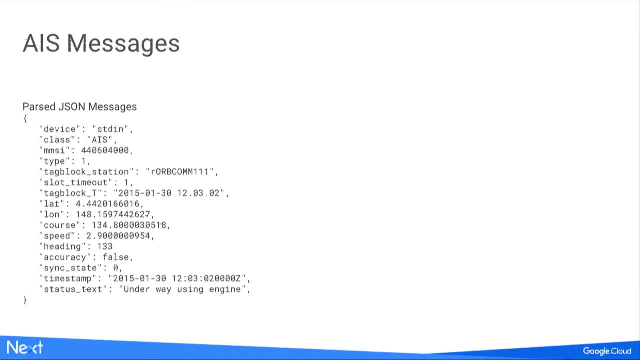 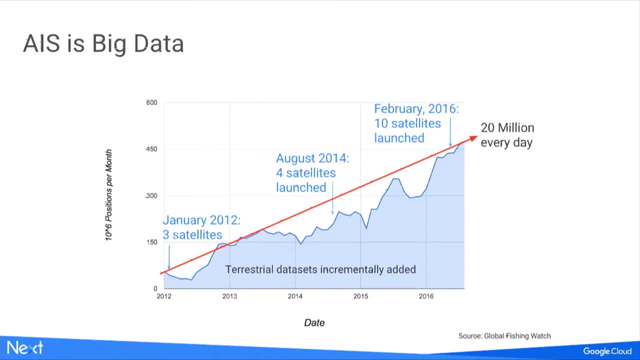 and this is what it looks like. It has, you know, information about the latitude, the longitude, the course, the speed, the heading, as well as some other information, And we get about 20 million of these data points a day. 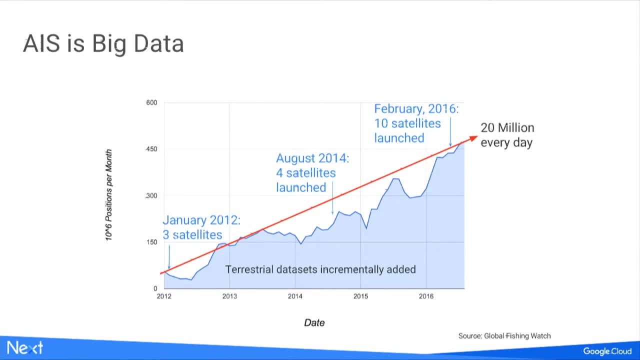 As you can see, like all other data graphs, it's going up because there's more. now We have about half a billion a month. In 2012, we were getting far fewer because fewer boats had this technology and we had fewer satellites and fewer terrestrial antennas. 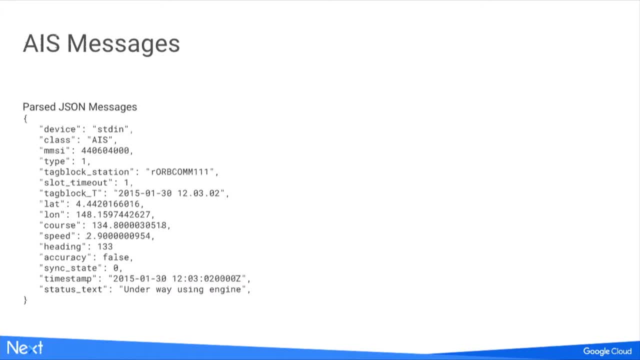 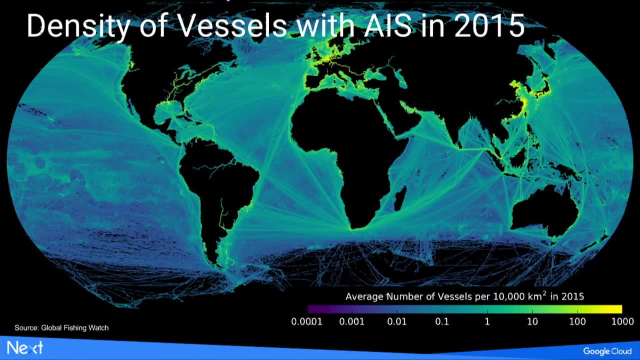 So we're getting more and more data every month, And when you map out what all the boats in the world look like, you can see that they're all the boats in the world look like. It looks like this: There's somewhere between 300,000 and 400,000 vessels with AIS. 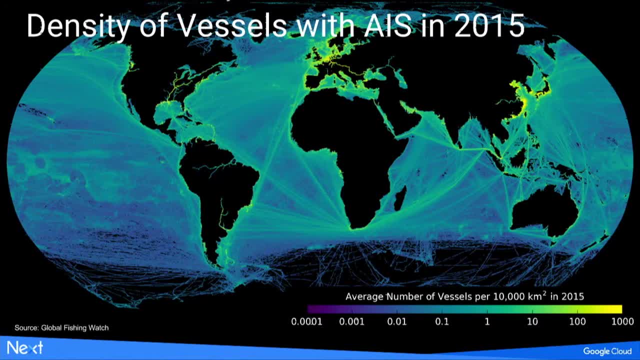 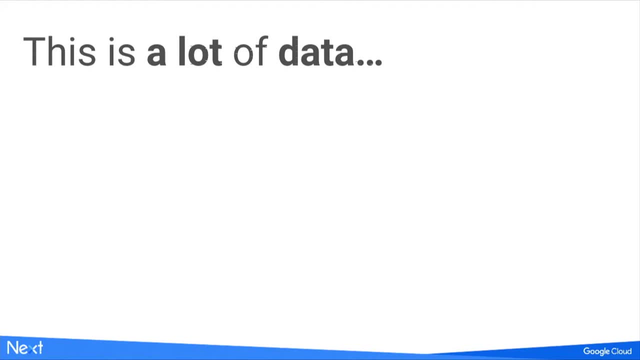 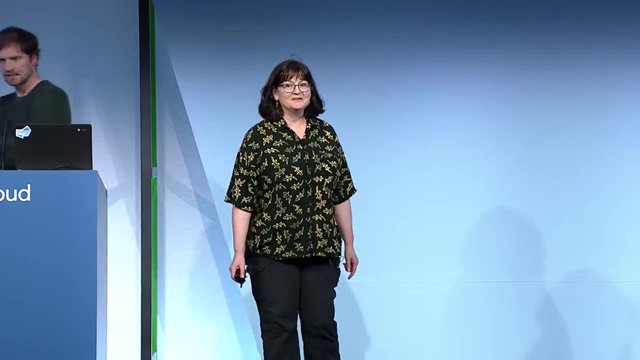 This is all of them, not just fishing vessels, And we- about 80,000 of these- are fishing vessels and that's what we identify to determine fishing effort. Okay, so, this is a lot of data. When I started looking at it, I was startled to find that every day, 15 gigs was getting. 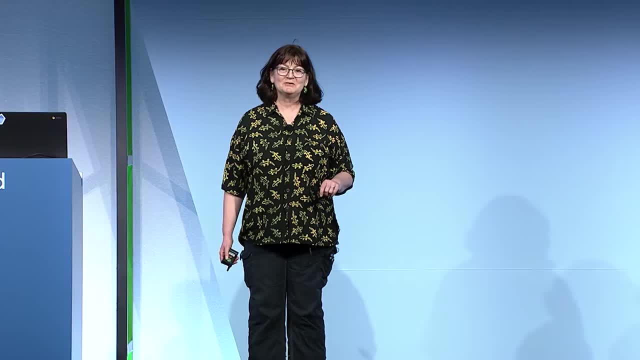 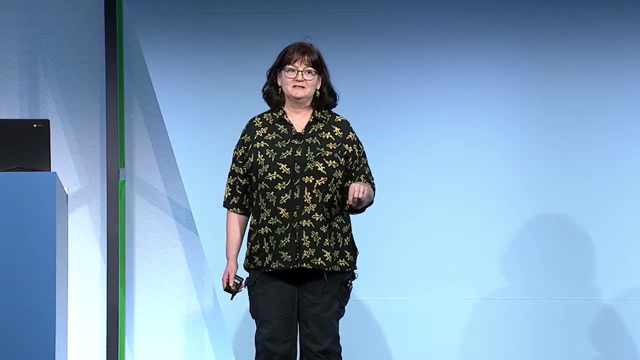 dumped Of this data. it was getting dumped into Google Cloud Storage, And so not only is a lot of data to kind of shuffle around, but if you're going to analyze it in any meaningful way, it requires a lot of compute power. 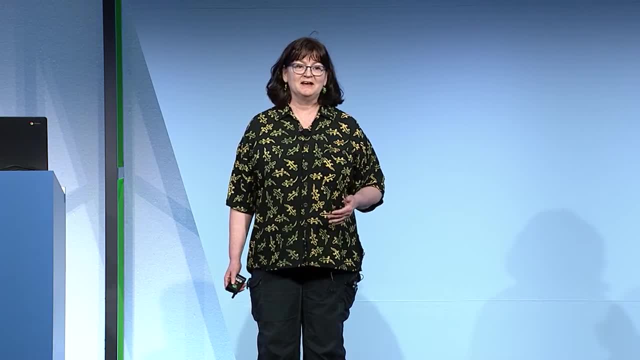 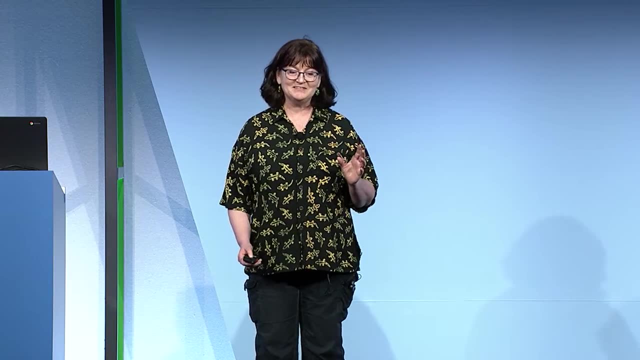 And so Global Fishing Watch would kind of like to not have to worry about that, about shuffling large amounts of data around, about provisioning VMs when they need it, And so you can probably guess the punchline: Google Cloud Platform to the rescue. 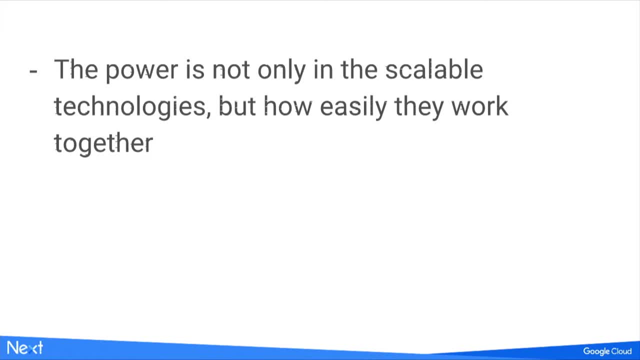 So what I'm going to talk about is the workflow that they're using and how they put together some Cloud Platform products to do what David described on that globalfishingwatchorg site And I'm going to focus on for this talk on Dataflow and Cloud ML Engine, but they're 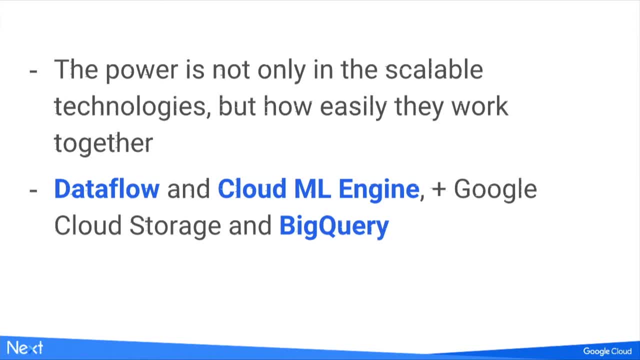 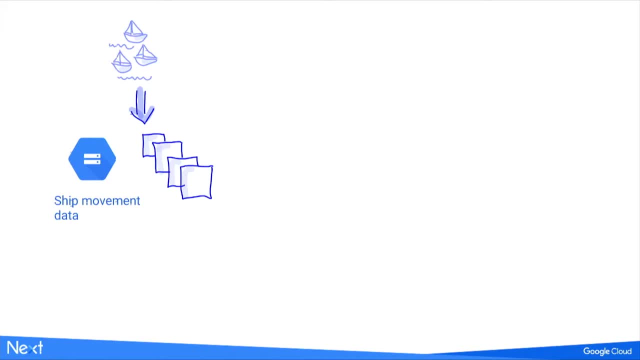 also making a lot of use of other stuff, in particular BigQuery, And David's going to end Cloud Storage, So let's get started. David's going to talk a little bit more about the BigQuery later. OK, so this is kind of a typical workflow. 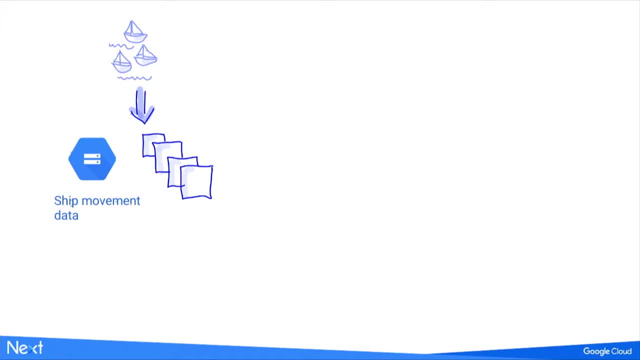 And they actually have several of them that follow this pattern. So, first of all, a lot of shit movement data- remember, it's like about 15 gigs a day- is getting dumped into Cloud Storage And then periodically, in batch mode, they're running Dataflow jobs. 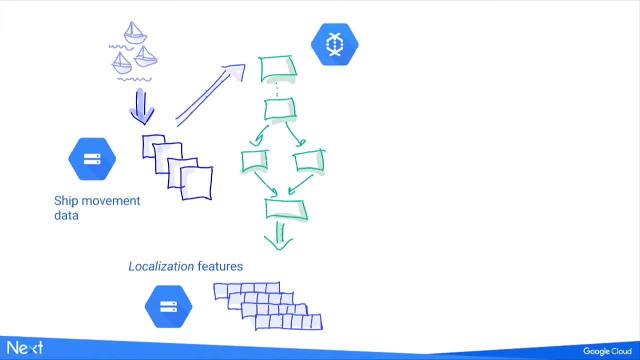 And they're going to have to do a lot of work to process this data, to transform it, to aggregate it, And the output of that Dataflow batch pipeline features, using the term in the sense of input to a machine learning model. So they're outputting data that is cleansed and aggregated and transformed into something. 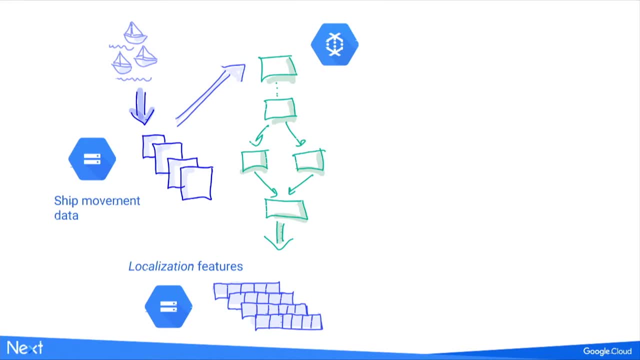 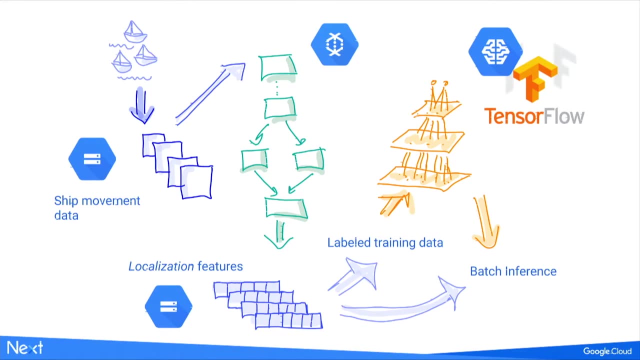 that they want to feed into a TensorFlow model. OK, so then you can probably guess that the next part of this workflow is TensorFlow and Cloud ML Engine. So they've got, the features are being generated, And then there are sort of three parts to what happens next. 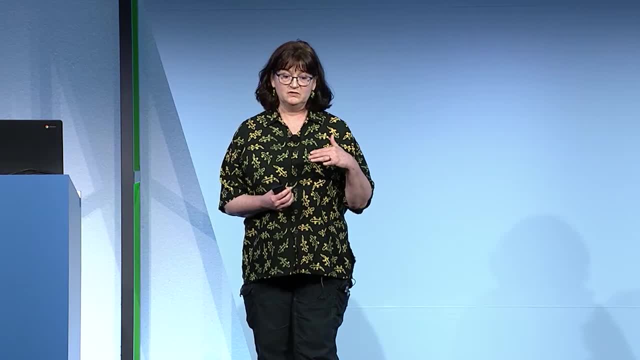 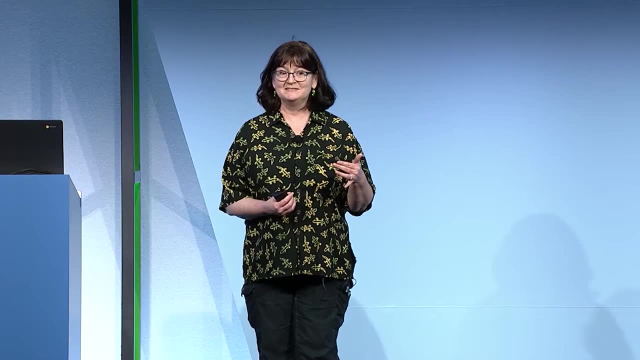 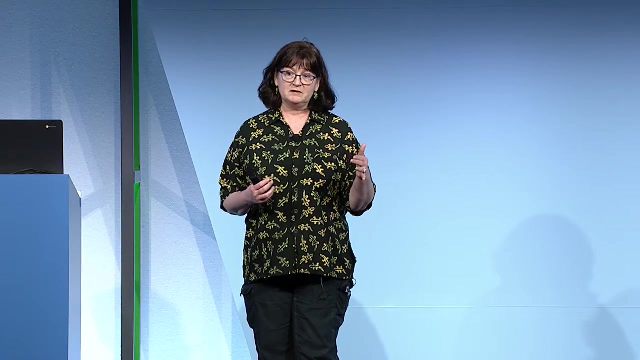 So the first part is generating the training data, of course- And as those of you who have done this kind of thing might know, that can definitely be non-trivial at times. David's going to talk a little more about that. And then they've built some very interesting convolutional neural nets to do classification. 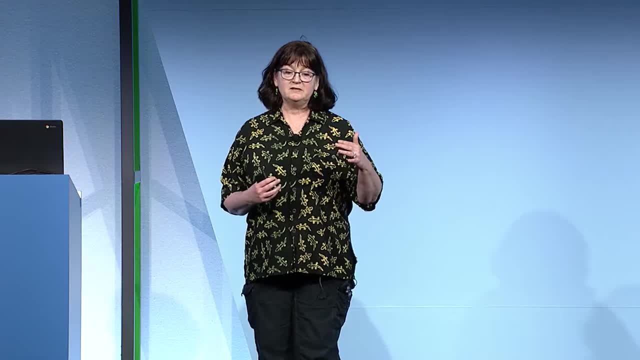 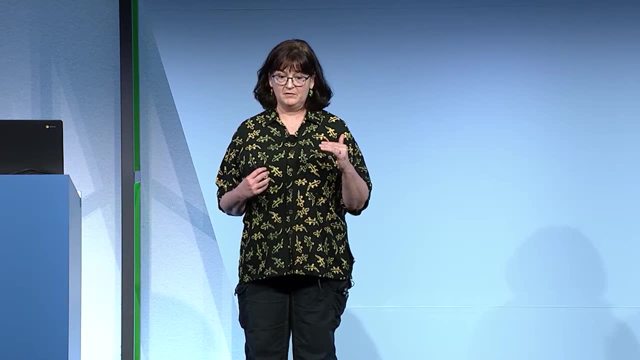 You'll hear a little bit more about those. So label the training data, train the model. So they're using Cloud ML Engine to do distributed training of the model, of the TensorFlow model, And then, once the model is trained, they use it for inference. 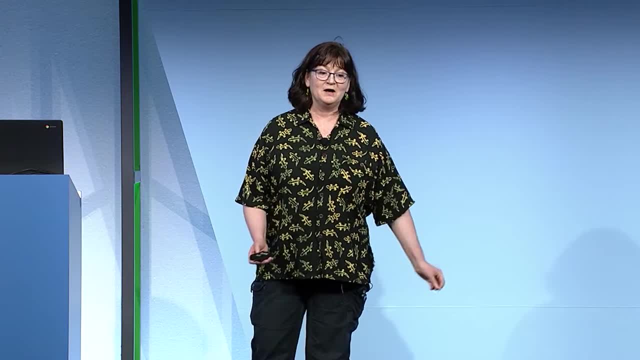 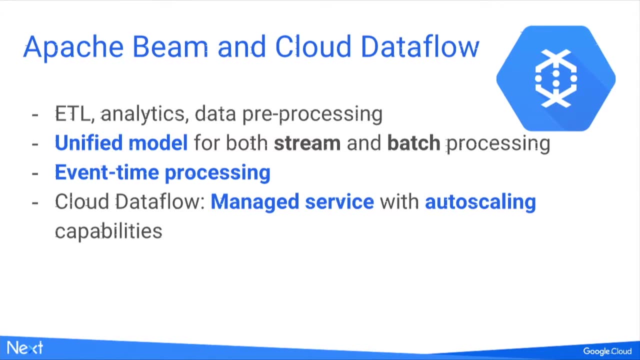 So to dive a little bit more into some of the pieces of this. So this is probably some of you who have been to talks that go into this in more detail. But for those of you who haven't, let me say a little bit first about Apache Beam and Cloud. 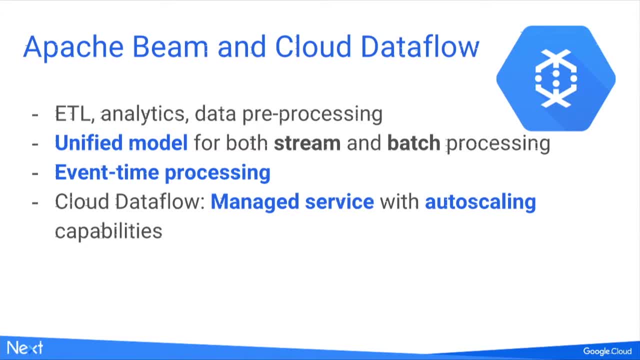 Dataflow. So Apache Beam is a unified model for building data processing pipelines that can handle both bounded and unbounded data- You know bounded, Batch and stream processing- And Apache Beam is also a set of SDKs for building these pipelines. And one particularly salient point about the model for the purposes of this talk is the 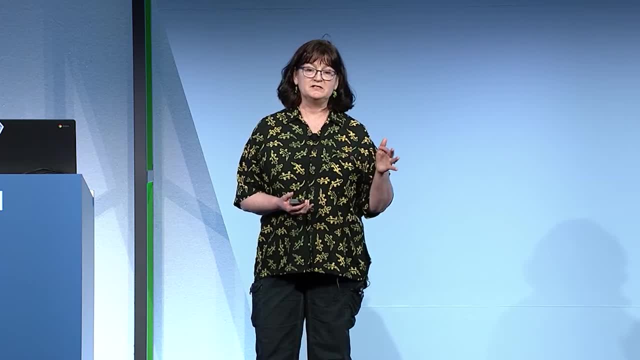 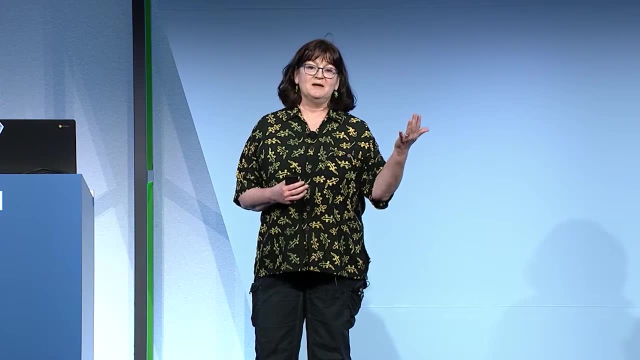 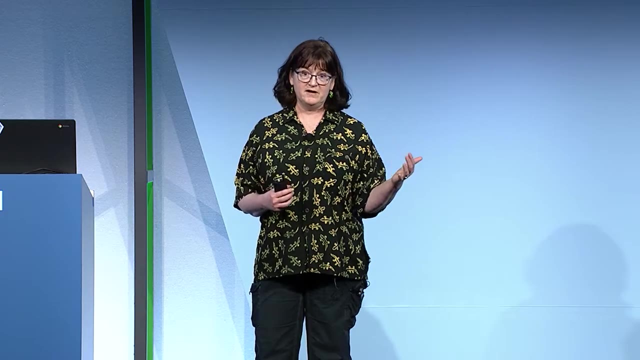 way that Beam does event time processing. So you can tell Beam- I want you to analyze this data with respect to the time it arrived at the pipeline, Or you can tell it. I want to analyze this data with respect to when it was actually generated. 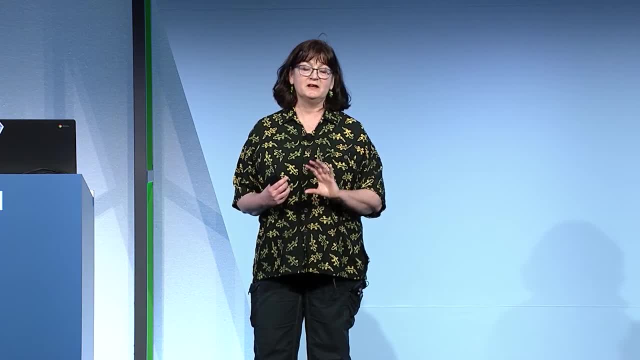 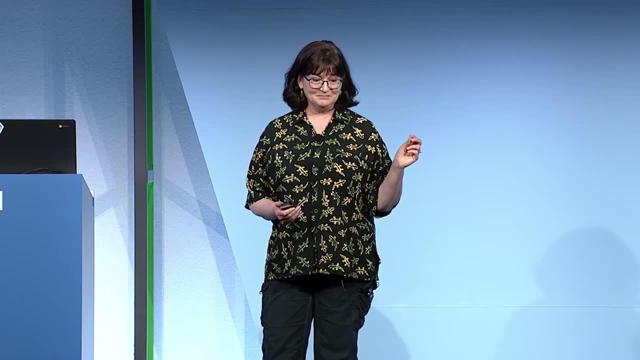 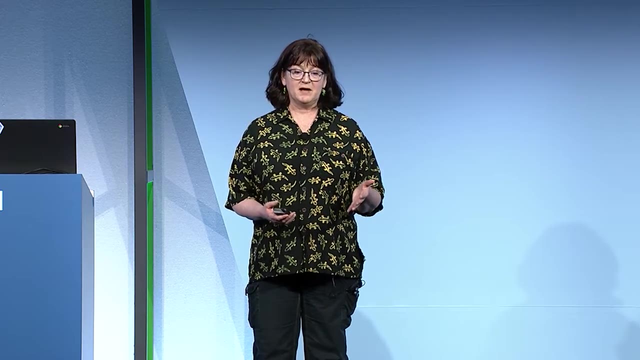 And we need to do that latter thing. for the global fishing watch data, We want to say: do your analysis with respect to the time this was actually logged by the ship. So then, Cloud Dataflow is a managed service for executing these Beam pipelines. 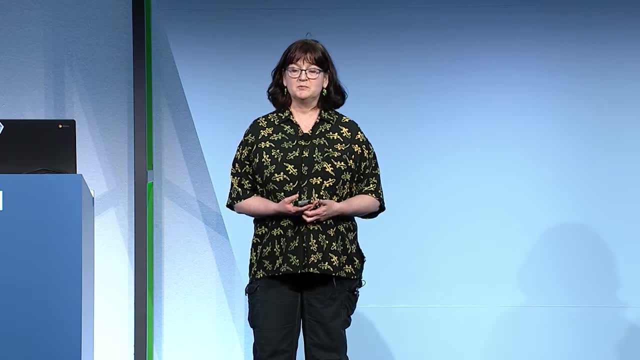 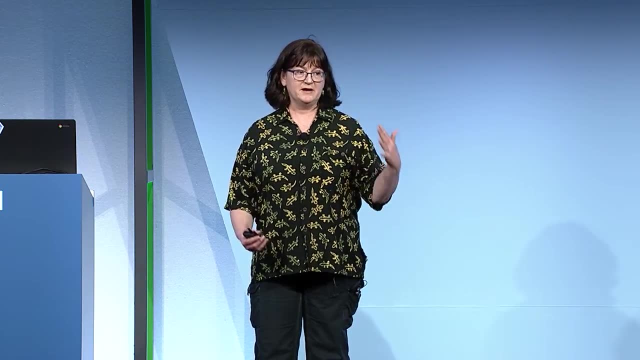 And one nice thing about it is that it supports auto scaling, So it will prevent that. It will prevent that. It will make sure that the data is stored in a secure environment And it will help to keep the provision workers up and down as it needs them while it's running. 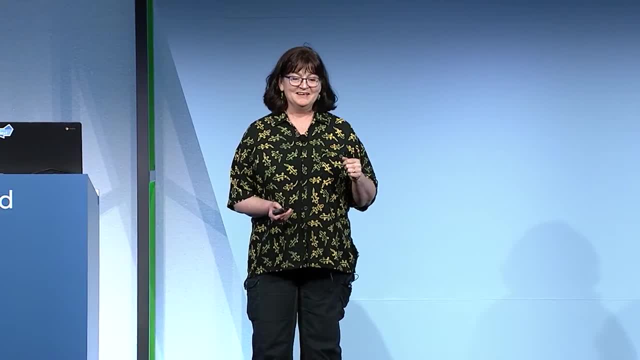 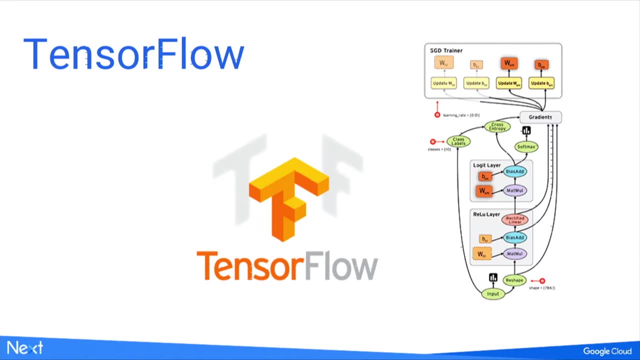 a big job. Okay, So that was Dataflow, the middle green piece there. Let me talk a little bit about TensorFlow and Cloud ML Engine. So again, some of you have probably heard about TensorFlow in the past couple of days. This is an open source platform for doing numeric processing. 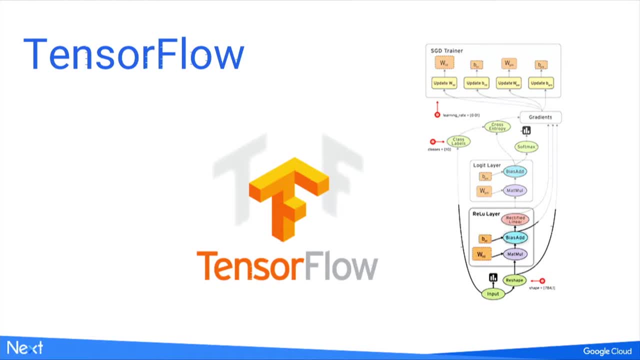 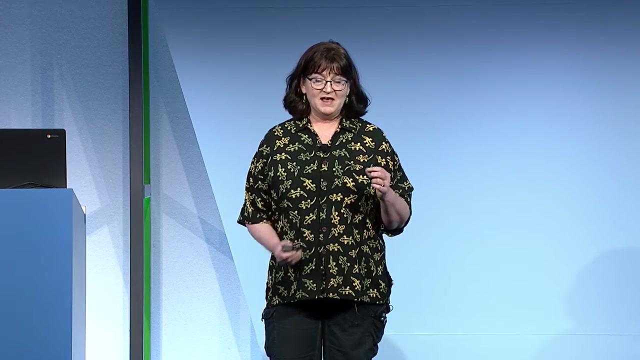 It's a very well documented DOM machine that allows you to do numeric computations with data flow graphs, But in particular it's particularly good for building and training deep neural net models. It has a distributed runtime. It supports auto differentiation. It was sort of built for deep learning. 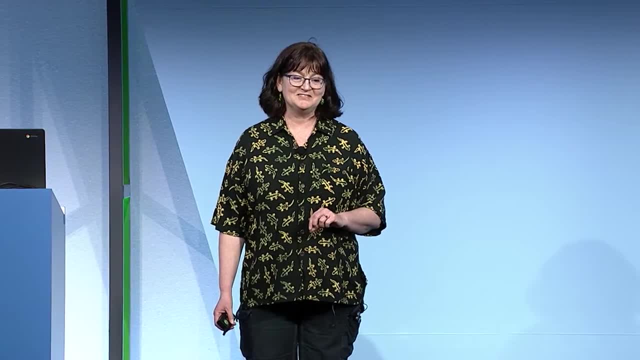 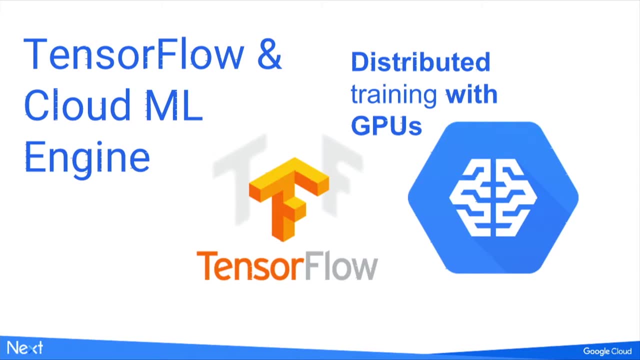 So Cloud ML Engine, Which those of you who attended yesterday's keynote know has just gone toналnet. Thank you, Bye to GA, then is a managed service for training. doing distributed training of your TensorFlow models with GPUs are now available, if you like. 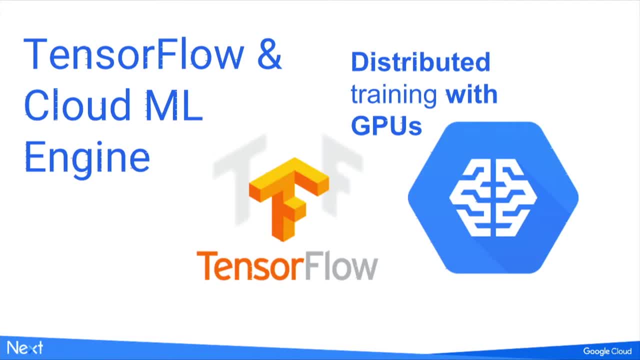 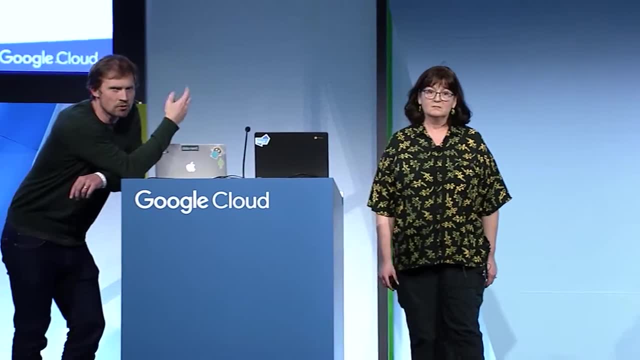 and then for serving the model once you've trained it. So we'll talk a little bit more about that later. And I should note that we've been using these GPUs and see about a 10 times improvement in our model training and inference using the GPUs over the CPUs, which 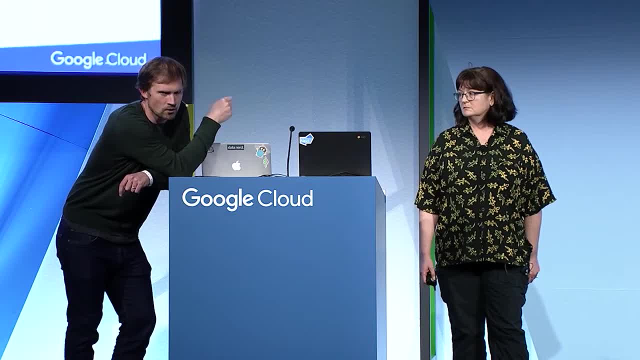 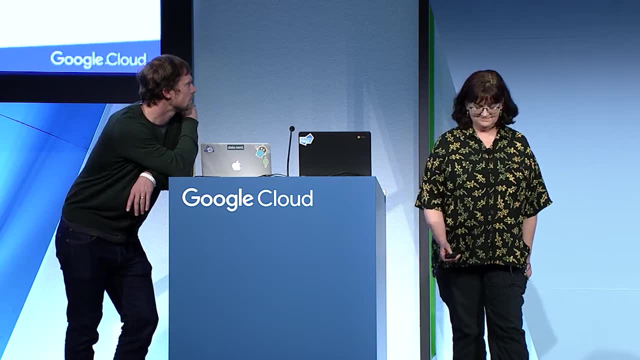 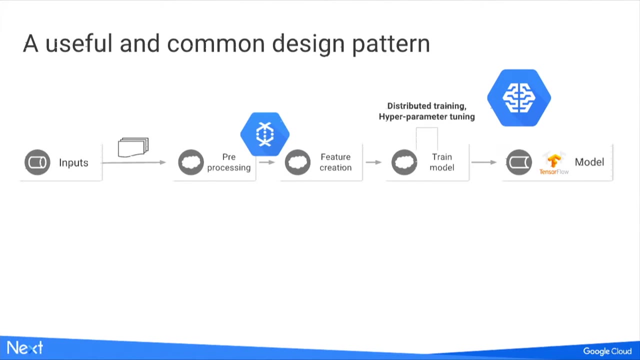 has been incredibly useful, especially right now. I'm actually having some back and forth with our machine learning engineer and doing lots of iterations on the model, and it's really helpful to have those fast processors. OK, so that was a workflow that Global Fishing Watch is using. 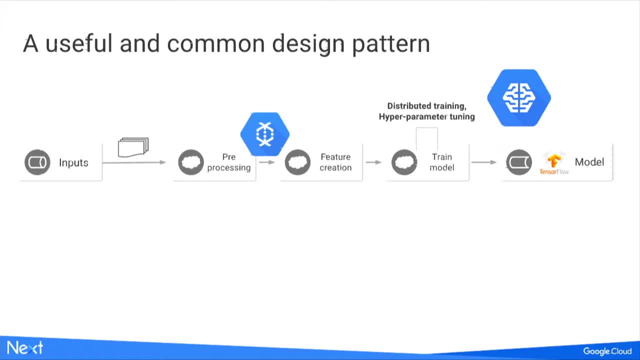 but actually it's much more general than that And this is kind of a useful and common design pattern where you want to do a lot of data, you want to do a lot of preprocessing and features, You want to do a generation and then you want to train a model. 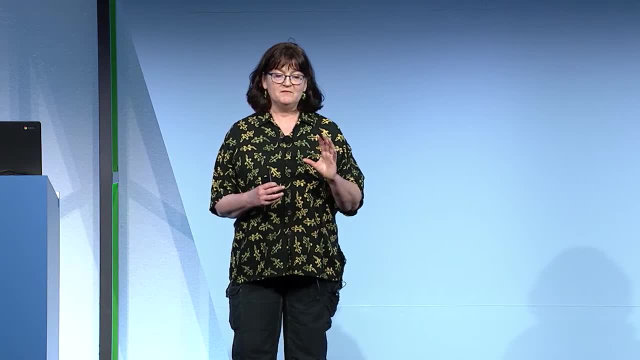 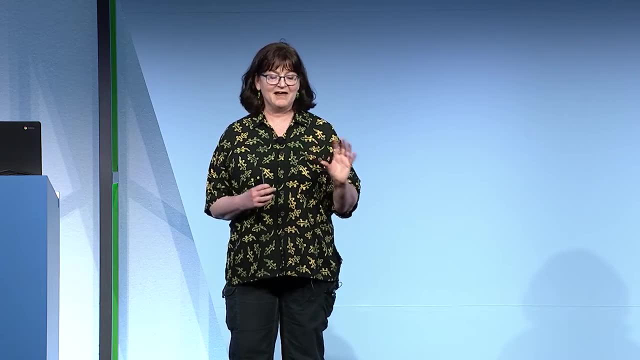 And so if you do this all in the cloud, you don't have to worry about scaling up, You don't have to worry about shuffling very large amounts of data around, And that's kind of what this suggests. Do your preprocessing with Dataflow. 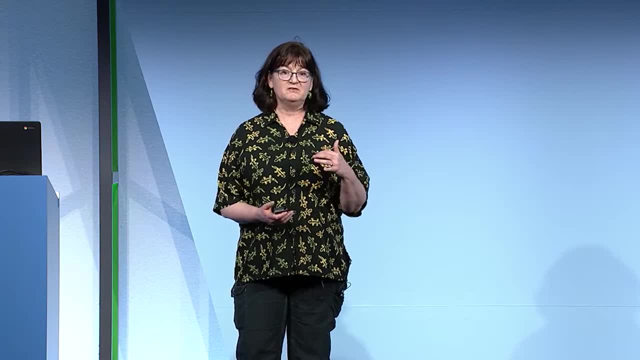 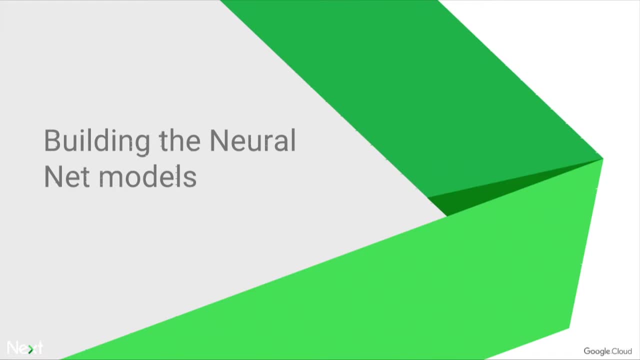 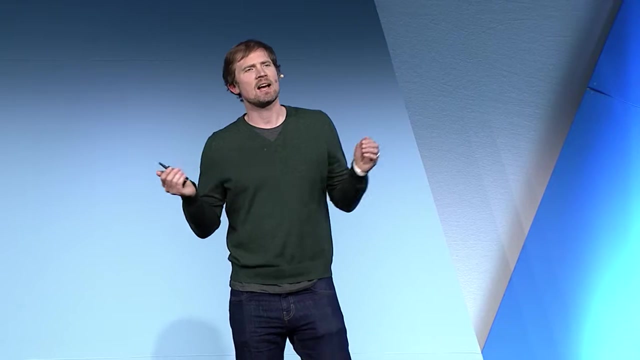 send the result to Cloud ML to do distributed training of your TensorFlow model. So I want to talk now about how we actually built the net and how we got the training data for it. So we have two main classification problems with Global Fishing Watch. One is vessel identity, so identifying 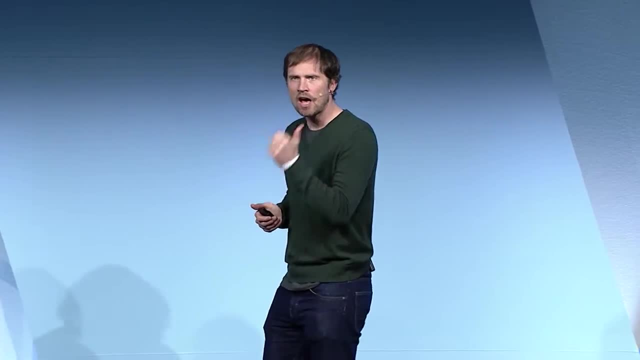 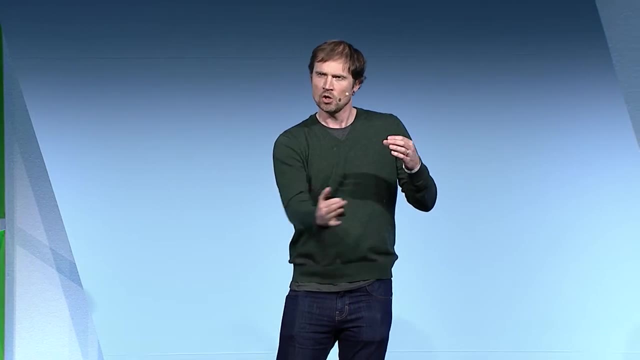 what type of boat it is and what type of fishing it is doing. It matters a lot for conservation and for marine spatial planning whether or not the boat is fishing with a trawling net which drags along the bottom, or if it's fishing with these. 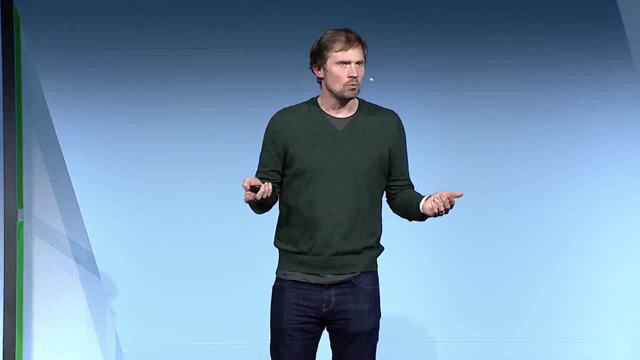 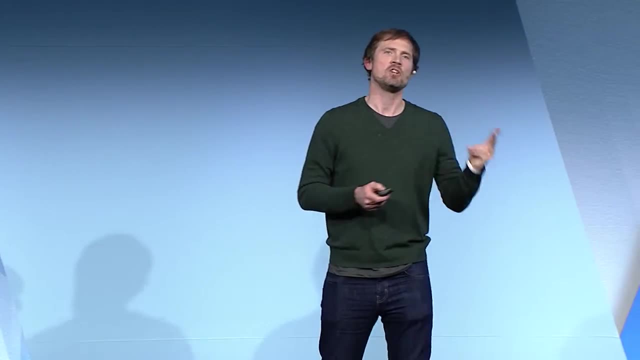 uh, long lines of hooks And they don't tell you what it is in the AIS message, so you have to look at how the boat moves to identify it. The second problem is identifying when they're actually fishing and when they're just transiting from one place to the next. 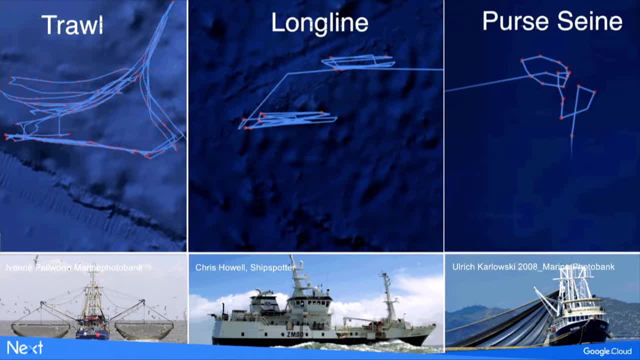 So here you can see these are three of the major types of fishing boats. There is a trawler, longliner and purse saver. They move differently. There are some pictures of these large vessels And your eye can see the difference. 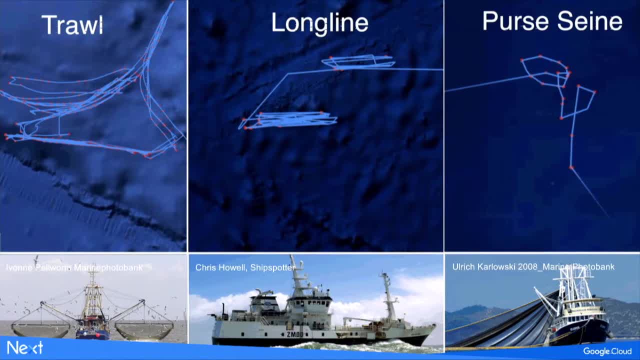 and so we can train a machine to see a difference as well. The hard part we had to in order to train them, train them. we had to train this model. we had to get a few thousand examples of these boats, And we did that by matching the AIS data. 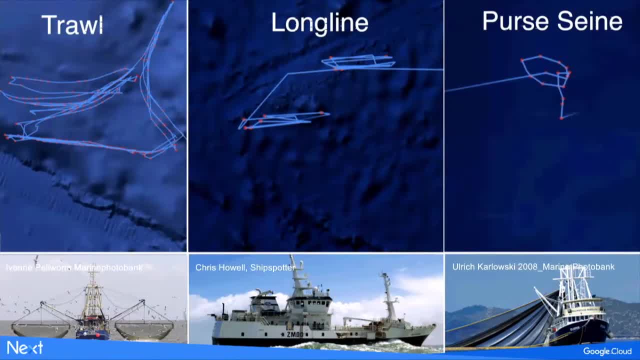 to official registries, which involved a lot of fuzzy logic and fuzzy matching. From that we got a few thousand boats from which we were able to match a few um, a few hundred, identify a few hundred thousand boats, And I should add that we were also 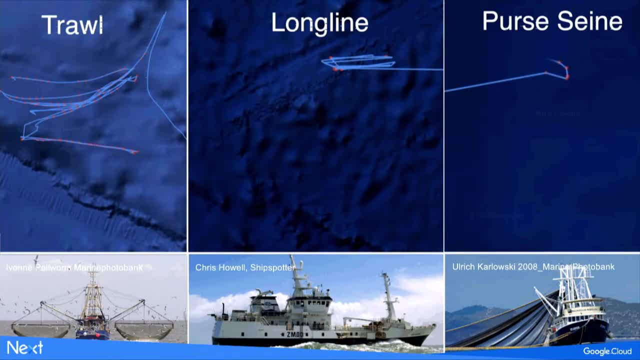 identifying non-fishing boats because, remember all the boats with AIS, most of them are not fishing boats. You have to be able to tell what's a tugboat, what's a longline fishing boat, what's a tanker. Second problem: 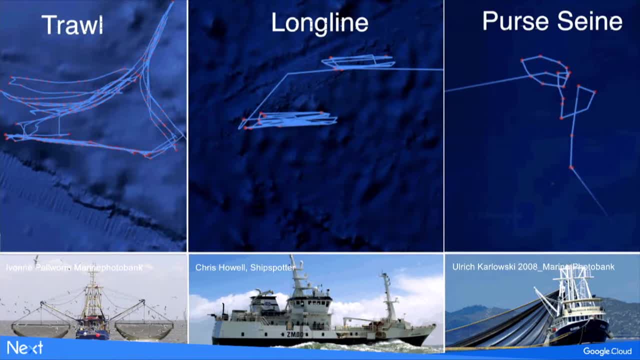 Second problem is identifying when the boat is fishing, And to do that, ideally you would have some logbook from the cap, some logbook from the captain that would tell you when and where they put their gear in the water. Problem is that one captains rarely. 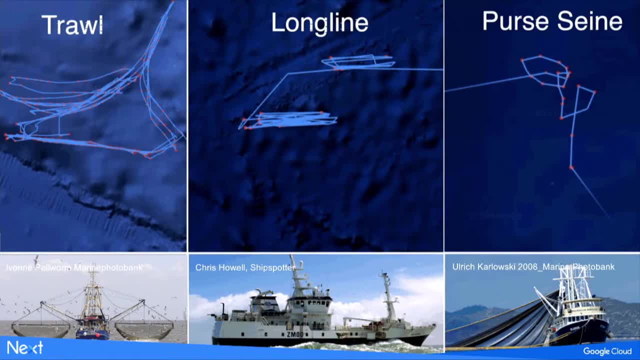 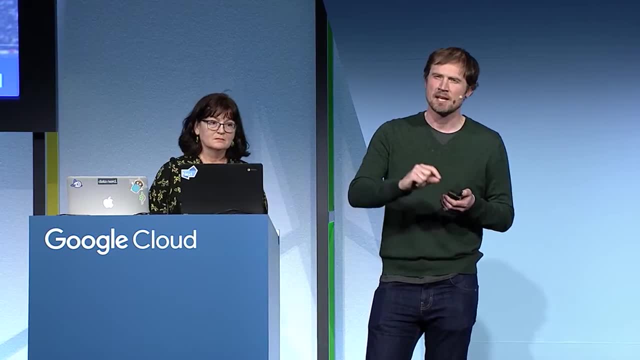 want to give you that information. And two, when you get it, usually it's not exactly right. For instance, the um, the, the latitude and longitude may be slightly off or the time stamp may be in the wrong time zone. 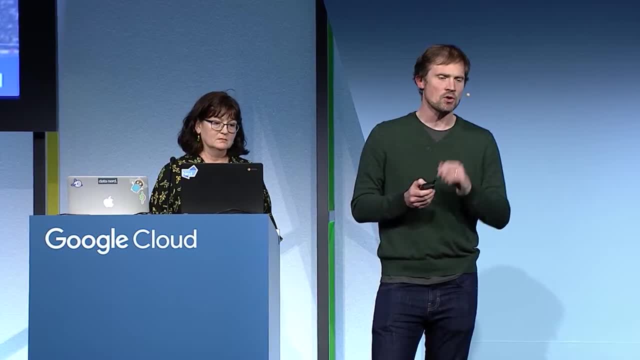 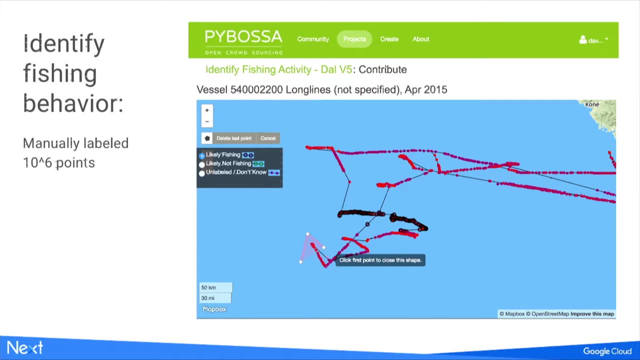 And so it's much easier, And sometimes more reliable, to just look at the tracks and hand-label where you think they are fishing. And so this is what we did, And this was very, very tedious. I built a small JavaScript interface through Pibasa, an open source platform for crowdsourcing. 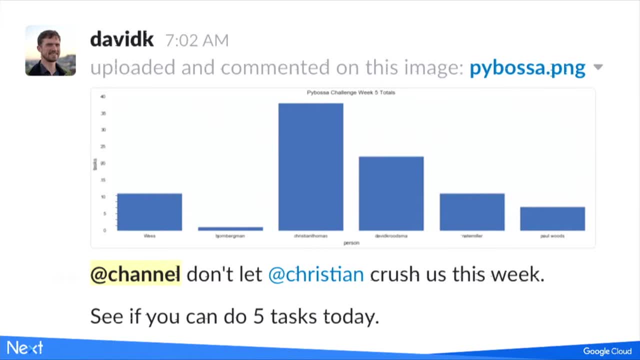 And then basically messaged everyone on Slack every day to tell them they had to do more tasks, And we made a little competition out of it. Don't let Christian crush us. He crushed us this week, And this went on for about six weeks- every day. 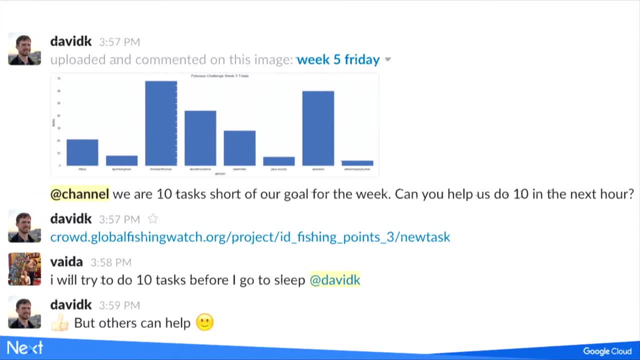 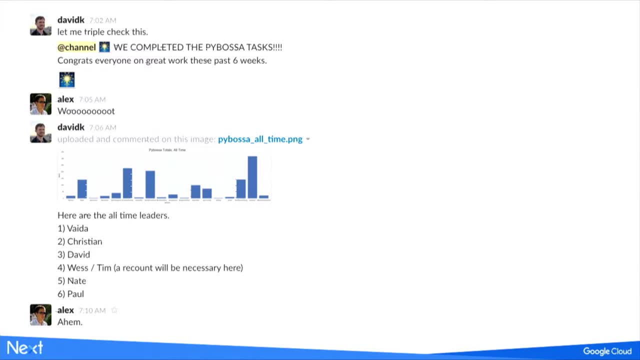 until we had labeled a few hundred thousand points. And this is one of the main things about this machine learning techniques- I've learned is that one of the major efforts is getting the training data and getting it in the right position before you can even do any of the fun model building. 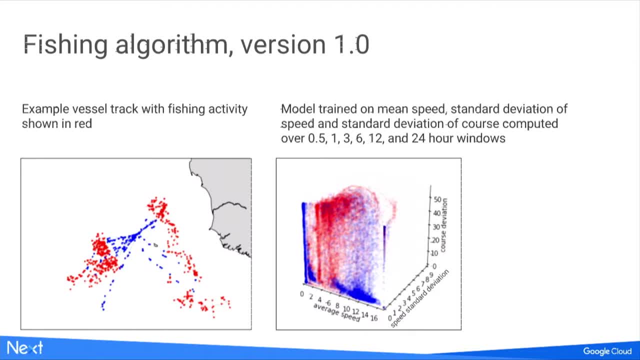 Our first algorithm on fishing was the simple logistic regression, trained on the average speed, the standard deviation of speed and the standard deviation of course, and as well as those features squared across a few different time windows. The whole idea is if a boat is moving slowly, wiggling, 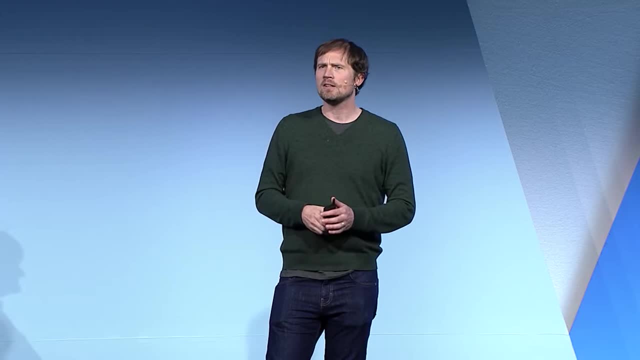 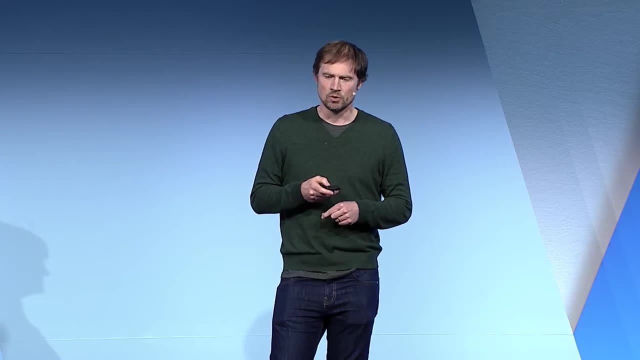 and changing direction. it's more likely fishing. And that model did relatively well in overall accuracy. I think just under 0.8.. But then we've decided we wanted to do both, for the idealization and for identifying specific vessels. 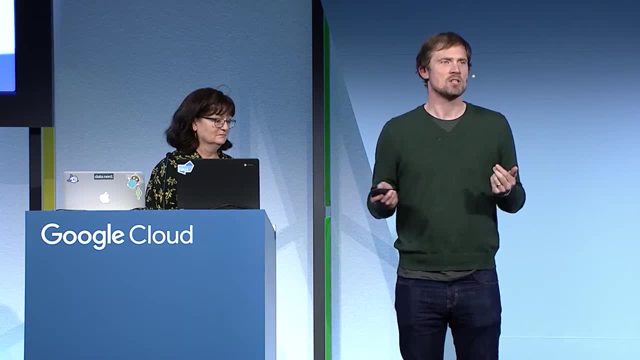 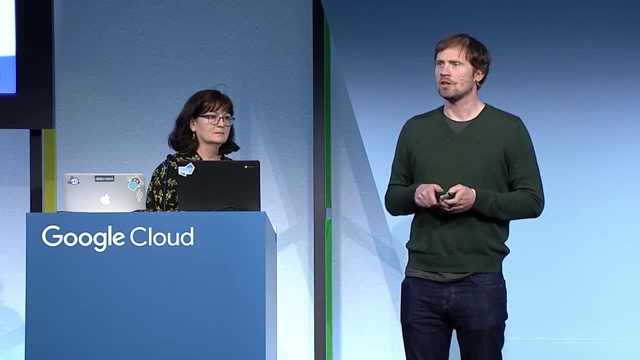 and for identifying this fishing effort. we wanted to build a neural network to do this, because we thought it could do a little bit better. And the problem with using a neural network is just the sheer number of points, So you can think about it each, you know. 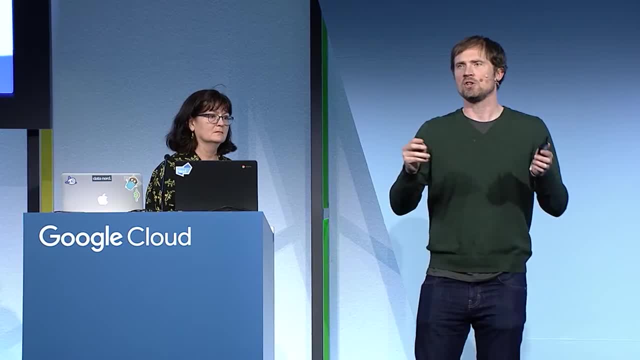 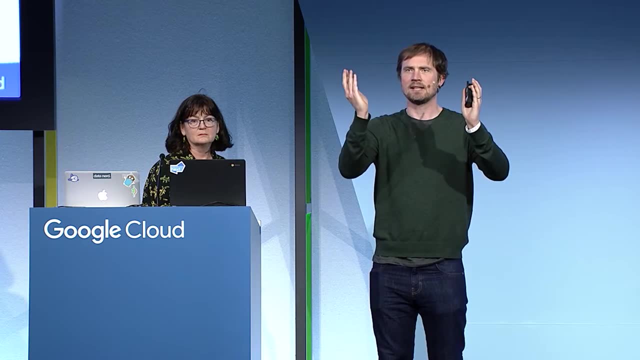 we want to take. we want to look at the whole path of a boat, And so you take maybe 10,000 data points of where it's been, And for each of those data points you have like 10 different features, such as the speed. 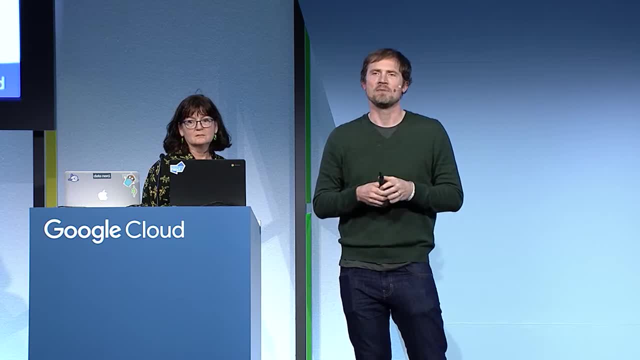 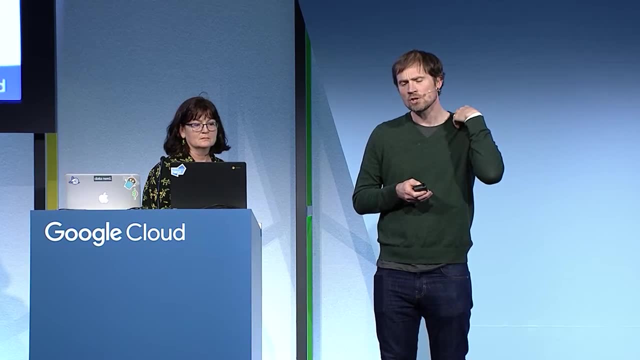 such as the course, such as the distance from shore, the time of day, And you want to use all that information to tell whether or not, what type of boat it is and whether it's fishing. So that's 10 features per point and 10,000 points. 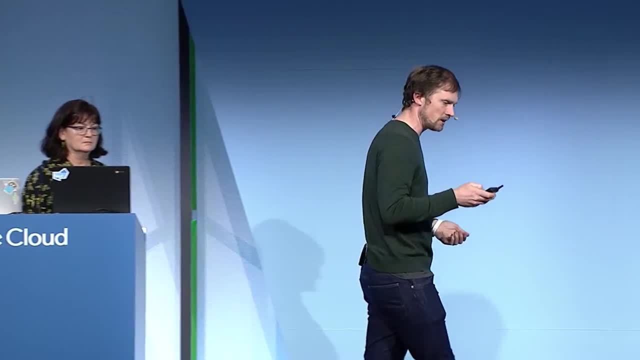 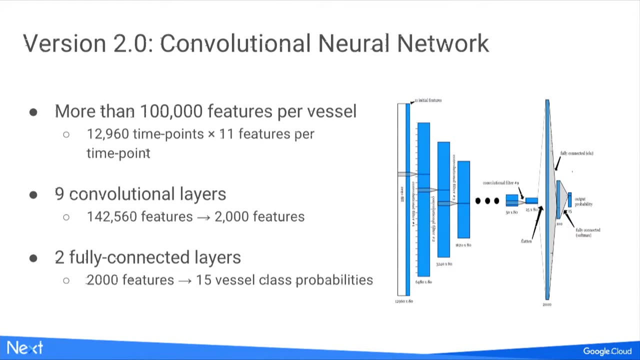 That's over 100,000 features Can't easily run a fully connected neural network on that. so we built a convolutional neural net that does a convolution in time, And what that does is we have nine of these convolutions and that takes more than 100 seconds. 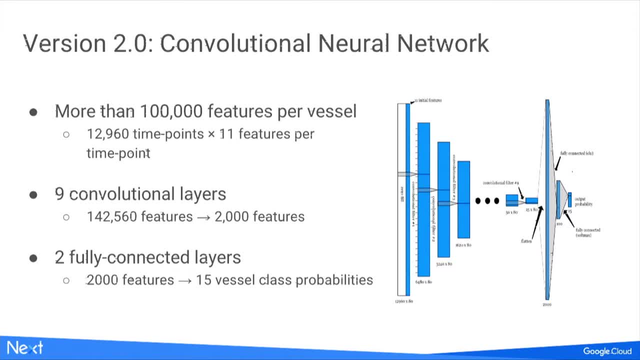 to get to 100,000 features and brings it down to around 2,000 features, And then after that we have two fully connected layers And that brings us down to a little over a dozen different vessel classes, And then we have a similar architecture. 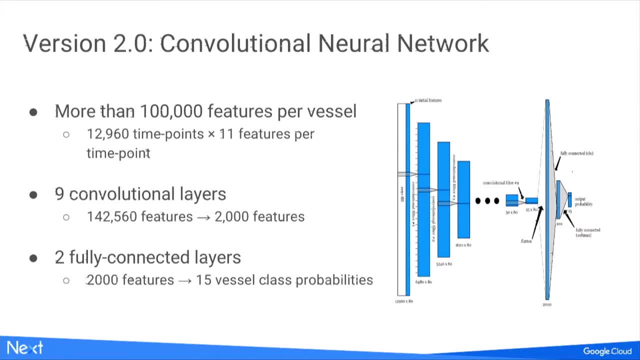 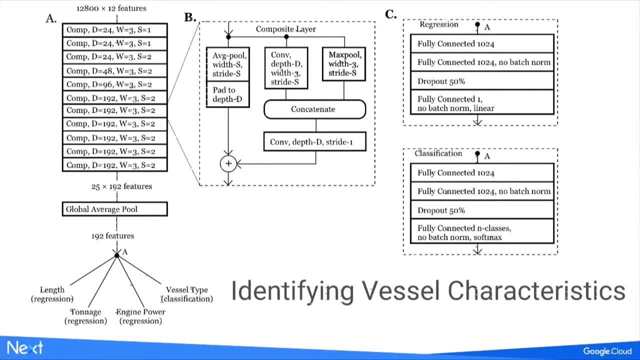 which figures out the looks at each point and identifies whether or not we think it is fishing. This is the detailed architecture of the identification model. We're also identifying the length and the engine power and the weight of these boats. Obviously, I'm not going to go over this. 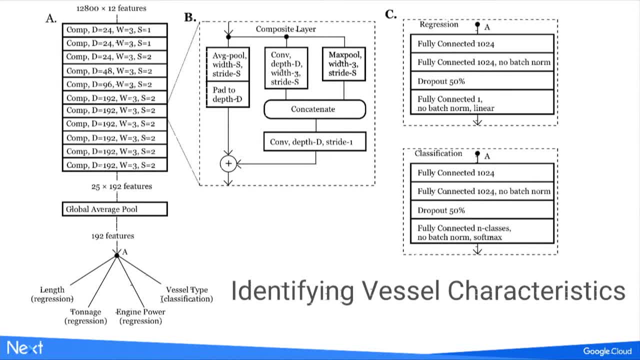 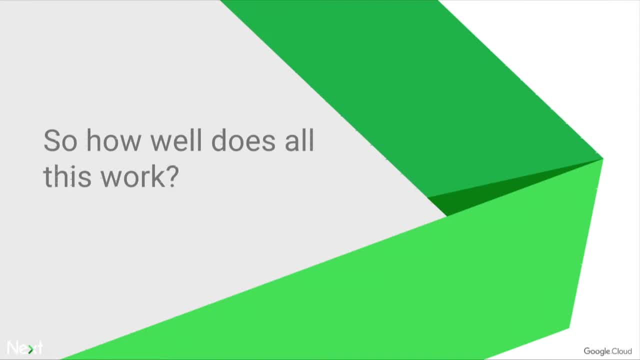 but we're working on a scientific paper to write up these findings And you'll be able to read much more about that in the supplemental materials of that paper. So how does it work? It works pretty well. Here's a confusion matrix of how the classification does. 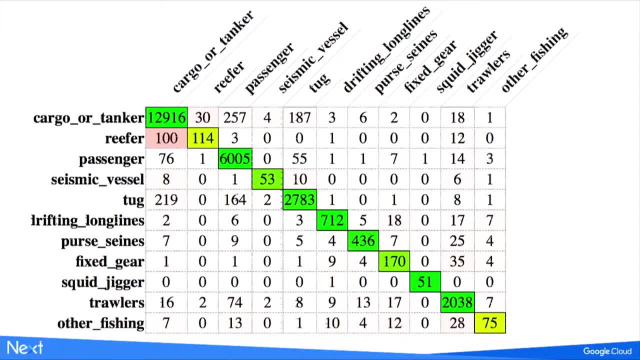 on our different classes, And so the top one. these are the different classes. The top one is cargo or tanker. A reefer is a type of cargo vessel for fishing, And so you can see it actually confuses it with something that you would expect it to, because they're 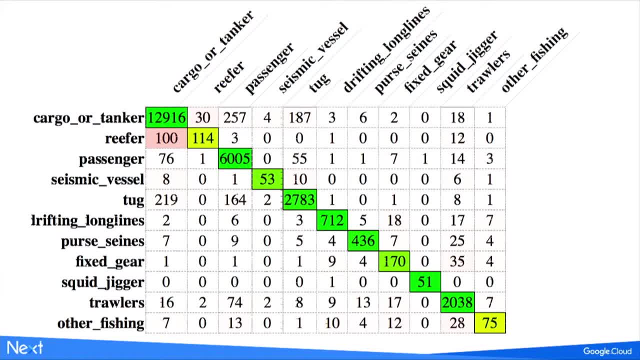 very similar types of boats, But for fishing boats which are all down on the bottom, it rarely confuses them with non-fishing boats, So we're pretty happy with this overall. And then the identifying fishing activity. it's a little bit better than the logistic model. 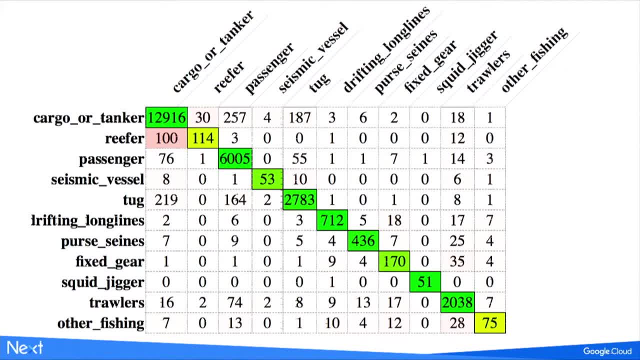 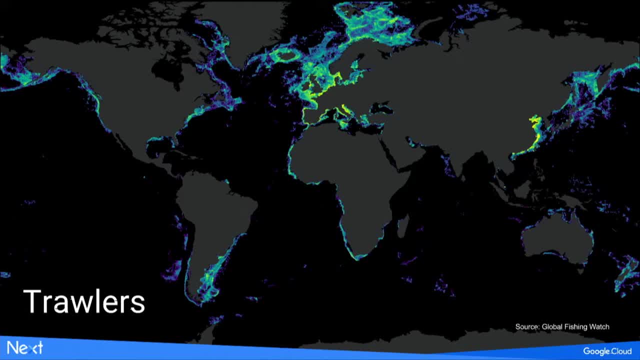 And we're making some adjustments to make it even better than that. So it performs better than the logistic, which is good, And then we can, for the first time, build maps like this, which is where we think trawlers are fishing in the world's. 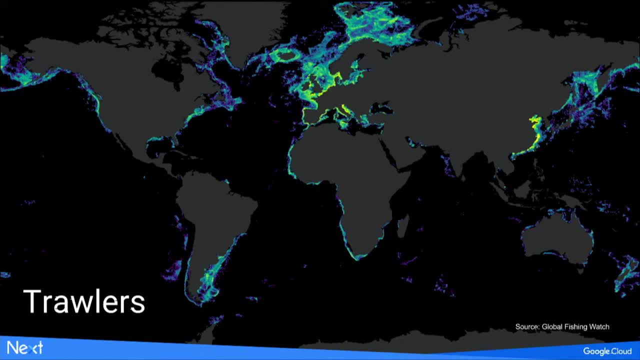 oceans And trawlers usually stay close to the coast because they drag their nets along the Bada ocean floor. So this is a map where we think all trawlers were fishing in 2016.. This is long liners. They set drifting long lines out in the ocean. 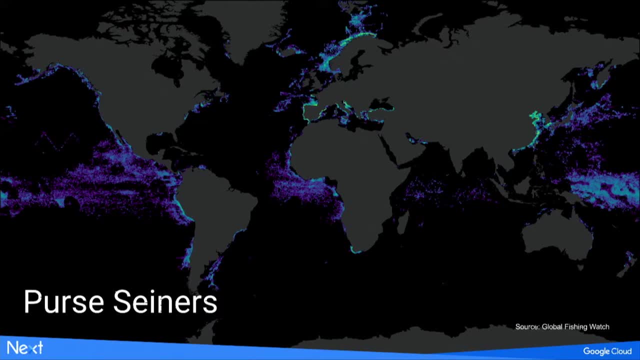 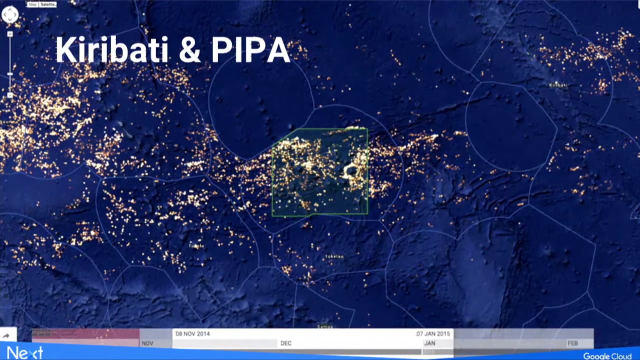 and so they cover all the oceans And then purse seiners which set these nets around schools of fish, often tuna, And you can see them fishing along the equator as well as off the coasts of some countries. Again, why does this matter? 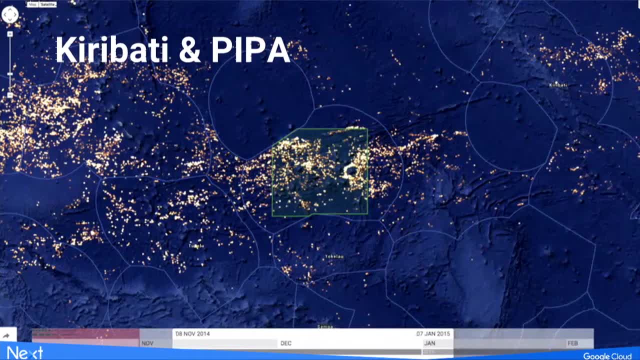 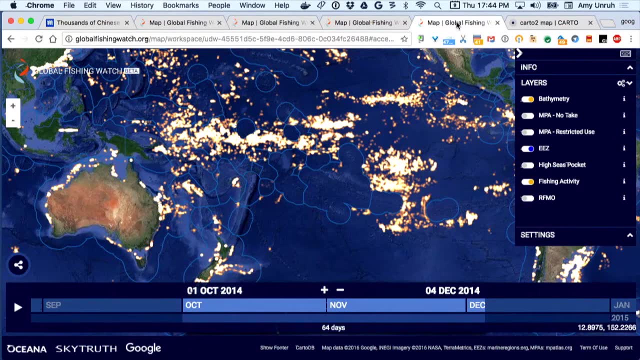 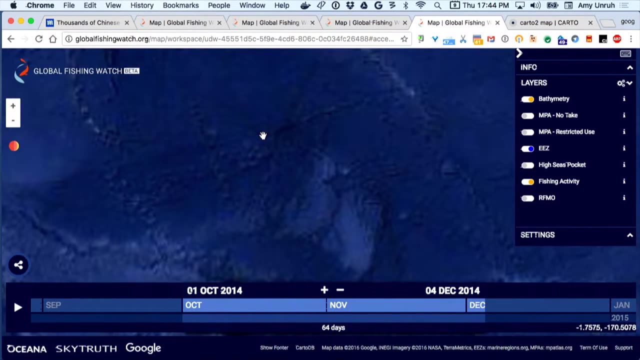 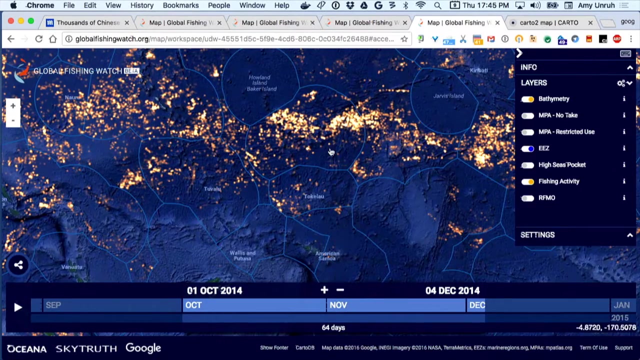 Why do we care about identifying where and when fishing happens? Well, here is a map of the Central Pacific and Global Fishing Watch, And I'm going to zoom into the country Kiribati halfway between. So the country Kiribati has the world's largest marine- UNESCO World. 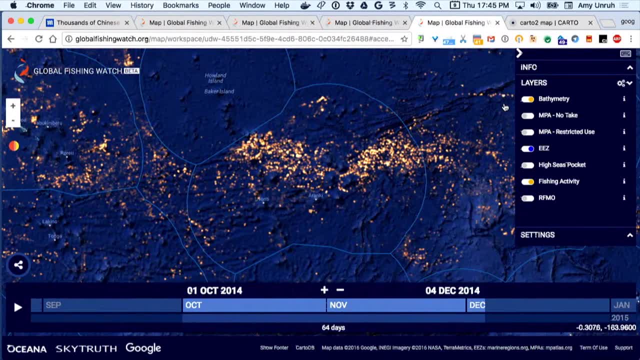 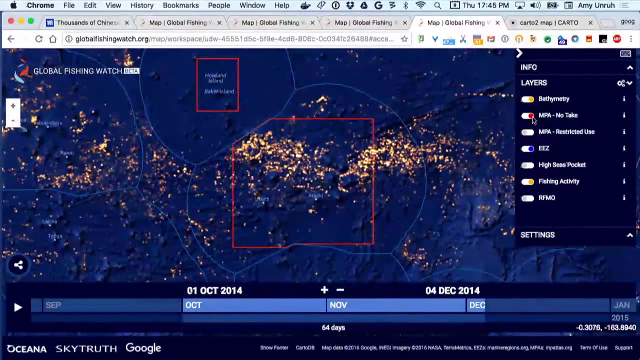 Heritage Site. Can you see it on this map? It is right there. So, even though it was a World Heritage Site- and this is from 2014,- even though it was a World Heritage Site, fishing- industrial fishing- was still allowed. 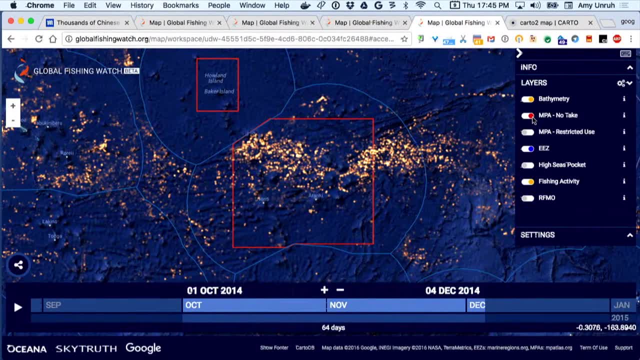 So you see lots of these yellow dots in it. However, on January 1, 2015,, the president of Kiribati decided to make industrial fishing illegal in this area- the Phoenix Islands Protected Area, or PIPA- And so all boats were going to have to clear out. 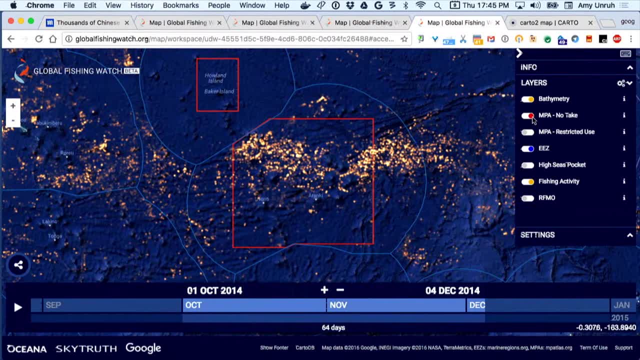 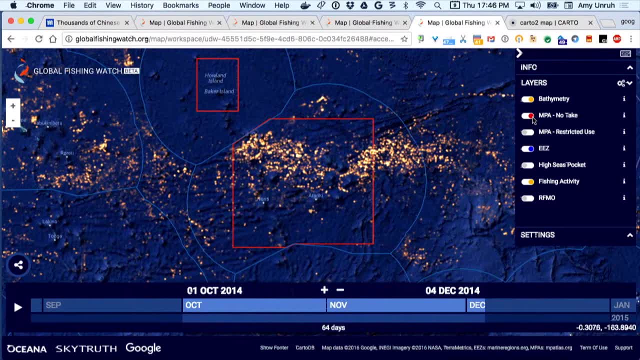 We're going to have to do it, We're going to have to do it, We're going to have to do it. So I am saying what's in the board. Well, I don't think we should emphasize This is the size of California, that red box. 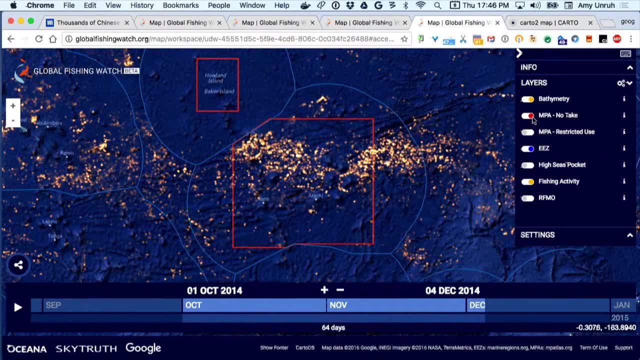 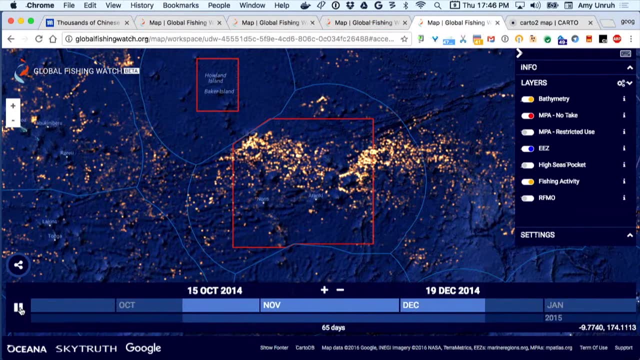 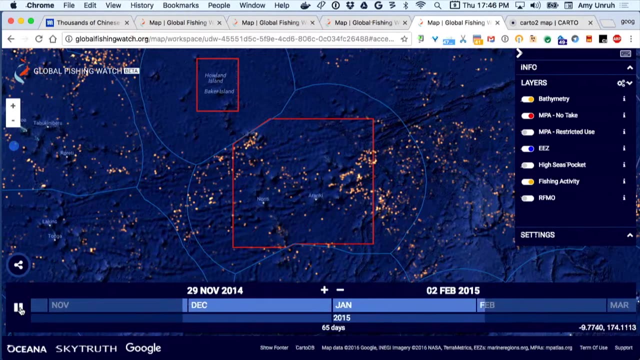 Kiribati is one of the world's poorest countries. They have one patrol boat for that entire thing, So I imagine you have to patrol California with one boat, And so what we did is kind of wait to see what happens. And now it's playing forward. 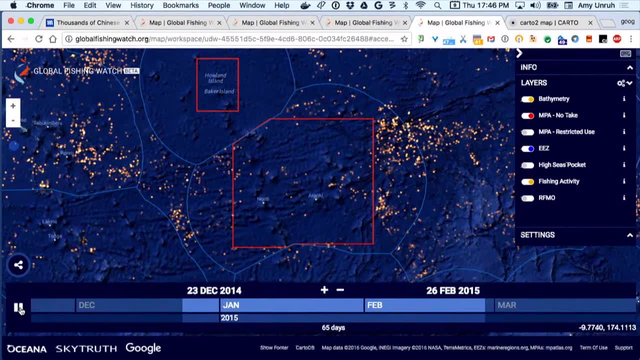 This is a two-month period time and now we're into 2015,. a little bit of 2014 still, And this would get into 2015 because there's new brefist here. all of it in 2015,. they clear out. 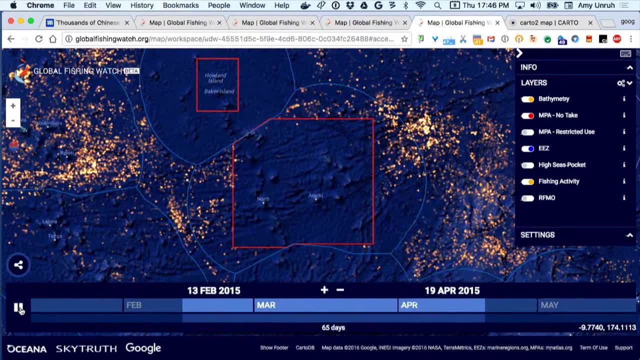 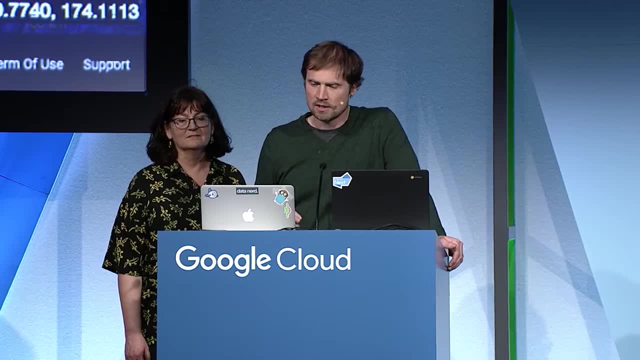 And we know the boats didn't just turn off their AIS, because we were able to track what happened to all those boats that left and saw that they actually went somewhere else and fished, And so it's really exciting that we're able to identify this park. 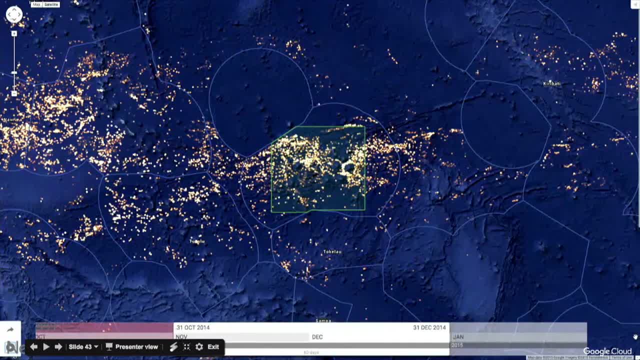 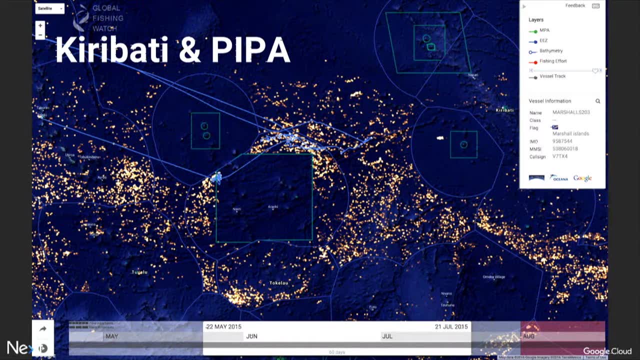 Now, in a few months after it closed, a boat- the Marshalls 203,, we saw fishing just right inside the line, right there, And the Kiribati authorities were notified and they went and their one boat escorted that fishing vessel back to port. 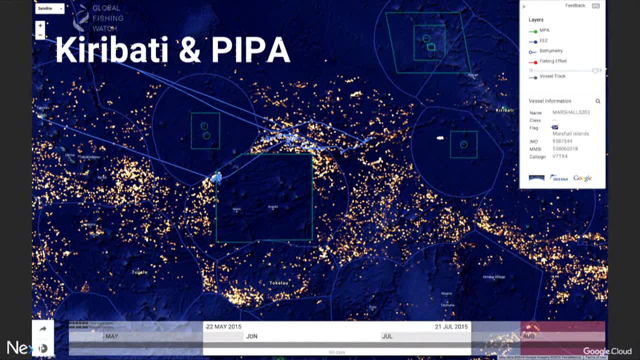 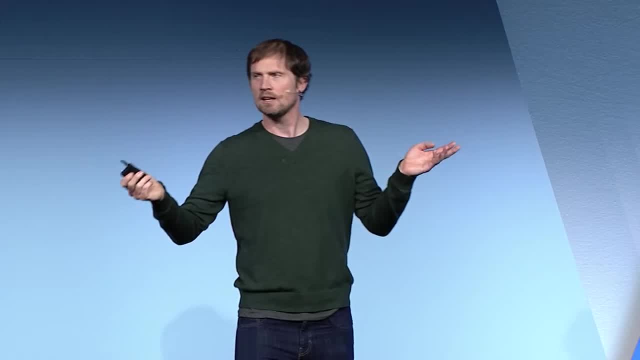 And they said the captain. they went to captain and said: you are fishing illegally. We want to fine you for doing this. And the captain said: you can't prove I was fishing. How do you know? I'll see you in court. 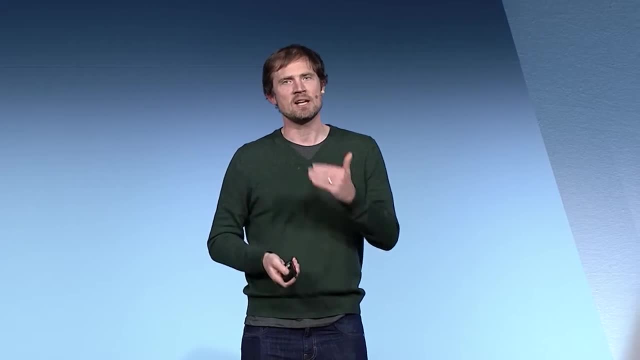 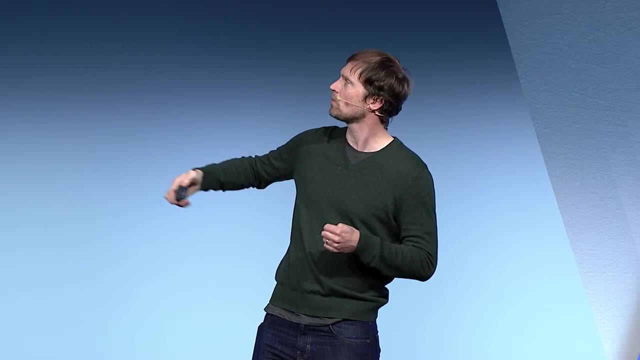 And so they actually called up Skytree within Global Fishing Watch and said: hey, can you guys look at this boat, see how it was moving, tell us whether it was fishing or not? And we sent them basically something like this with an analysis on it, as well as the results. 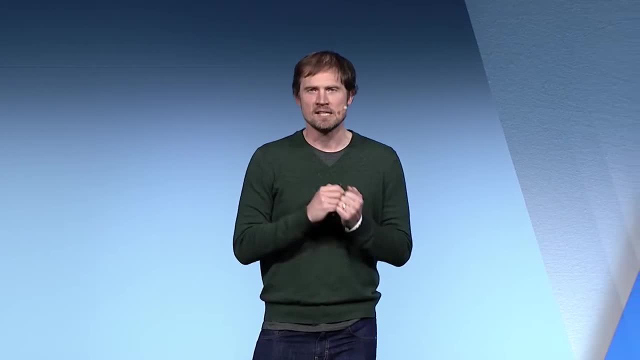 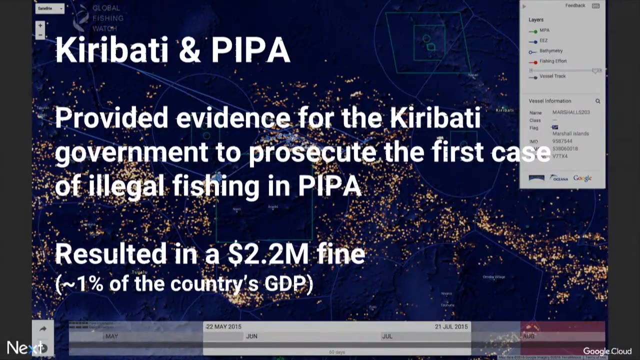 of our fishing algorithm. They showed that to the captain of the boat and he said: okay, I'll settle, And it resulted in a $2 million fine, which is about 1% of the country's GDP. And so it was. 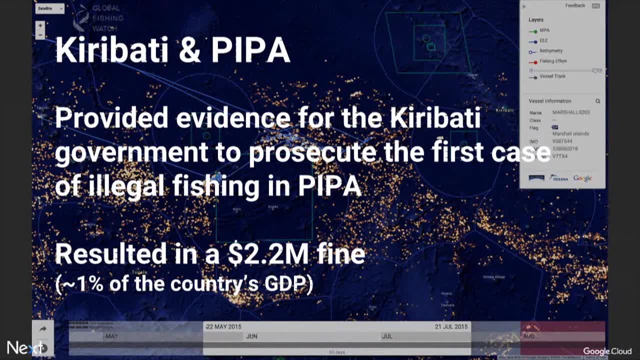 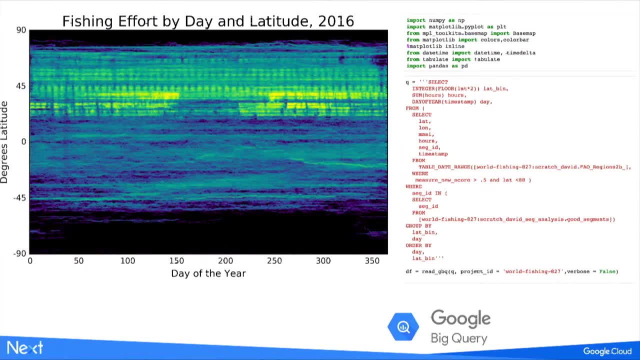 it was extremely yes, So I also enjoy a lot of data science work on this. So once we have this big data set- there's a lot of- we want to be able to look in all different types of way, but it's still several terabytes. 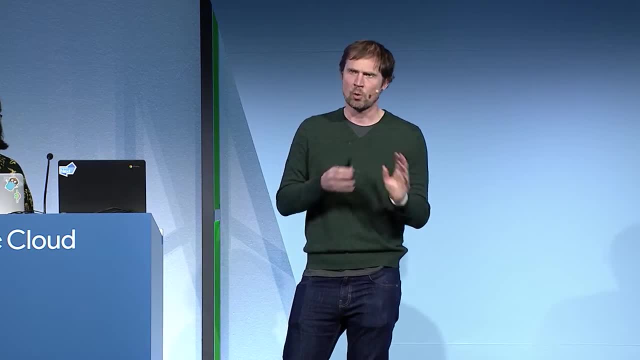 And so we load it into BigQuery and then use various tools to query in BigQuery, to slice in different ways, And this is an example. I do a lot of work like this. This is a IPython notebook. I run the write I wrote. 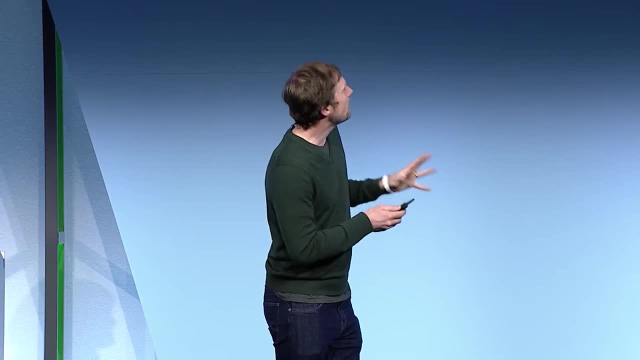 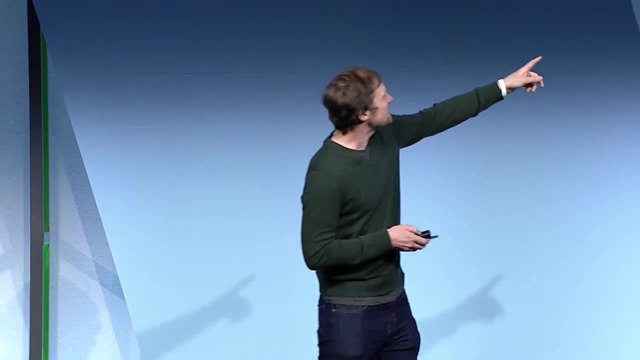 to write a query to make this graphic, which it's not impressionist art, It's not a. someone saw this and said congratulations, But what this is is the x-axis is the day of the year, The y-axis is degrees- latitude. 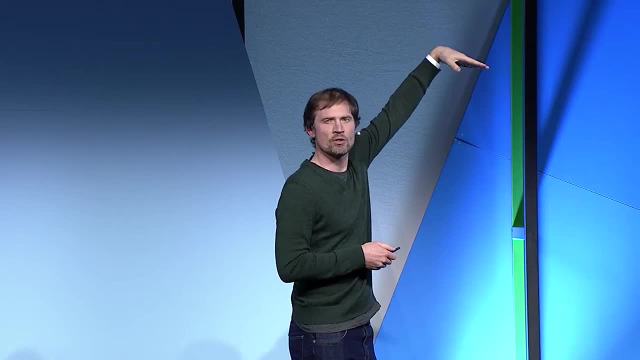 And so you can see when and where fishing is happening. You see, we have a lot more fishing in the Northern hemisphere. That's partially because of our data set. You can see people take the weekends off. That's what each of those stripes are. 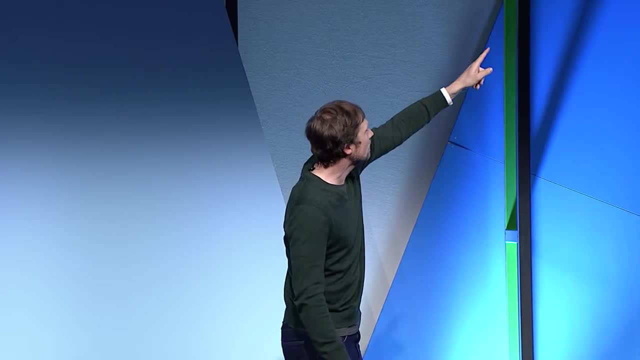 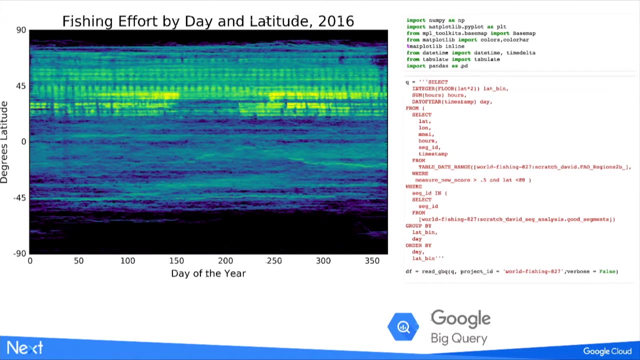 You can see that three month closure period. That's what we're telling you about in China. You see how that's right there. You can also see that China- actually people in China don't take the weekends off as much as in North America and Europe. 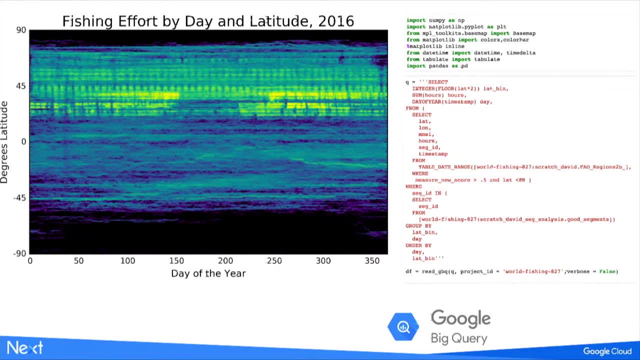 You can see other things. You can see that in Antarctica there's very little fishing and it happens only in the Antarctic summer. And what's exciting about this is, every time I look at this data I make a kind of a new discovery. 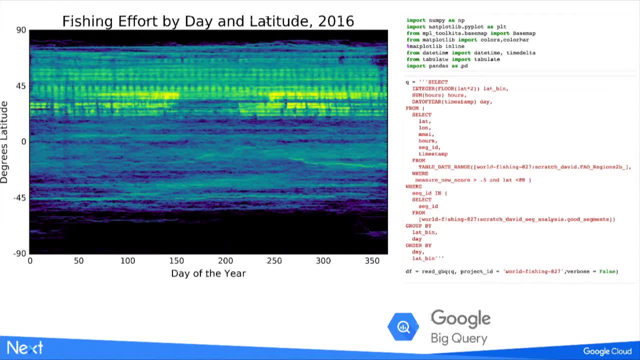 something no one's ever seen before, And it's only possible because we have these big data tools, like BigQuery, that allow us to quickly slice this data in different ways. We also are starting to use Earth Engine, which is a Google platform that allows you. 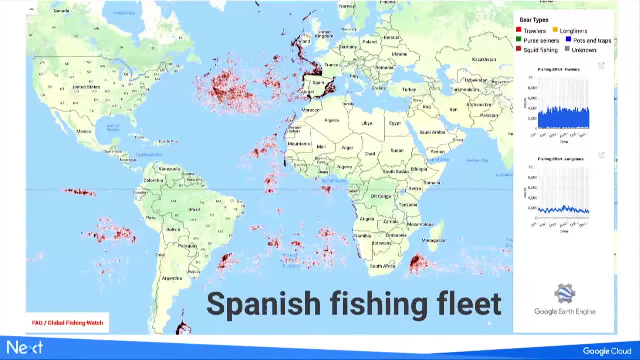 to do calculations on very large rosters, And so we can actually make our data, turn it into a raster and load into Earth Engine and then look at how it compares to various like climatological or other types of global data sets, And this just shows where all the vessels 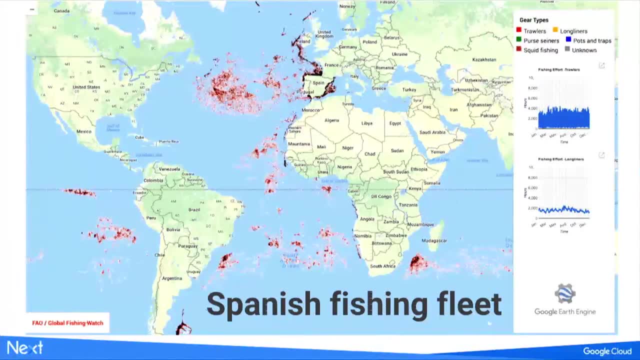 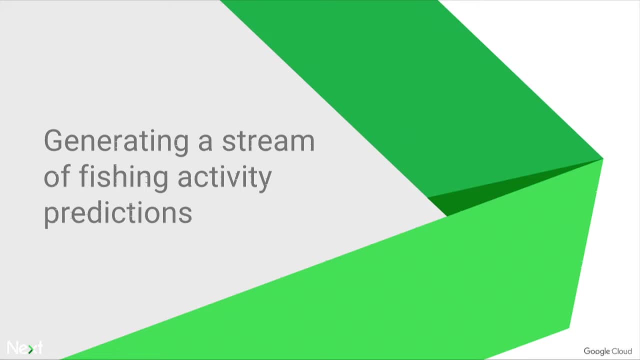 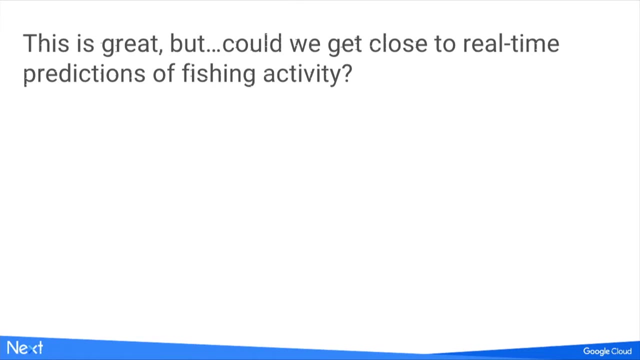 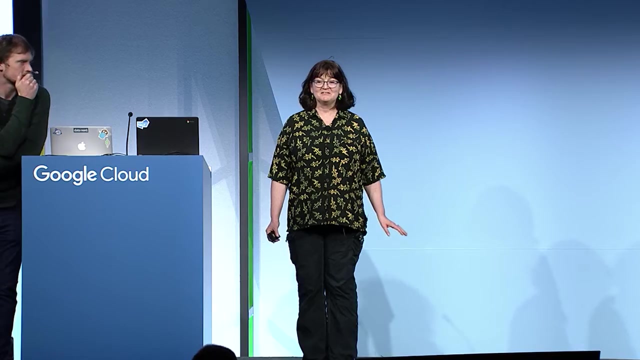 are coming from. This is from Spain fish, And actually it's quite remarkable if you look at how much Spain is fishing all over the world's oceans. Okay, so this is where I came into the story, So I wanted to see. this is obviously very, very cool stuff. 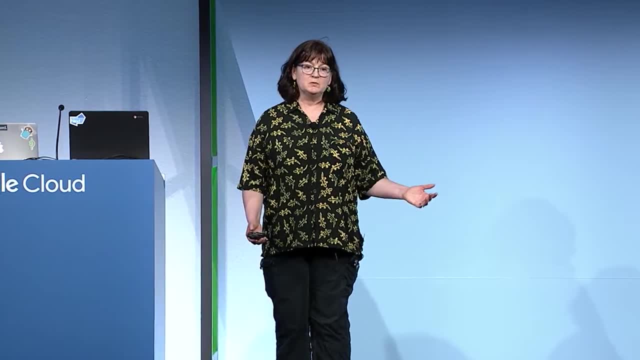 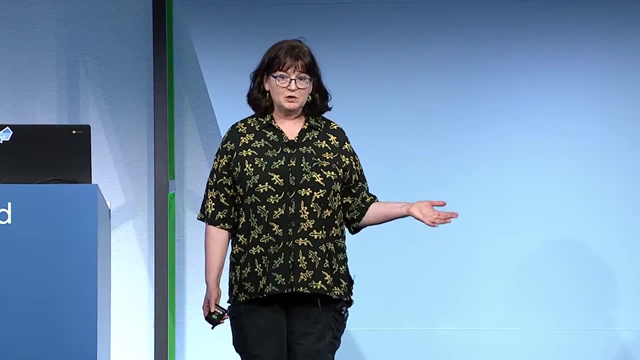 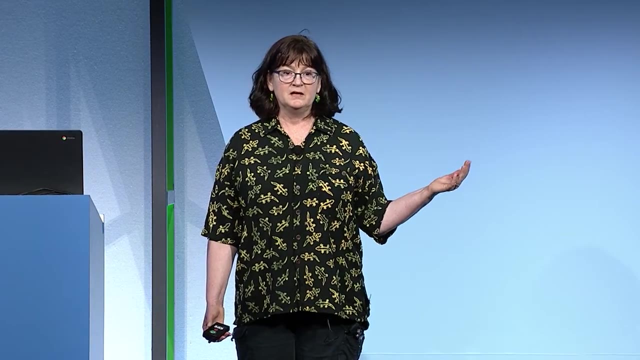 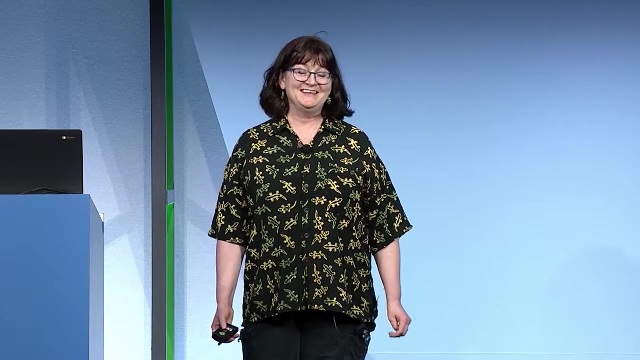 So I wanted to see what would it take to basically build on top of this, to see if we could generate close to real-time predictions of fishing activity, as all this data gets dumped into cloud storage every day. So it turns out that the answer is yes. 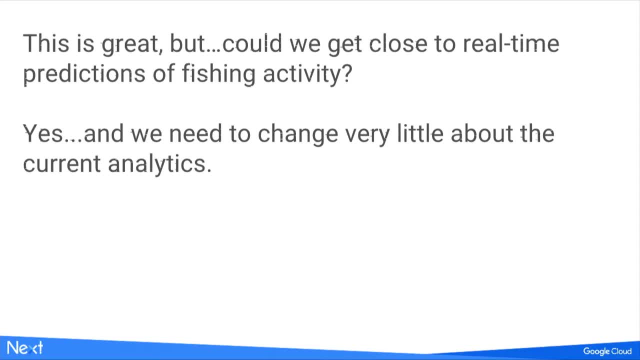 And it was pretty straightforward And I was able to do what I'm gonna talk about in just a few weeks. And I was able to do what I'm gonna talk about in just a few weeks. And I was able to do what I'm gonna talk about in just a few weeks. 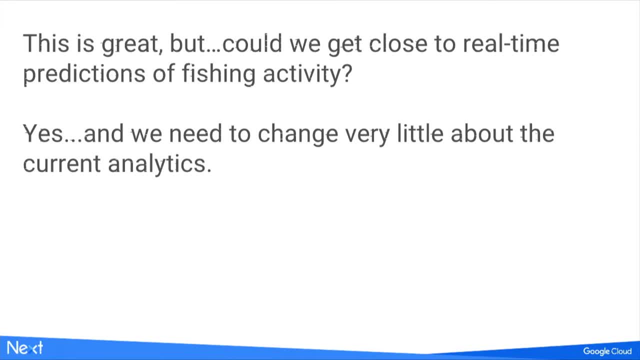 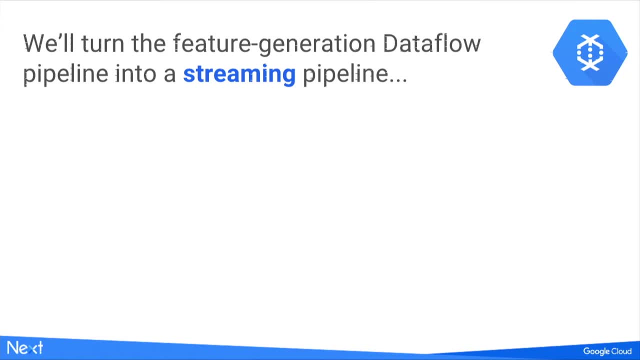 And very little needed to be changed in terms of how I hooked into what they had already built, And so primary reason for that is that it is very straightforward to take the data flow pipeline that we talked about earlier that Global Fishing Watch has been running in batch. 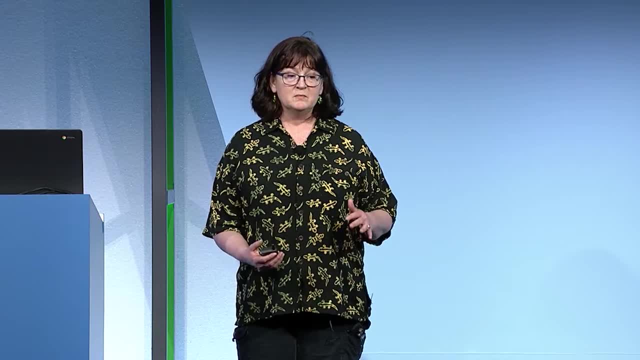 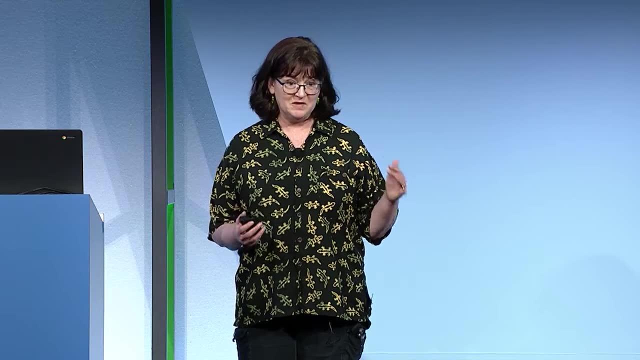 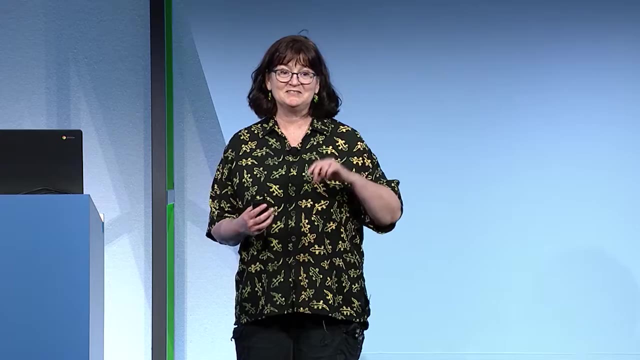 using to generate feature data, Because BEAM has this. Because BEAM has this unified streaming batch model, It's very straightforward to turn this into a streaming pipeline, And so essentially all I had to do was to change the so-called sources and sinks. 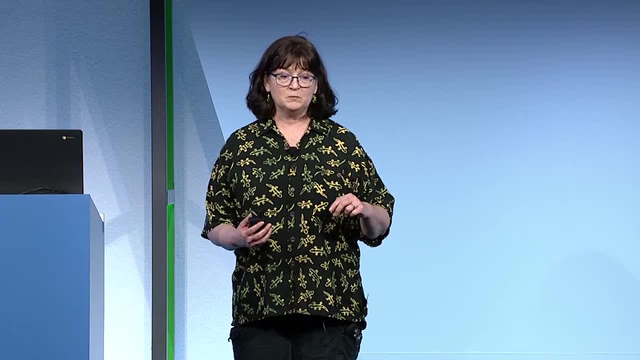 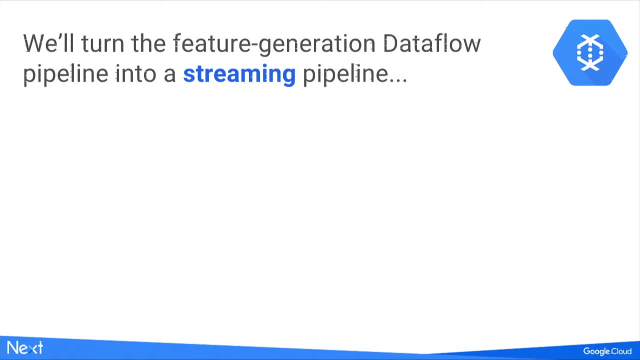 the inputs and outputs of the pipeline. So I did some work to stream data into the pipeline with using PubSub and then the PubSub. the pipeline was also modified to emit data to another PubSub topic. So streaming in, streaming out, But the logic of the pipeline could stay the same. 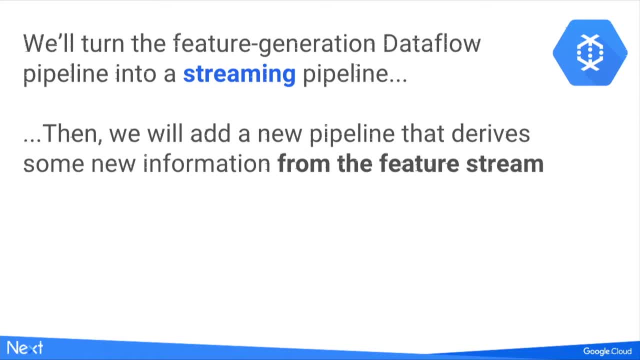 And so that was really nice, it was really straightforward. And then I added a new pipeline that consumed that output stream and did some further derivations of using the derived features and using CloudML Engine and the trained TensorFlow model to make predictions about where phishing activity was happening. 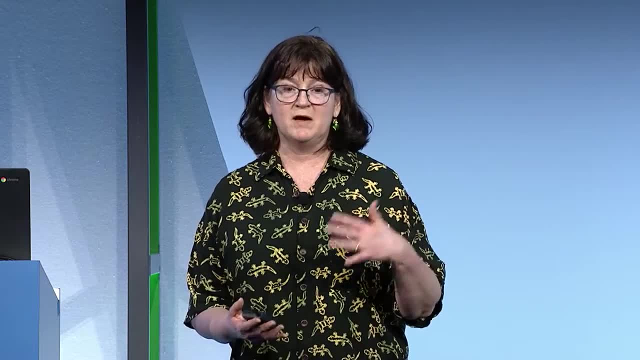 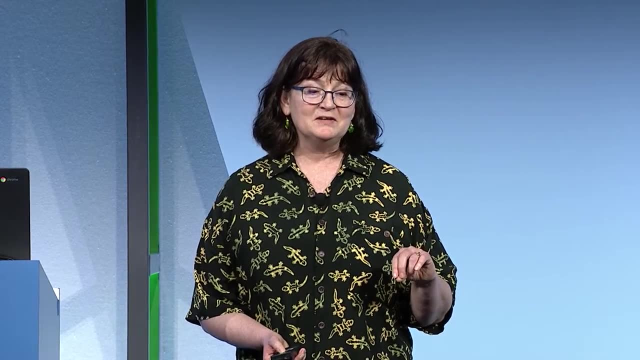 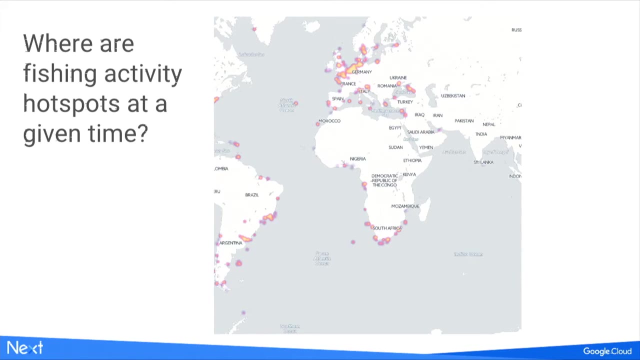 So this was the second of the two models that David was talking about, the model that predicts phishing activity. Okay, so what the second pipeline does is basically surface in near real time Where are the phishing activity hotspots at a given time. So let me show you what kind of the results of that. 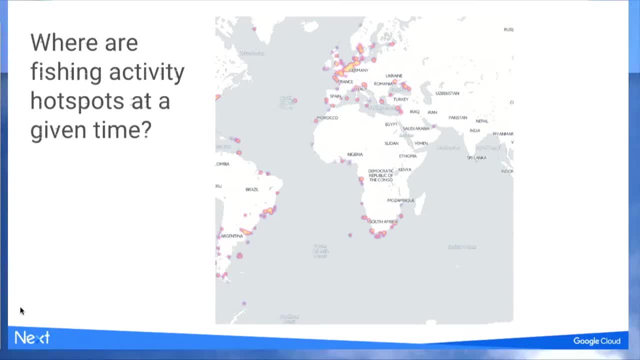 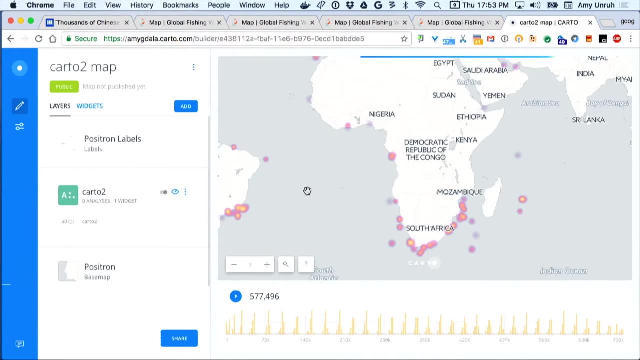 and then I'll dig into the tech that made it work. Okay, so this is being displayed on Cardo, a cool site. This is data from real data from a couple of weeks ago, And when I hit play, what it's gonna show is basically over the course. 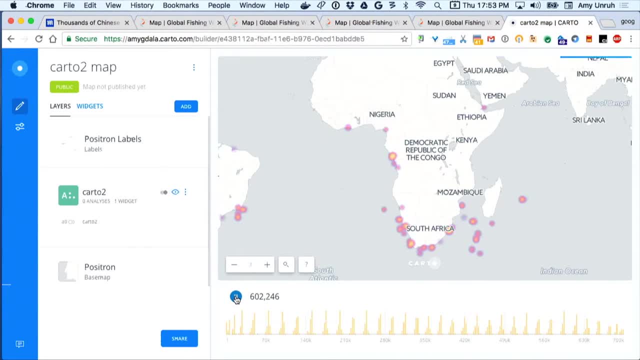 of about 10 days. what phishing activity hotspots did we find? So the heat maps are just showing magnitude of phishing in the area. you know might have been more than one boat And over time you can see those shift around. 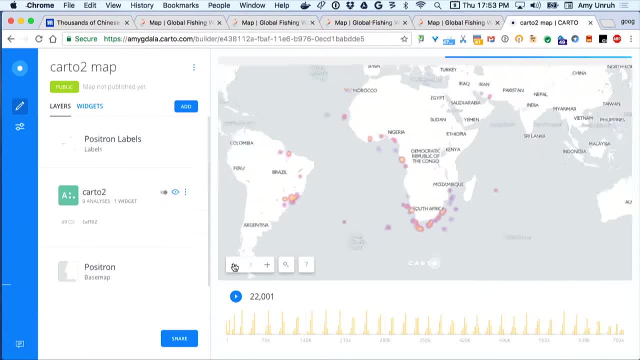 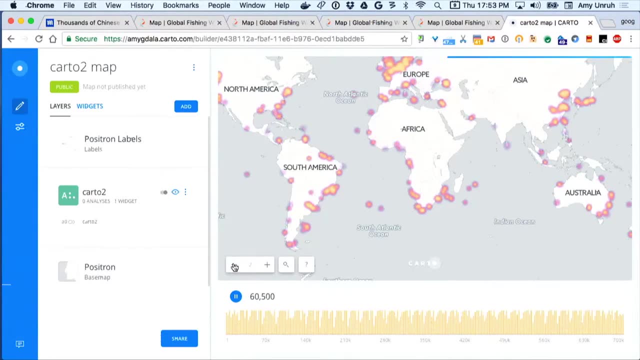 And it's even a little more dramatic if I, if I zoom out a bit here. Okay, so you can think of this as being in near real time. as the data comes in, we're saying, all right, there's phishing activity here. 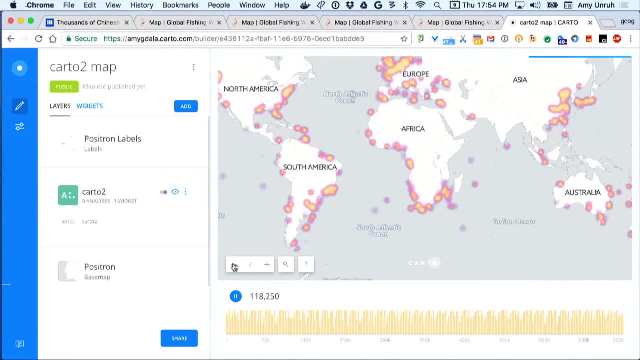 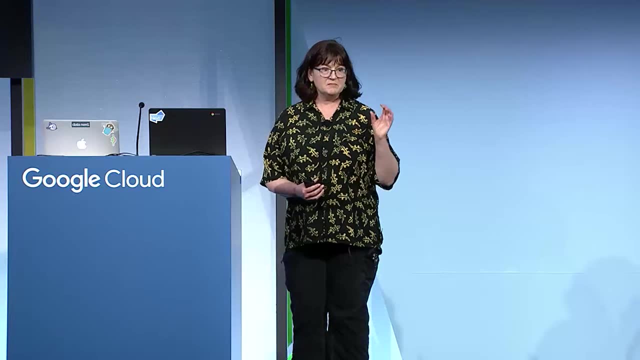 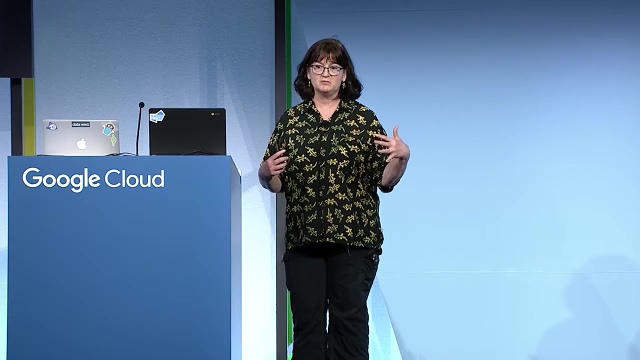 there's phishing activity here at a given point in time and then we kind of have a sliding time window and so that can help Global Phishing Watch give them early indication if phishing is happening where it shouldn't or if there's things they wanna focus on in their larger batch analytics. 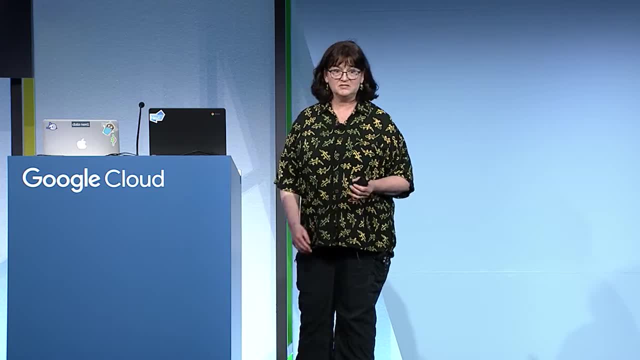 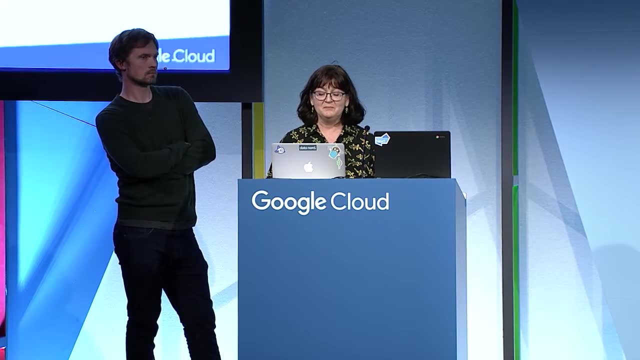 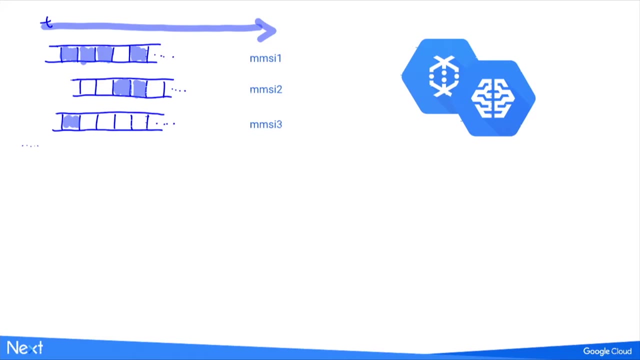 that doesn't look quite right in terms of where people should be phishing at a given time of year. Okay, so now let's look at what went into that under the hood. So here's the- just kind of at a high level, the logic of the second pipeline that I built. 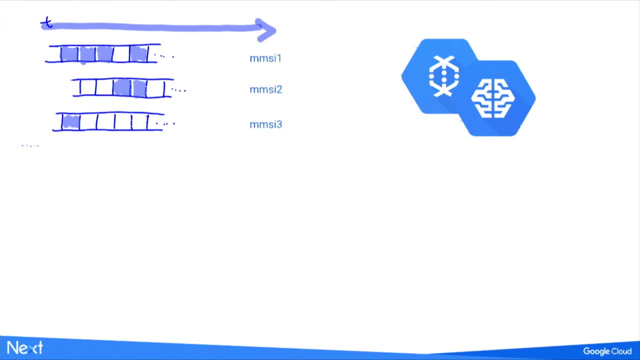 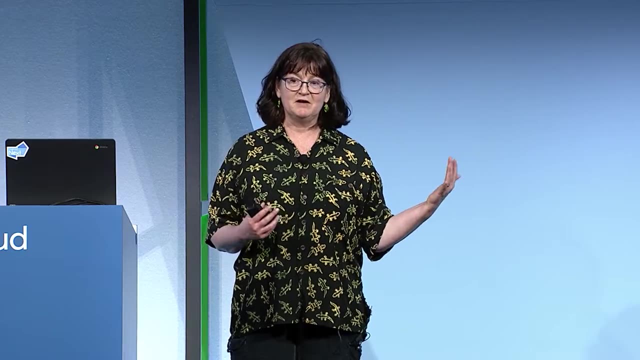 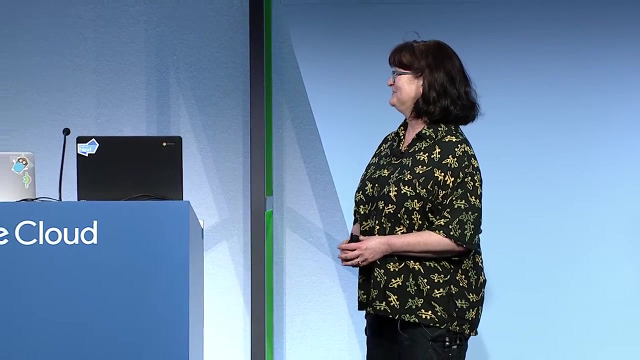 So as input are these derived features from the first original Global Phishing Watch pipeline and again using features in the sense of input to their machine learning model. And David, remind me what is MMSI? Marine Mobile Security Number Identifier. 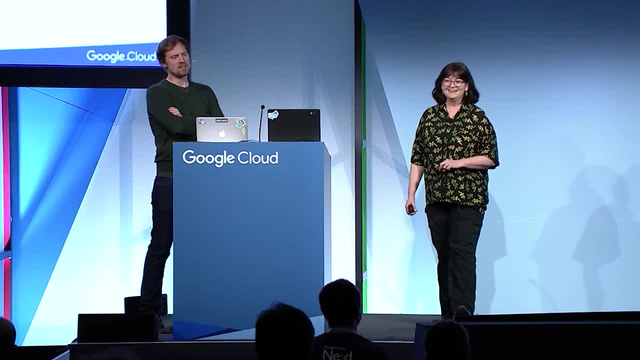 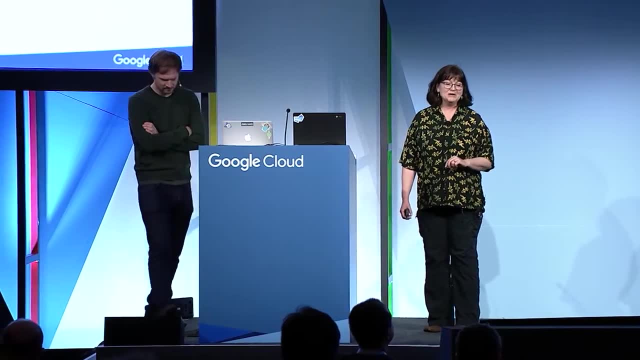 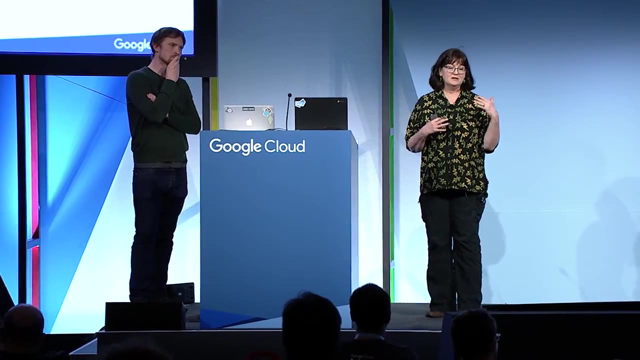 Yes, It's a yeah Each Given out by the International Telecommunications Union to boats. There you have it. It's a little quiz. So each such identification which corresponds to a ship, a stream of features is being generated for that ship. 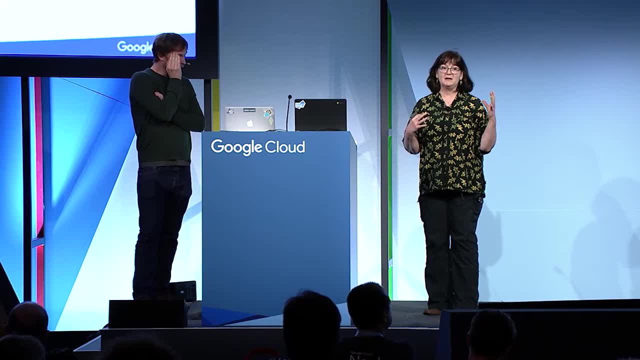 And so this new data flow pipeline first aggregates those for each ship into a sequence that's of sufficient length to send to the trained machine learning model, And it responds with, with indications suggested by the blue colored cells here, of where it thinks phishing activity. 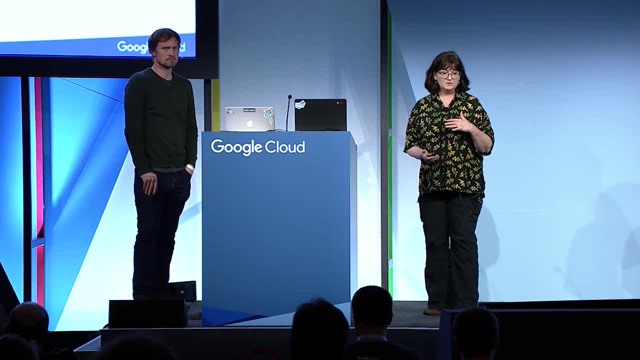 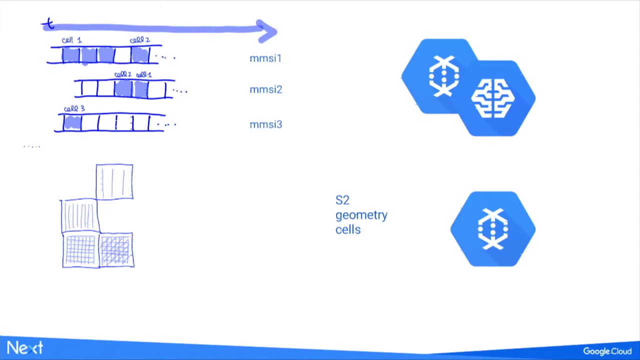 where is happening in that sequence. So we know the time where it thought phishing was happening, We know the location. So then, and we used the learned TensorFlow model and CloudML to do that. So then the next stage of this data flow pipeline. 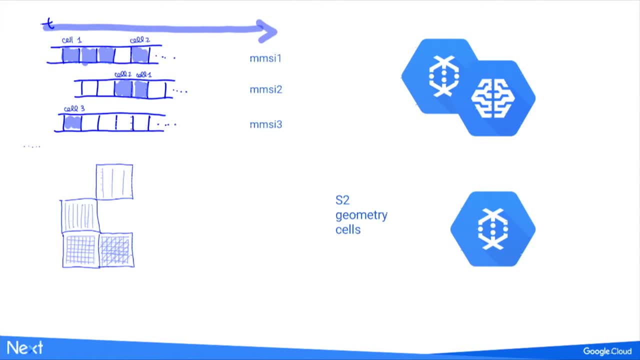 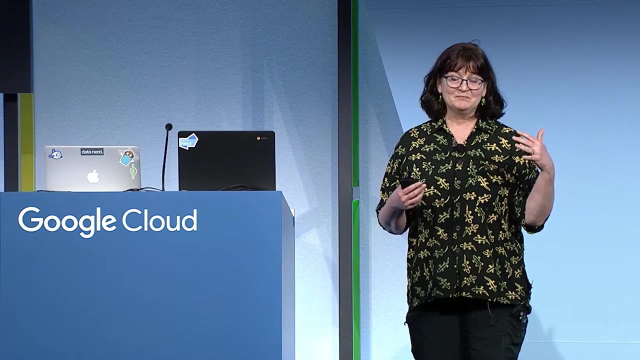 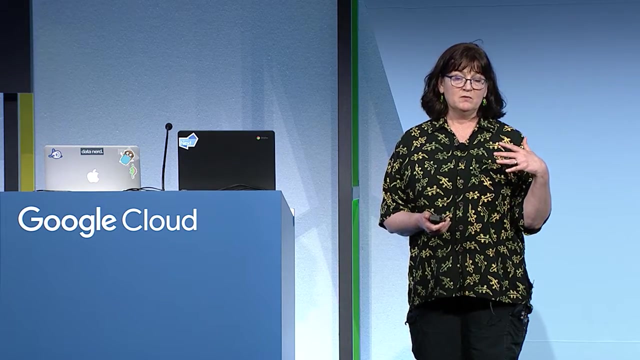 groups this information by by geographic region. So I'm using a representation called S2 geometry to group the detected fishing, predicted phishing activity into basically like one kilometer square areas, And so by doing that we get an indication of like what's the magnitude. 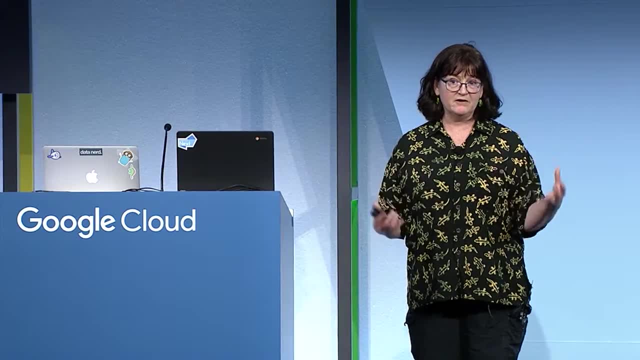 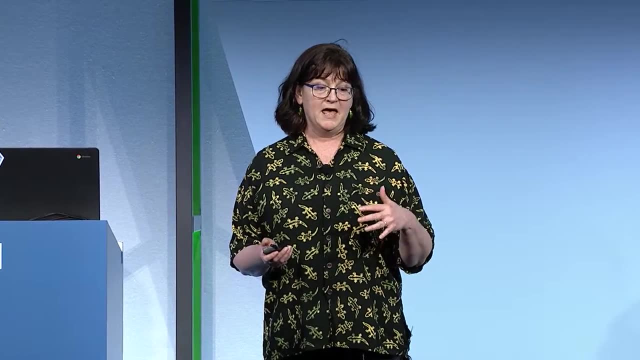 Might be more than one boat. What's the magnitude of fishing in a given area at a given point in time? And then of course we want to analyze this over time And of course the the magnitude might change over time for a given square. 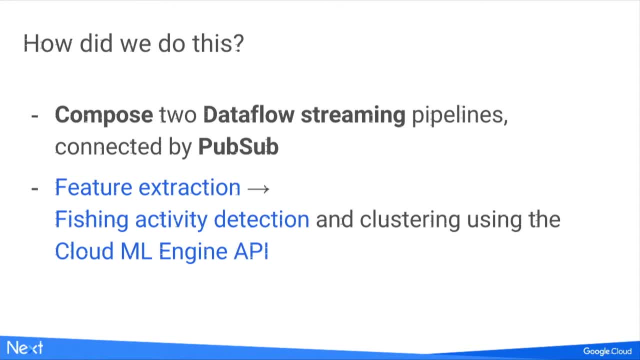 Okay. so to do this, start to look at the nuts and bolts a little bit. The first thing we did was compose the two Dataflow streaming pipelines, connecting them by PubSub. So the first original feature extraction pipeline and then this new pipeline to use CloudML Engine. 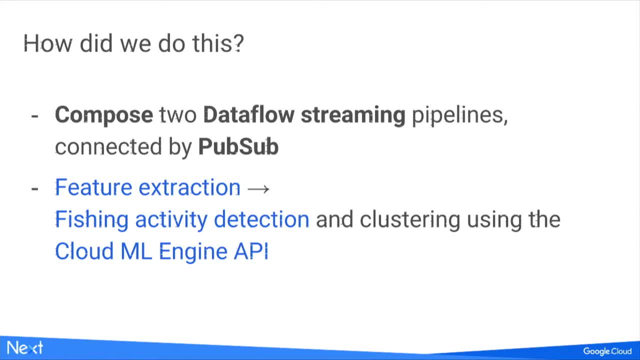 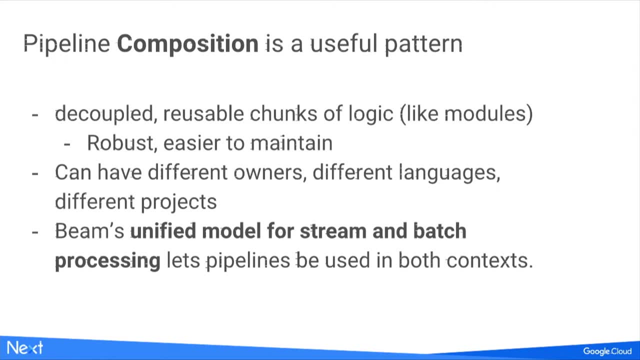 to do prediction of phishing activity and then to do basically location-based clustering. So this is a really useful pattern And you can kind of think of Dataflow pipelines as like decomposable chunks of logic, kind of like modules and actually almost kind of reminiscent. 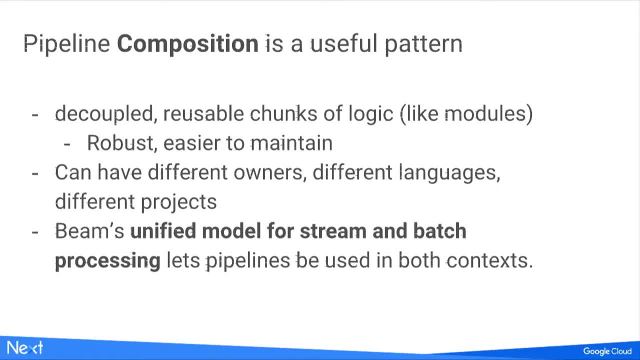 in how you hook them together, of Unix pipes as well, So you can compose them together. You just need to connect their inputs and outputs essentially, and the Dataflow pipelines can have different owners, They can even be in different projects, They can be written in different languages. 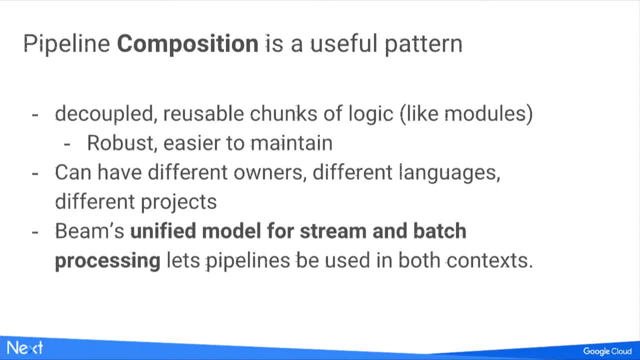 and that was actually the case here. The original pipeline was written in Scala, and the one I built was written in Java, And then the means of connection is PubSub. So something to keep in mind, then, is that Apache Beam's unified model for doing both stream and batch processing. 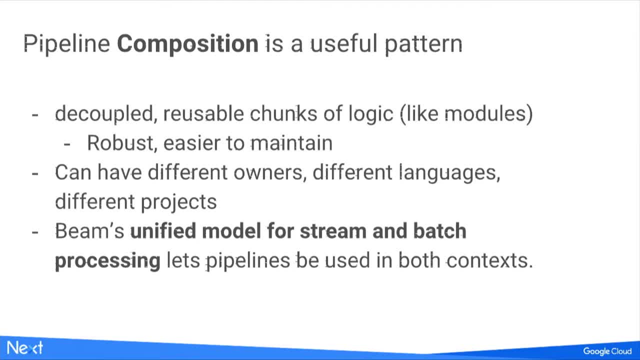 lets you use these pipelines that you build into different contexts, like the device or a virtual model. So you want to be able to use both of these pipelines that you build in different contexts. Do you want to hook them together in stream mode? 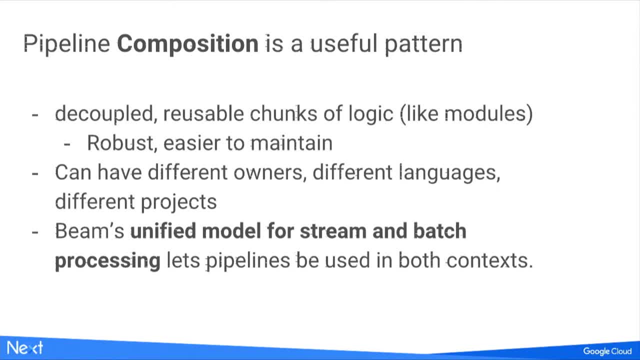 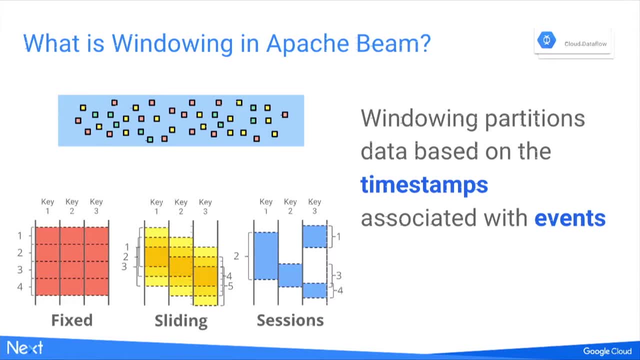 Do you want to use them in batch mode? You can use essentially the same pipeline for both, Okay. so another key thing that we leveraged to do this is Apache Beam's windowing model. So if you think of, if you think of, you've got an unbounded 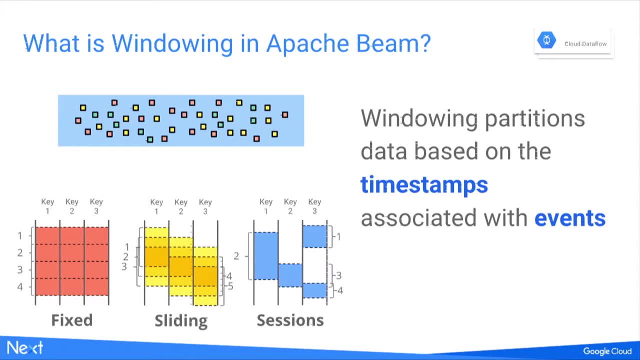 essentially infinite stream of data coming in and say you want to, and say it's colored tiles, kind of like what's suggested up top there, and say you want to group them by color. so you want to group all the green tiles together. 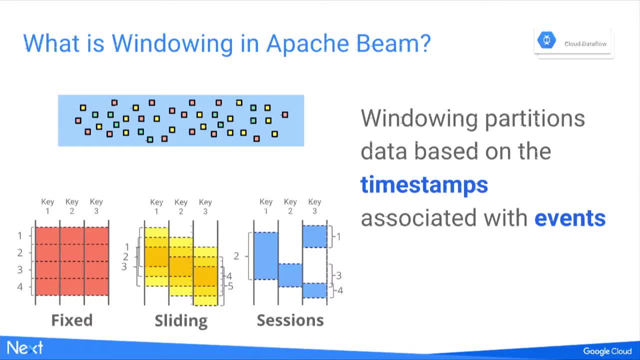 and count them. you want to group all the old tiles together and count them. you need to do that in the context of some defined window, or else it's ill-defined. it's an ill-defined problem. So Apache Beam has really sophisticated and flexible windowing model. 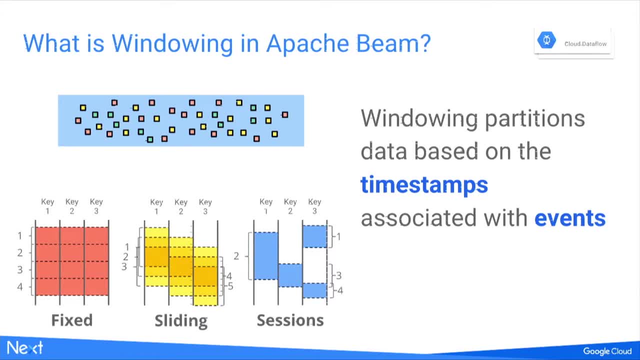 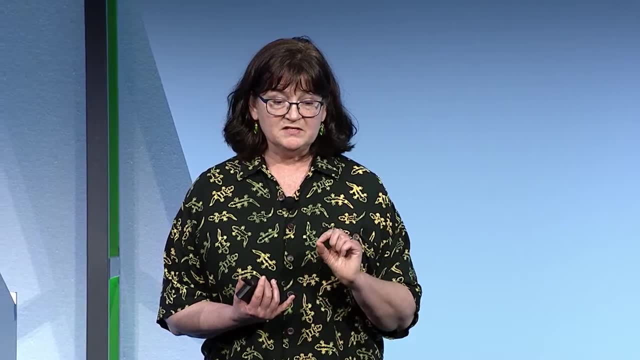 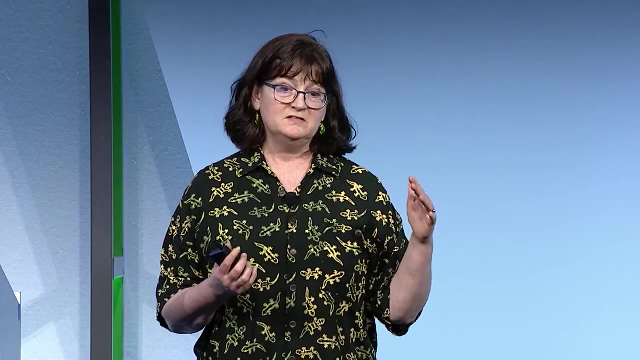 It has different kinds of windows. For the second Dataflow pipeline I built, I used sliding windows And I mentioned this earlier. it does something that's really powerful. It lets you say: do you want to window by data arrival time into the pipeline? 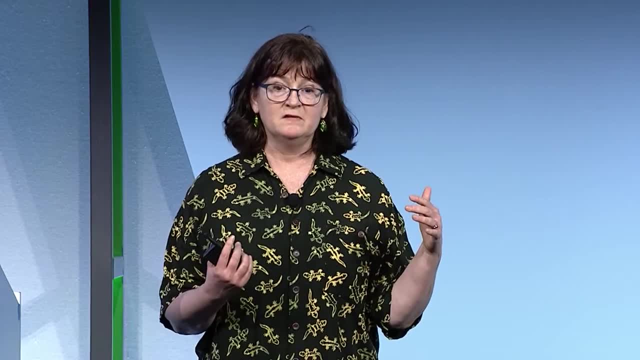 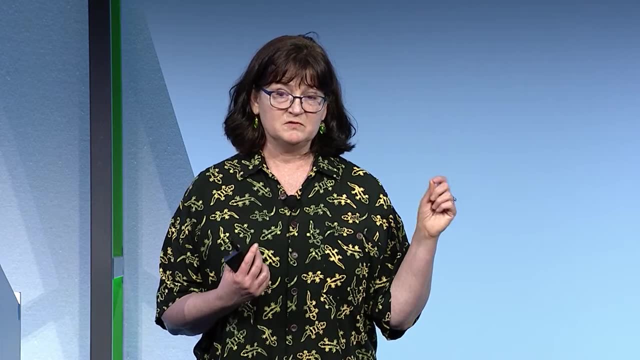 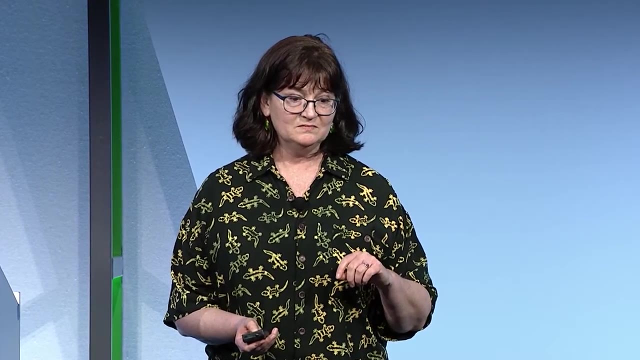 or do you want to window by? do your analysis with respect to when the data was actually generated? And so we were doing it with respect to when the data was actually generated, when the ship actually emitted that bit of information to the satellite. Otherwise we wouldn't get good results, of course. 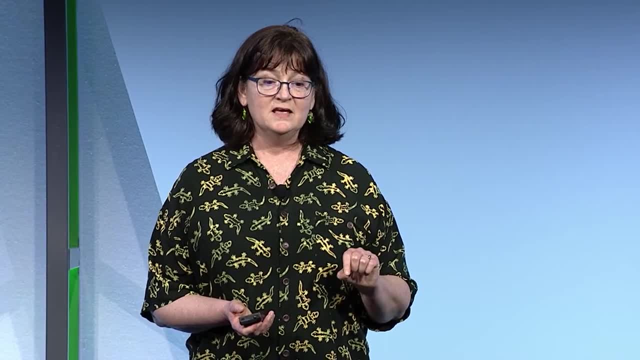 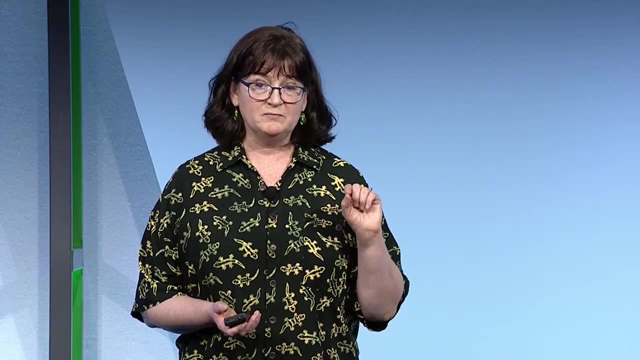 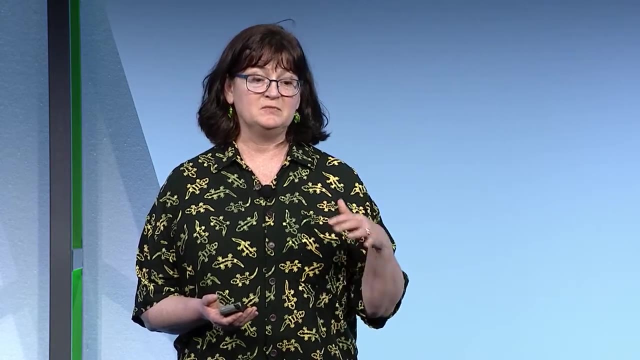 Okay, and then the other key piece, then, is using the CloudML Engine Online Prediction Service and the Learn TensorFlow model to within our pipeline. we're going to be able to use this to actually do these predictions, So you can do this with any TensorFlow model. 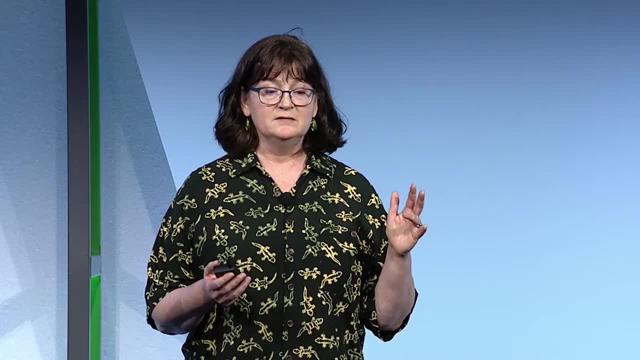 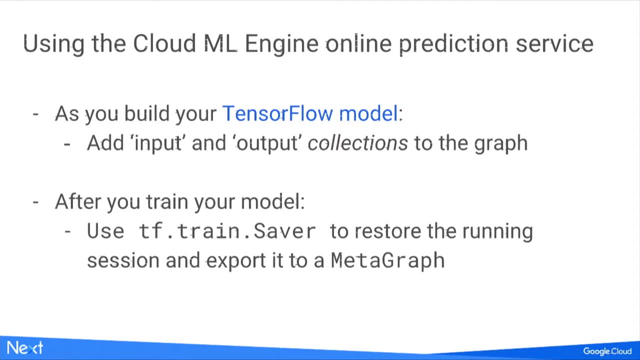 and you just need to make sure that it adheres to a certain convention when you're building it. This is spelled out in the documentation. obviously, When you're building it, you need to add certain input and output collections to the graph And you can actually do this kind of post hoc. 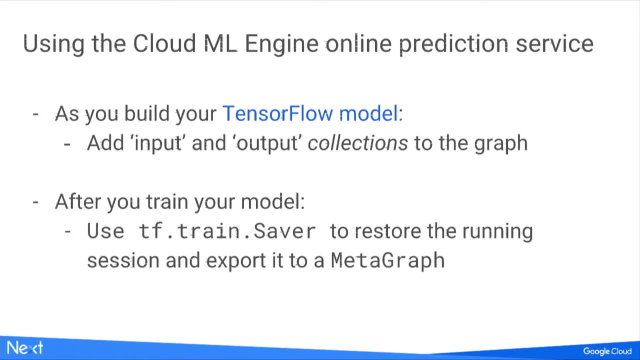 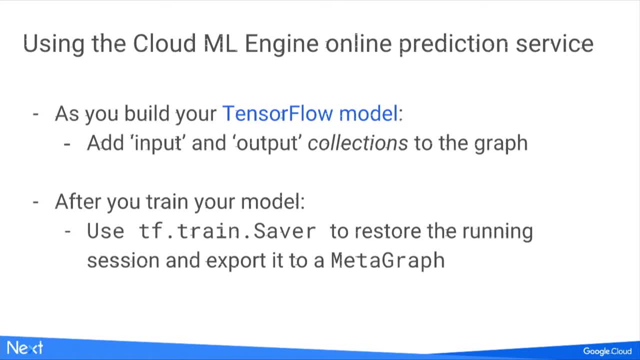 added these new nodes that were necessary for CloudML and then wrote it out again, So you don't need to do retraining again to add these nodes to your TensorFlow model graph if you've done any messing with TensorFlow. So after you train your TensorFlow model, 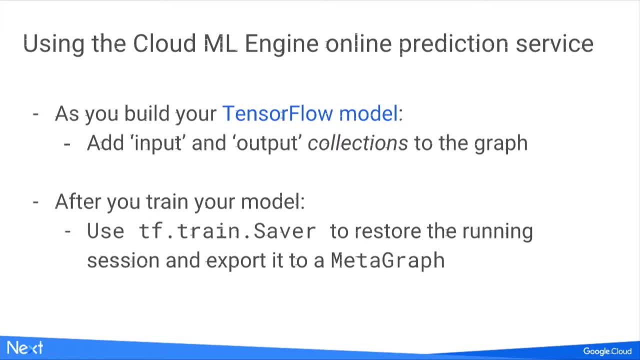 you have to save it, to save it in a certain way. basically you need to export it as a metagraph And then, once you've done those two things, then CloudML Engine knows how to deploy that model and how to use it. 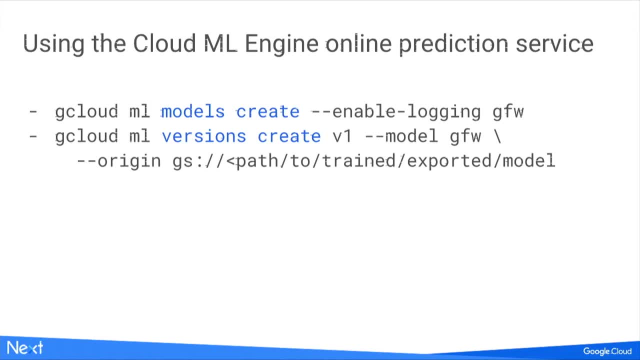 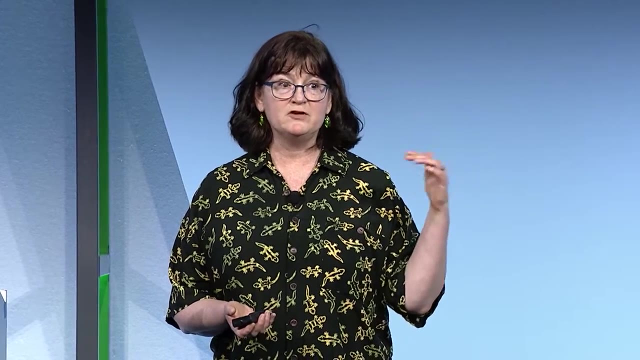 how to serve it for predictions. So that looks like this: This G Cloud- for those of you who aren't familiar- is the Cloud Platform. SDK is the Cloud Platform SDK. So this is command line: You first call, you first create your model. 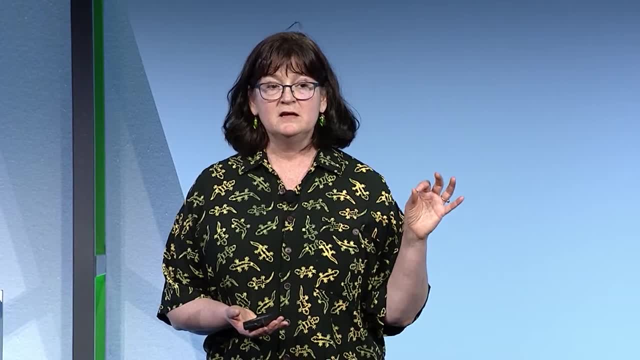 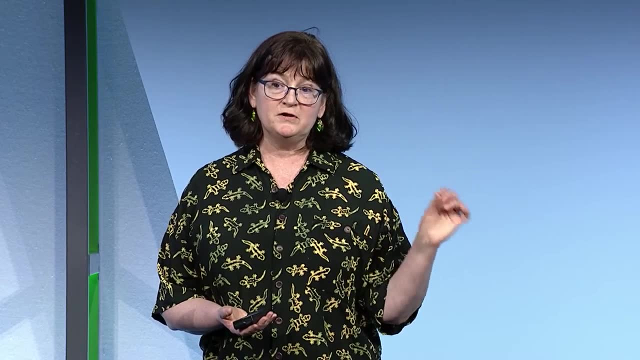 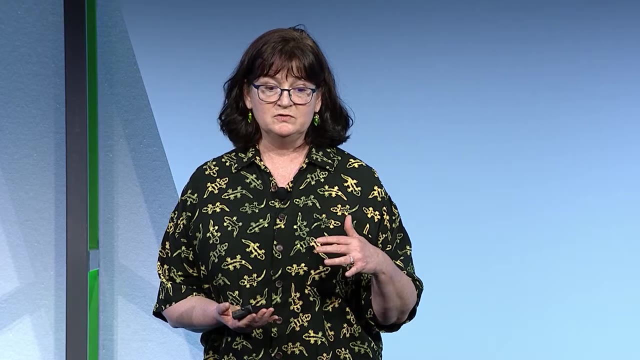 that's just kind of like a semantic tag for the model, And then you deploy a version, a named version, of that model with a pointer to the path where you saved the model once you were done training it. So you did your training. 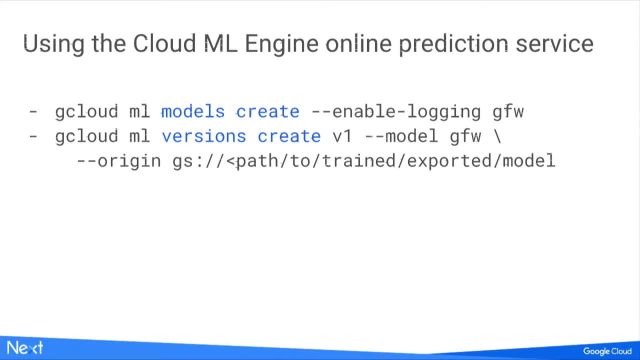 whether it was on CloudML Engine using GPUs, as David's team has been doing, or you know some other way. You've got your train exported model. Now you point to that path and this deploys your model to the cloud. 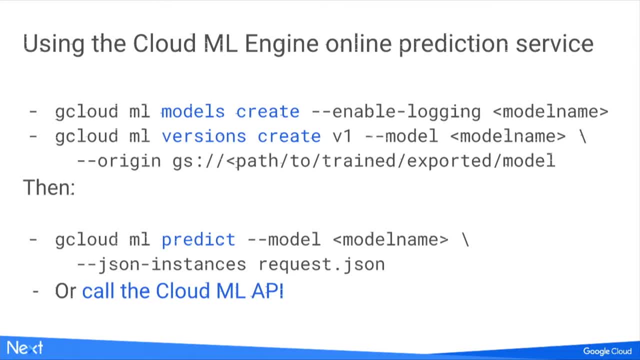 So then, once you have done that and it's successfully deployed, you can use it for prediction. So this is, you can do that in all sorts of ways and you can do it just from the command line G, Cloud, ML, predict, and it's you know. 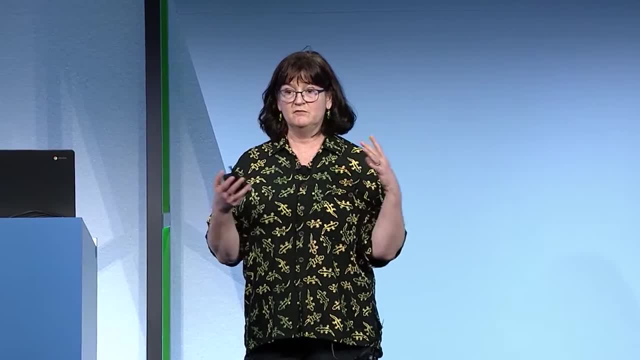 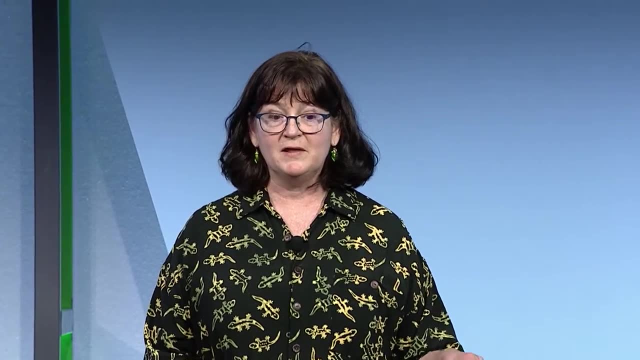 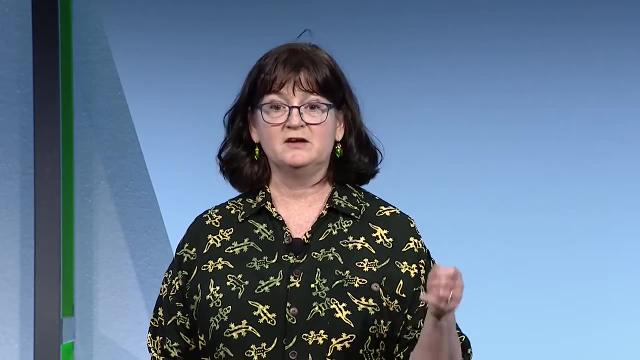 and just feed it the model input in the form of, like, say, a JSON file, Or you can do what I did in this data flow pipeline, is use the Cloud ML REST API and send it data and call it directly from the data flow pipeline. 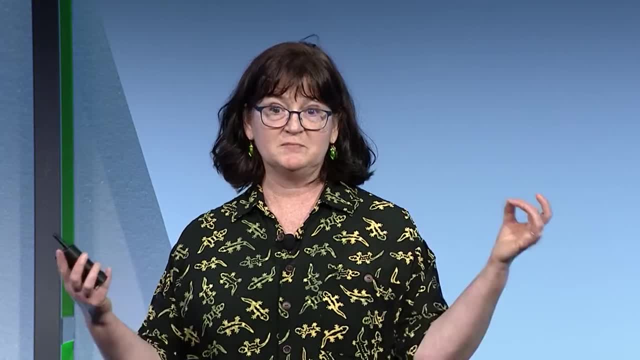 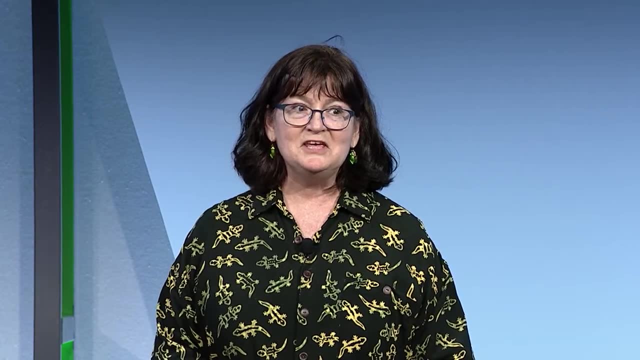 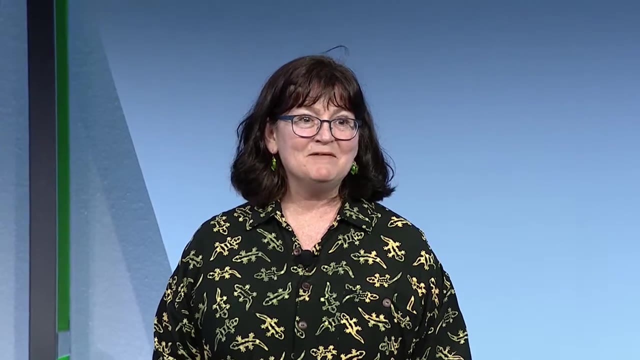 and get back the prediction and use it for subsequent processing in the pipeline. So I don't know if any of you caught the keynote this morning and the New York taxi- very cool New York taxi demo- But if you did you might have caught. 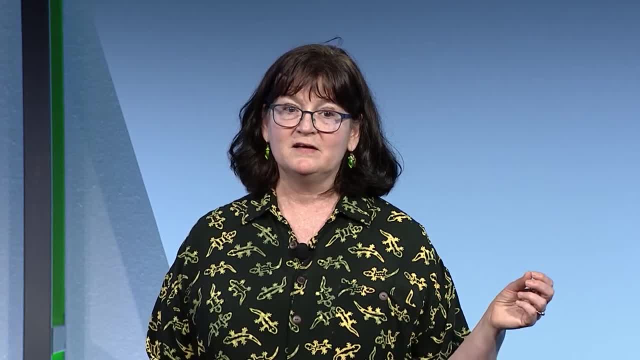 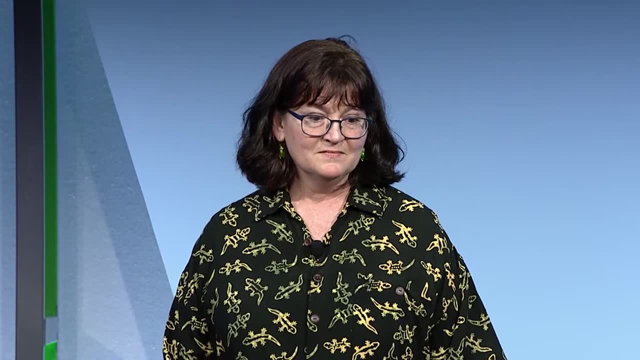 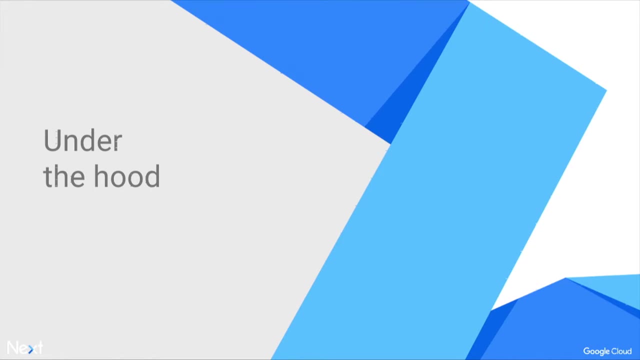 that it was using. it was doing the same thing. It was calling the Cloud ML engine online prediction service from a data flow pipeline. Okay, So just sort of one more dive a little bit further to look at like what to the 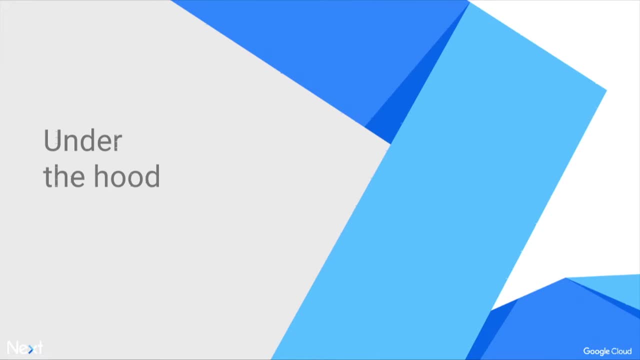 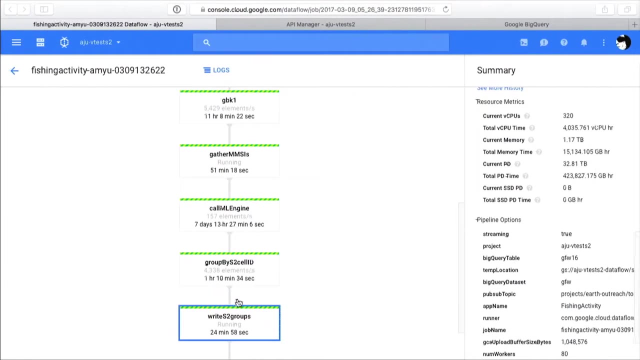 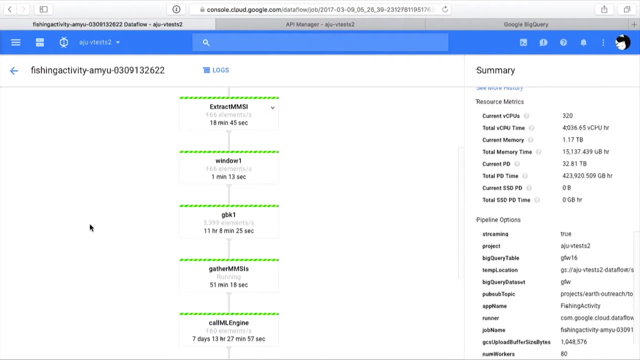 what's the UI. look for this. If you're gonna build this. you know what would you see in the Cloud console. Okay, so here is. here's that pipeline, happily running, And you can see the. the call ML engine part. 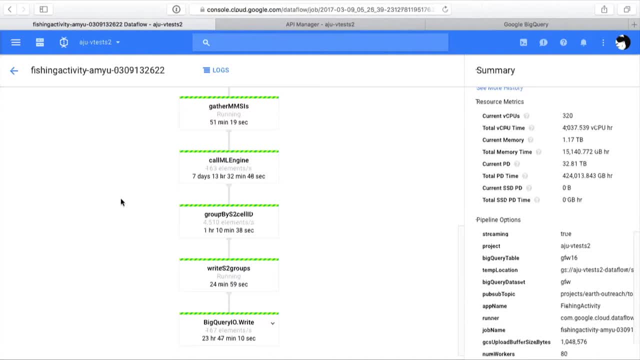 is where we're actually making. the REST API API calls out to the Cloud ML prediction service And then we're taking that information. basically, where do we think phishing activity's happening? And the rest of the pipeline is grouping it according to these S2 geometry regions. 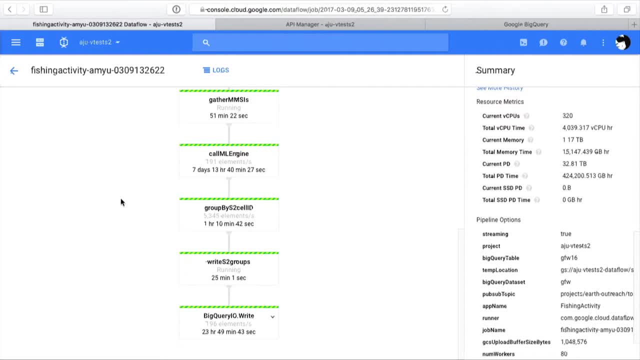 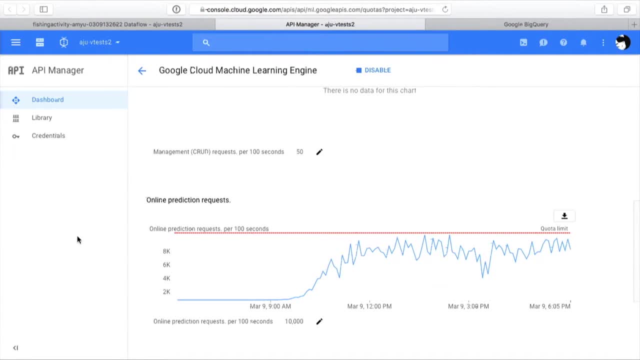 So you can see I'm kind of like cutting it close. I keep coming close to my quota, but I'm carefully backing off when I do So. this just lets you track what's going on with your deployed TensorFlow models. And then this last tab here is BigQuery. 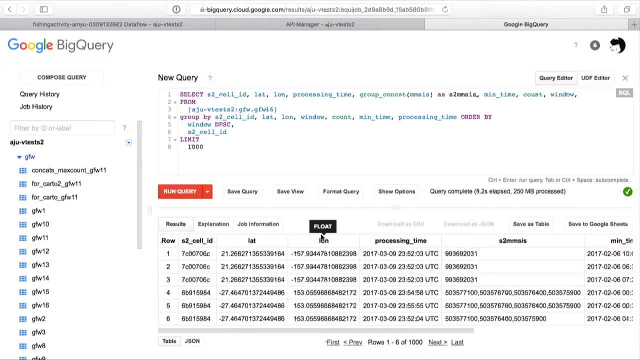 where all this derived information is getting written. BigQuery has a streaming API, and then we can use it for whatever we like, including building a map like the one I showed you. So I'm going to try to run this query just to kind of prove that it's a live demo. 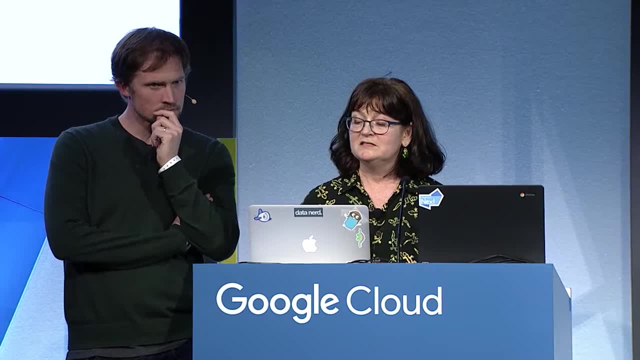 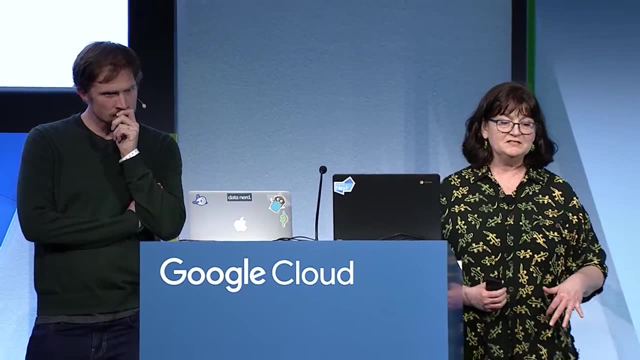 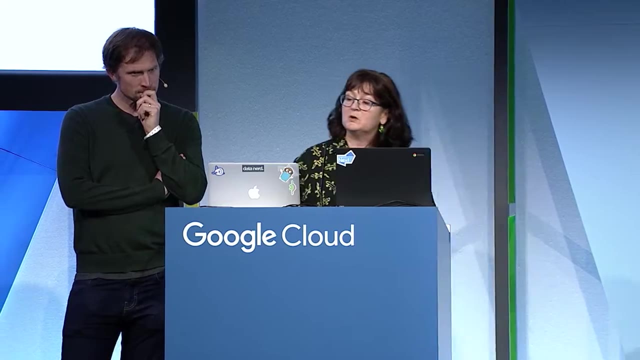 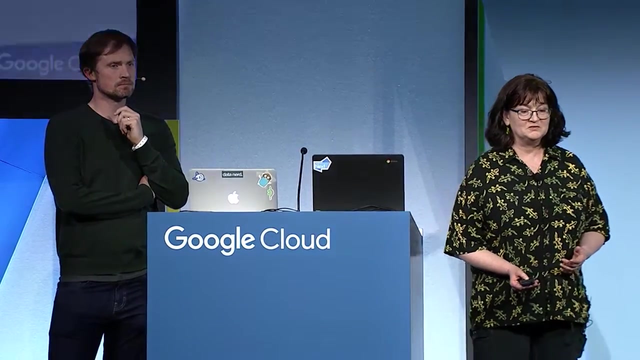 that we're watching And so the processing time is in UTC. but you can see that it's written in BERT, You can see UTC time. That's relatively close to our current time. Okay, There's my backup slides there, All right. so if we go back to that sign pattern, 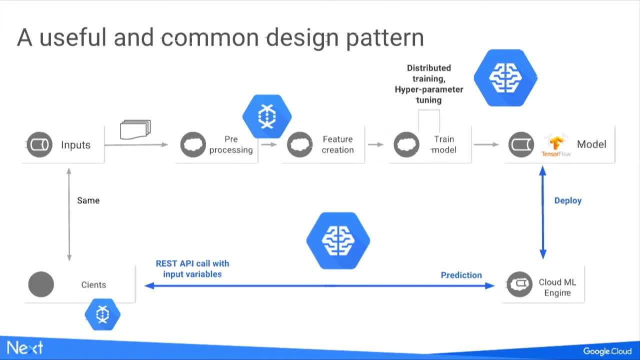 that I was showing you earlier. use Dataflow to do preprocessing, to do feature creation. shuttle that data off to Cloud ML Engine to do distributed training- really highly scalable. use GPUs. Now we can see there's another piece of this that is also very common. 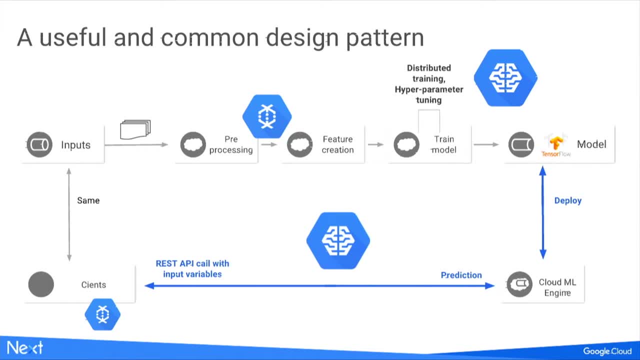 is: you've got your trained model, you want to deploy it and then you want to use it for prediction. So that's sort of the bottom part of this graph, And in the lower left that's my new Dataflow pipeline, which is using the deployed model. 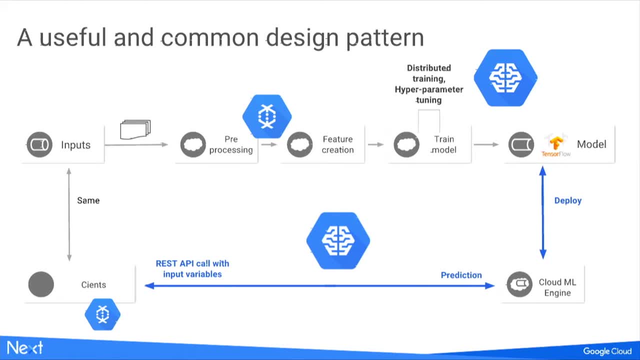 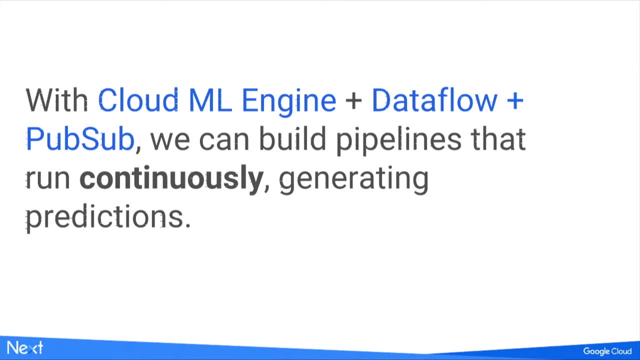 through the Cloud ML API to get those predictions. Okay, so just to kind of to summarize what I did with the new streaming pipeline, there were a few cool things that made it all fit together. So the first thing was Beam's unified batch streaming model- right. 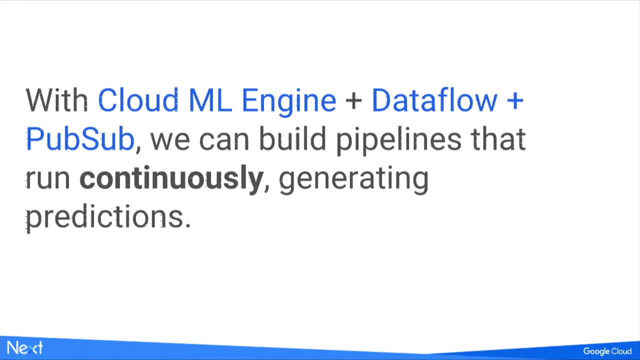 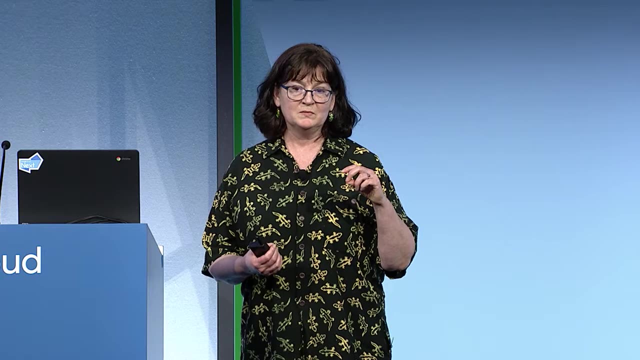 There wasn't really very much. It had to be done before I started building on top of this. So that was one thing: The ability to easily compose pipelines, kind of glue them together, using PubSub Beam's ability to support reasoning about event time. 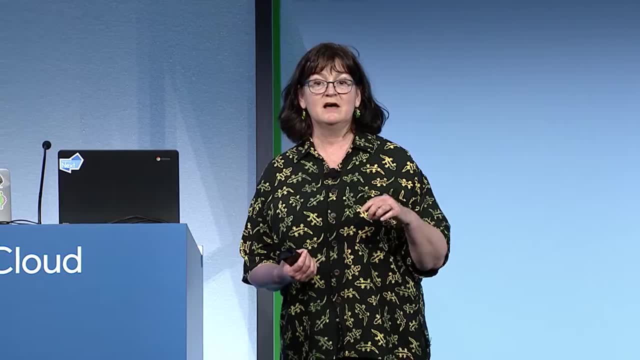 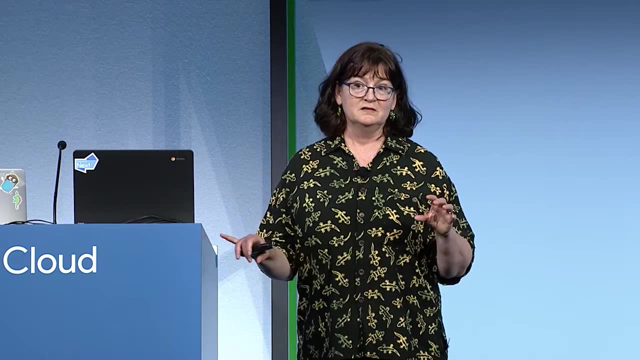 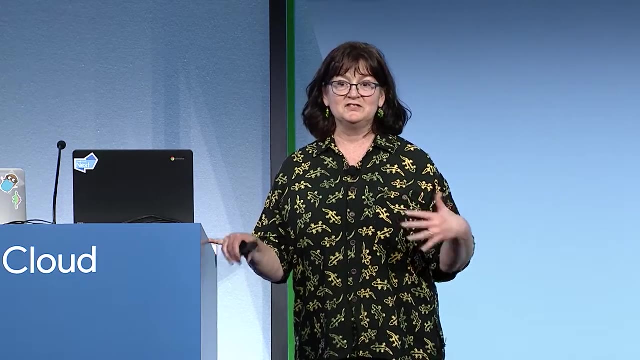 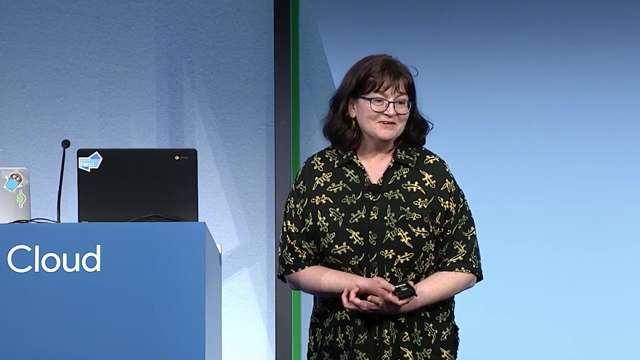 in terms of when the data was actually generated, not when it arrived. And then, of course, Cloud ML Engine Online Prediction Service to use our trained model in this new pipeline and get results and just incorporate it into the analysis. Okay, so we covered a lot of stuff. 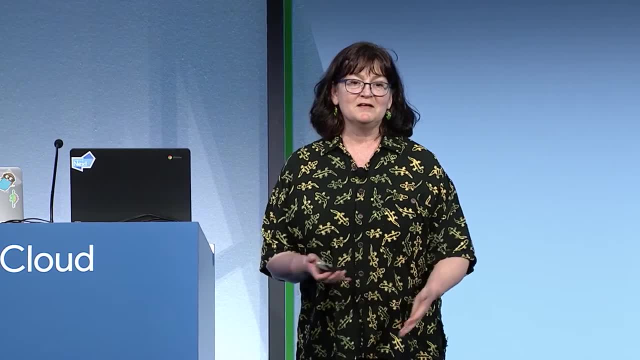 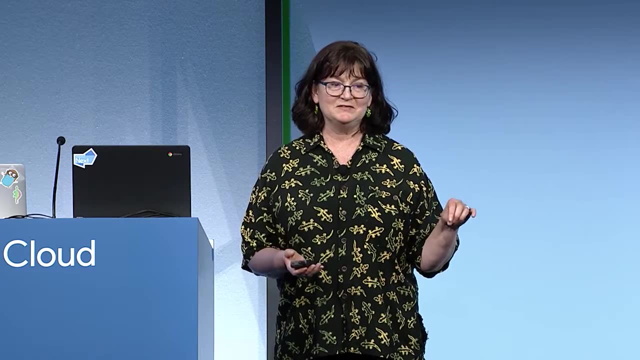 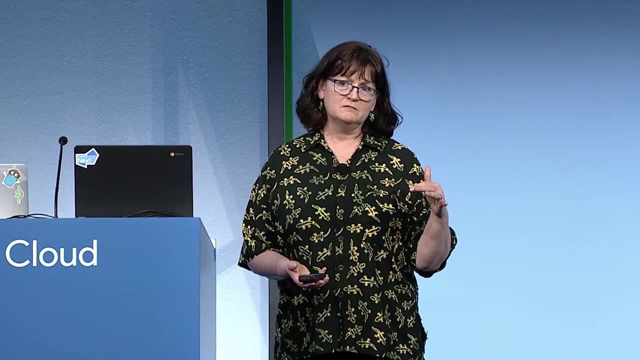 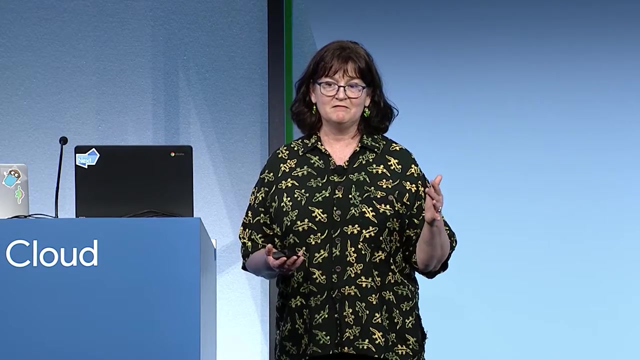 and from the cloud platform standpoint. hopefully you've gotten a sense of how you can use these products for real world problems in an interesting way, how easy it was for me to build on that and extend and add new functionality without having to do a huge amount of extra work. 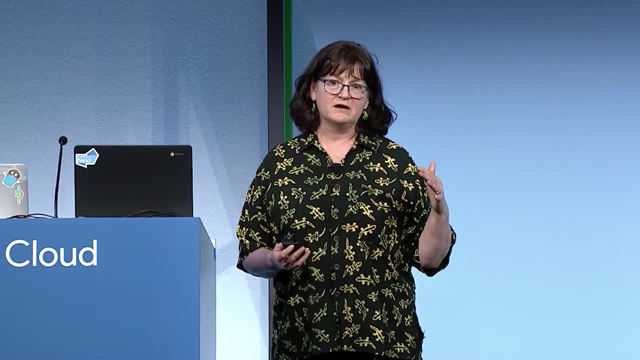 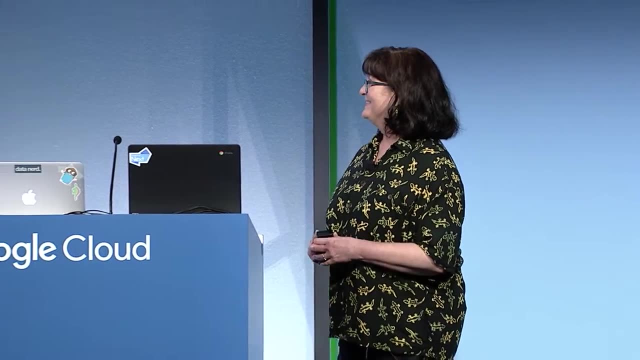 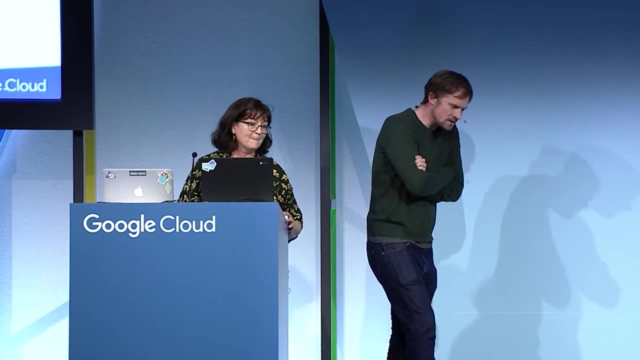 And that there are some useful design patterns that we talked about that come up again and again when you're building this kind of workflow. So I think that brings us more or less to the end of our talk, And I just want to take a step back. 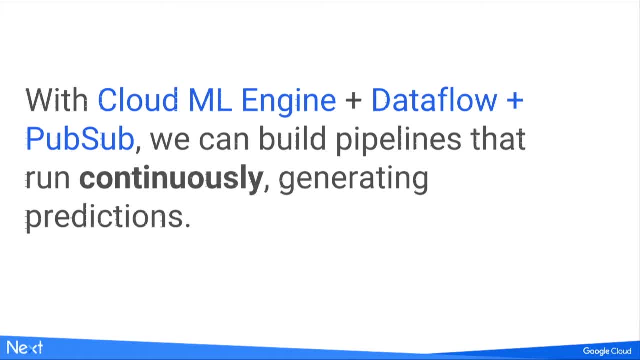 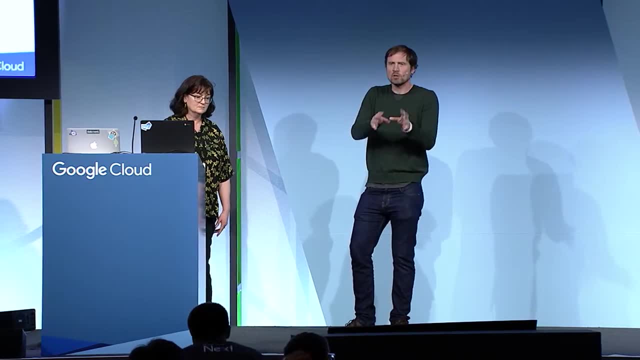 and say why I think this is really exciting, And as someone who's kind of interested in working on big data problems to address the global environment, what's really cool about this is we couldn't do this five years ago because we didn't have the satellites. 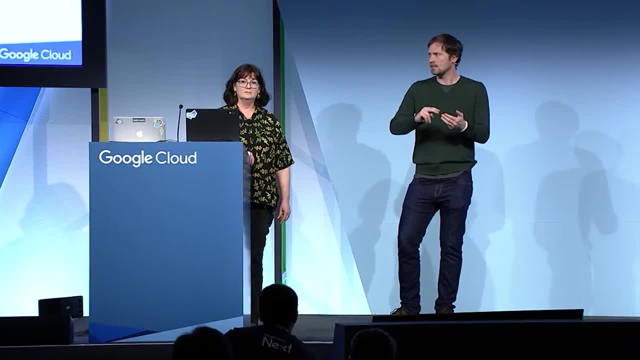 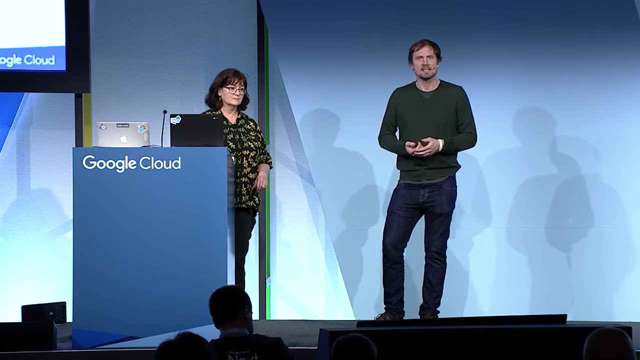 we didn't even have the data set, And even if we didn't, we didn't have this technology to process it, to be able to do. these machine learning techniques didn't exist, And so we're really able to make a huge leap forward now. 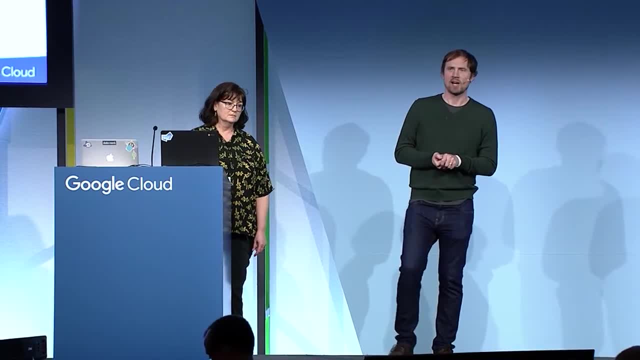 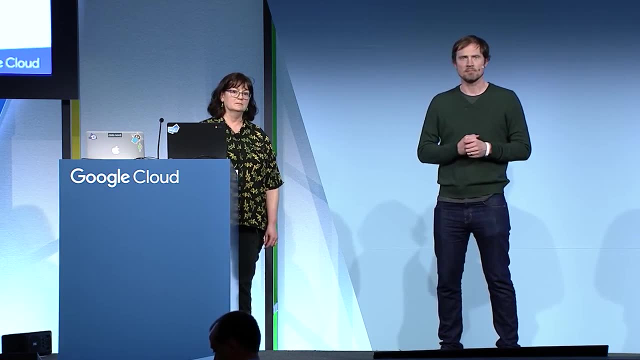 compared to just a few years ago, And that's one of the reasons why I got up and really excited to work on this data set every day, And I think it's going to make a real big difference in terms of how we manage some of these. 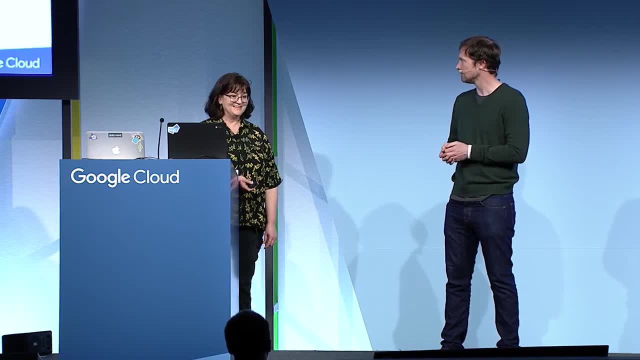 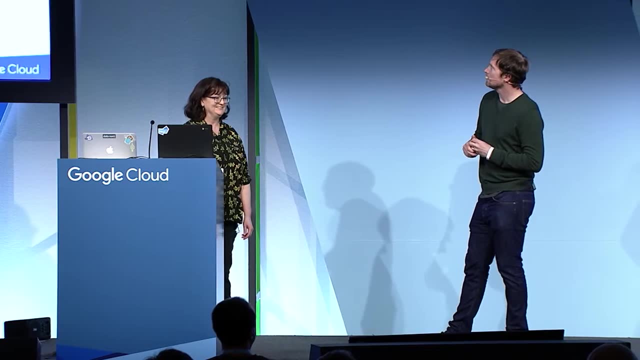 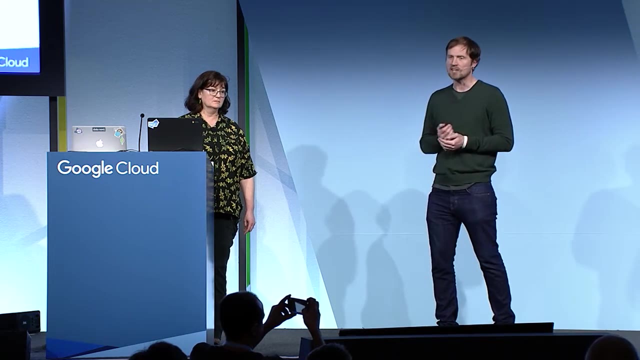 globally shared resources. Okay, so what's next? basically, First exciting news from Global Fishing Watch. I will let David, Yes. so first we have a data website, globalfishingwatchio, companion to the org site, where you can download all of this data. 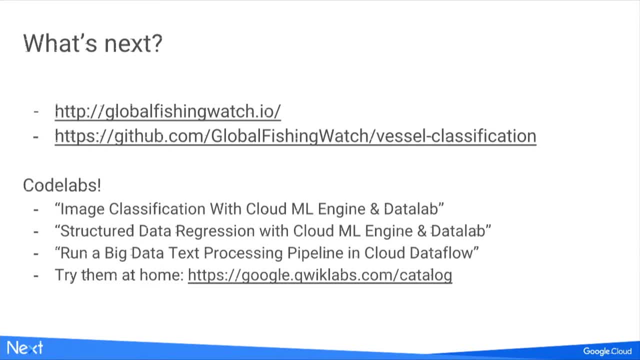 You can download all of our data and code that we are able to post there. The main data set of AIS is proprietary. We have to buy it so we can't just share it with anyone But the other but our code and a lot of the derived data. 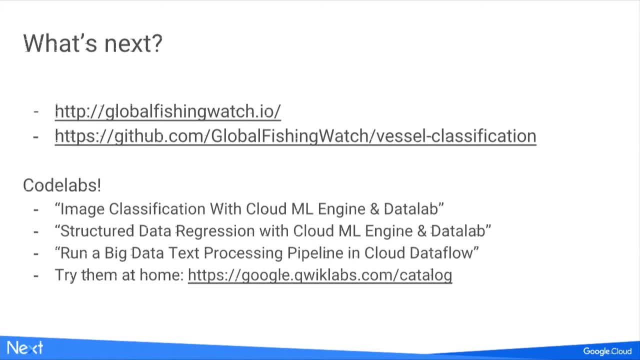 we can share and so we're making it public there. And also just today we have made the repo with this whole vessel classification and fishing identification. all this machine learning stuff we've been talking about is all in that repo So you can go and do this yourself.